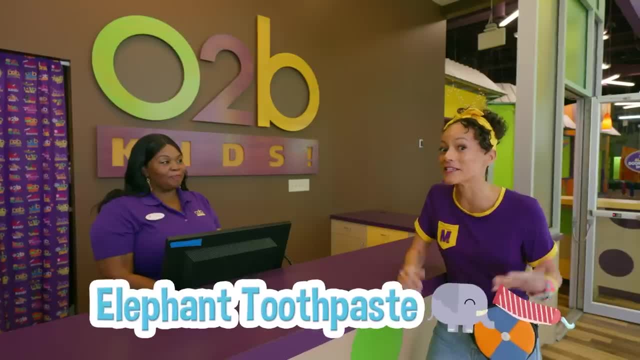 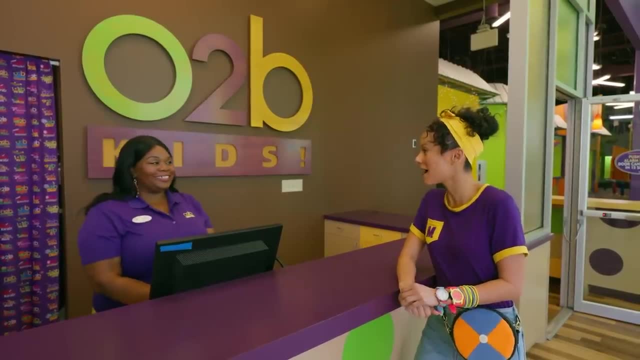 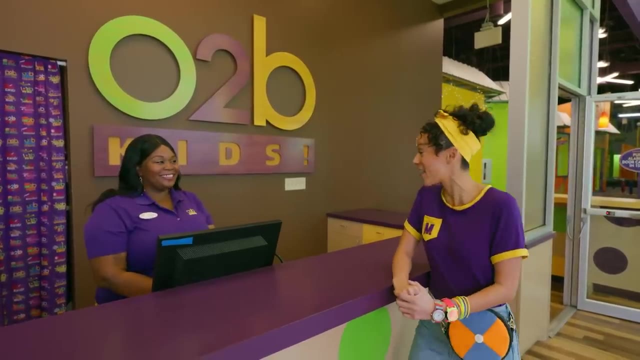 could do a science experiment here and make elephant toothpaste. We love elephant toothpaste and we've actually put together a scavenger hunt for you. What That sounds so fun. Will you go on a scavenger hunt with me? Cool. So how do I start? You're all checked in and ready to go. Oh, okay, Let's go. 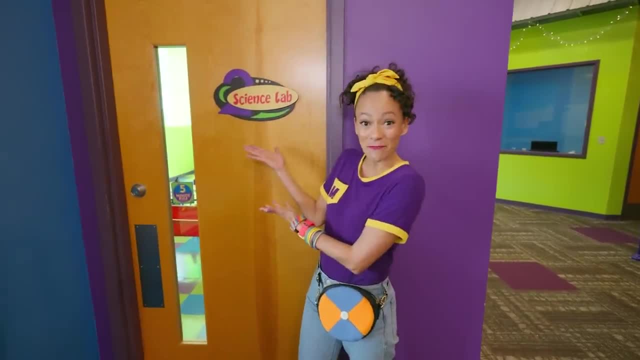 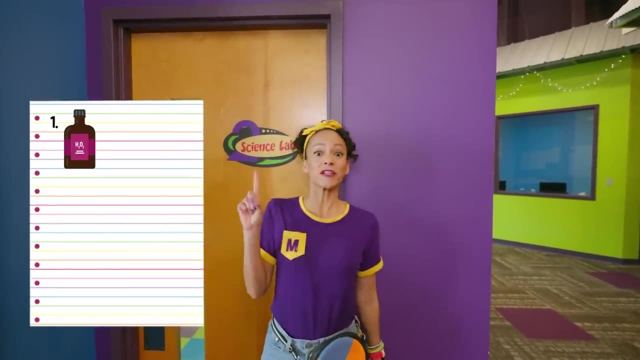 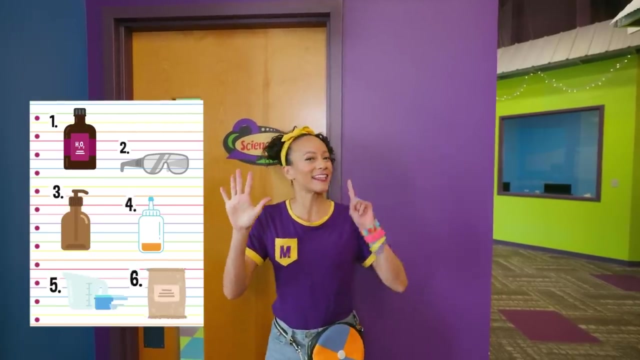 Check it out. We're at the science lab For this science experiment. we need to find six items in our scavenger hunt. We need to find hydrogen peroxide, safety goggles, dish soap, food coloring, measuring cups and yeast. Okay, 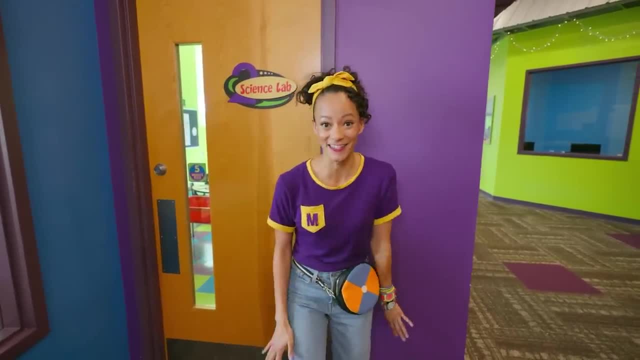 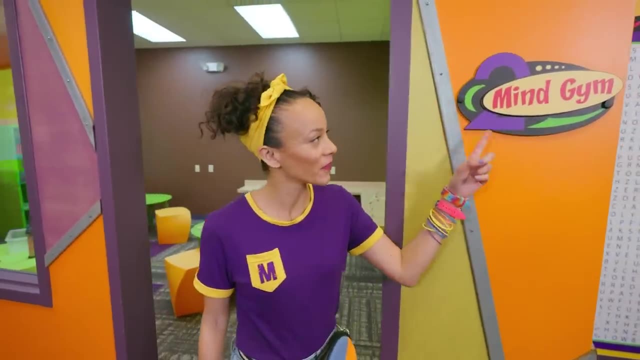 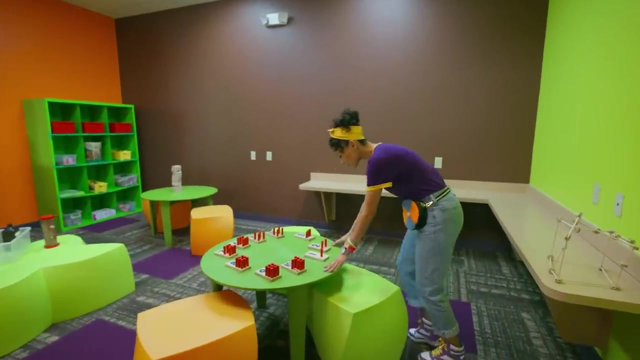 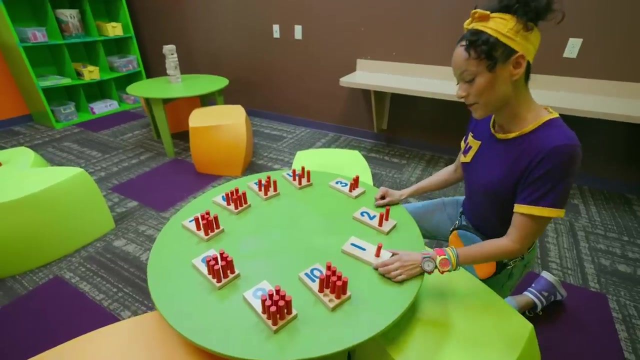 Can you help me look for these items? Great, Let's go. Whoa, Mind gym. Whoa, This must be a room for your mind. Wow, This is so cool. I recognize some numbers here. Can you count with me? Okay, We have one. 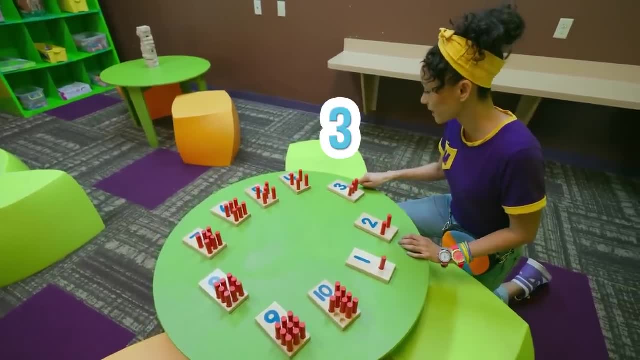 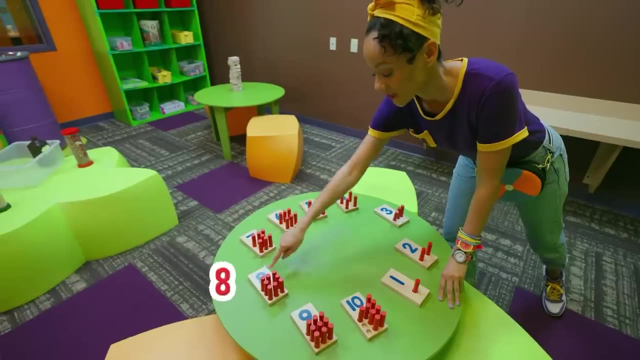 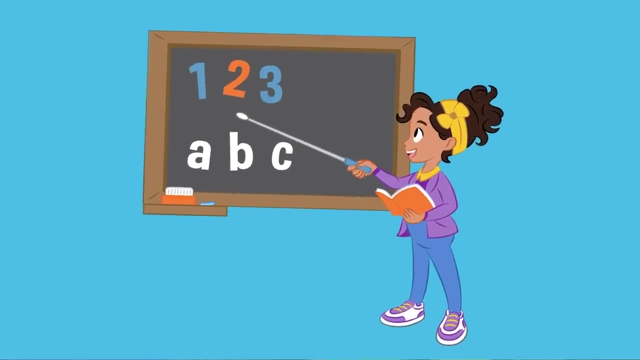 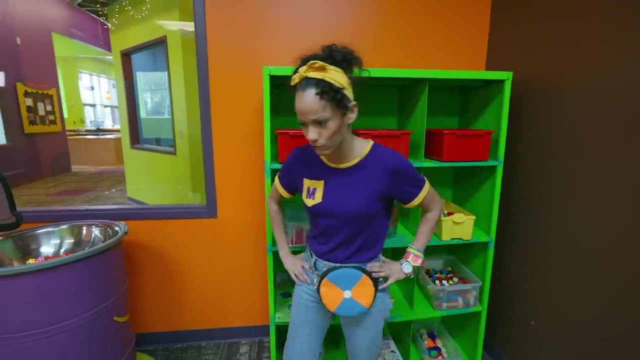 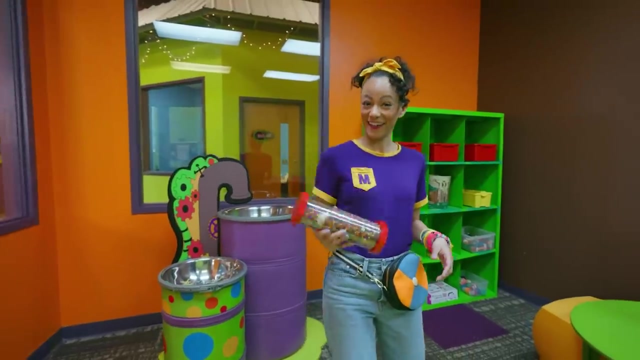 two, three, four, five, six, seven, eight, nine, ten. Wow, That's so fun. Okay, I don't see any items yet for our science experiment. Hmm, Oh, what's this? Oh, It's kinda like a musical instrument, like some kind of musical instrument, I don't know. I'd like to check out this picture. 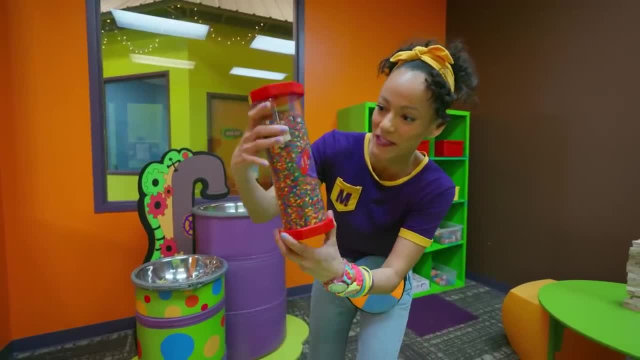 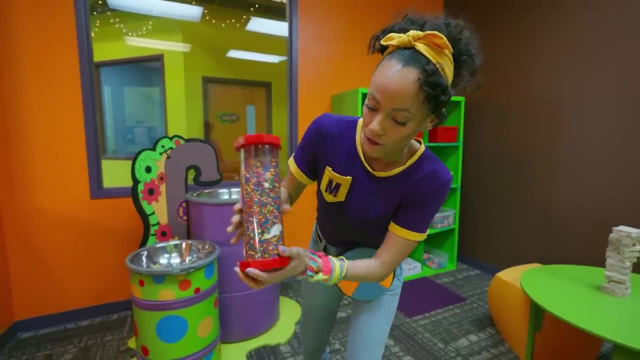 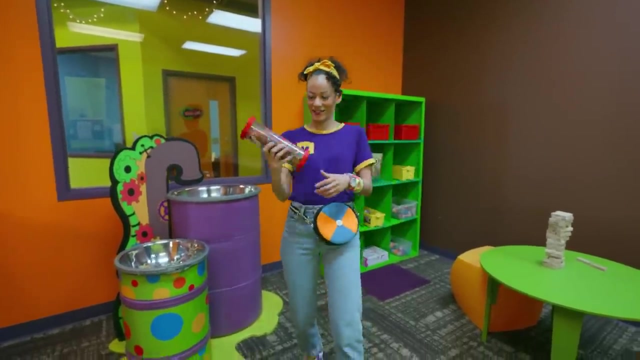 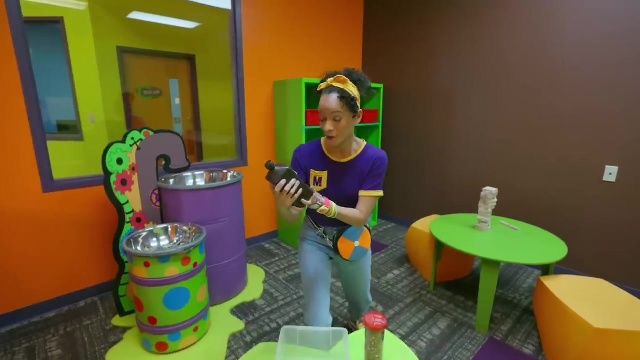 a musical instrument. See all these different colors. Oh look, there's little items in here that you can find. Looks like a balloon and a little fuzzy ball. This is fun, Cool. Hydrogen peroxide. We found our first item for our science experiment. Hydrogen peroxide can help. 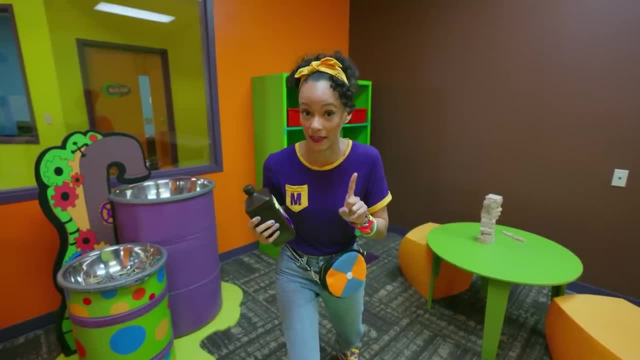 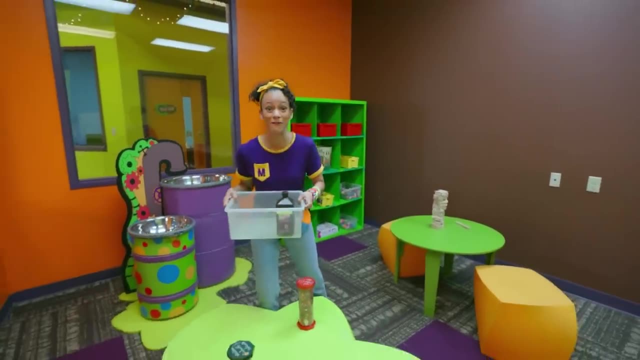 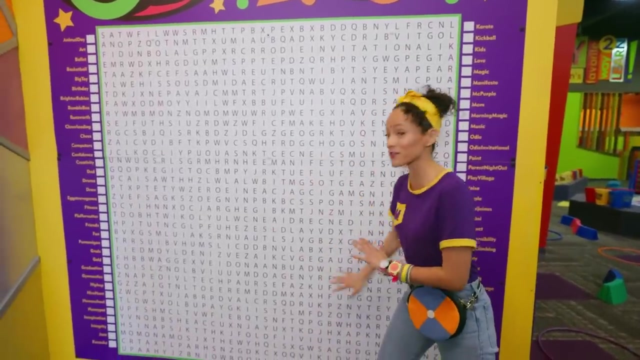 heal a cut, but you do not want to get this in your eyes, So we need to find safety goggles. Okay, good job, We have our first item. Check it out, A word find. So this big puzzle has a bunch of words in it, but they throw other letters in it to mix it all up, So it's kind of hard to see. 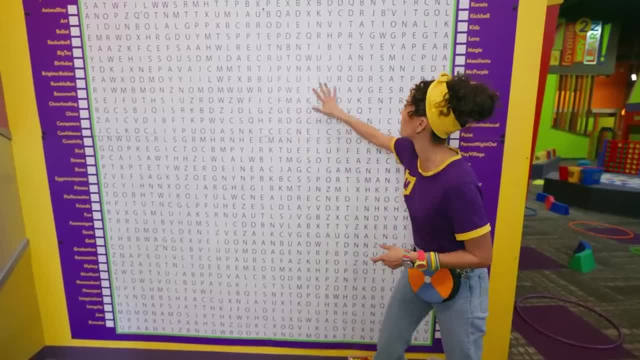 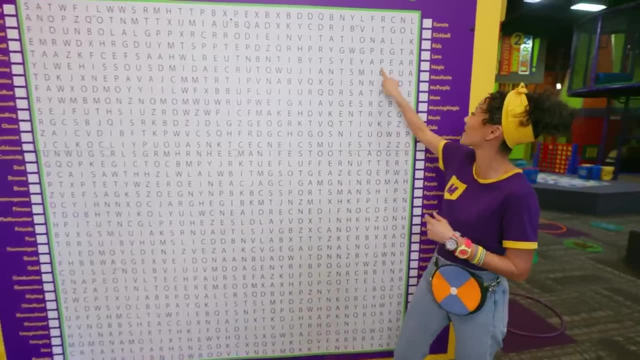 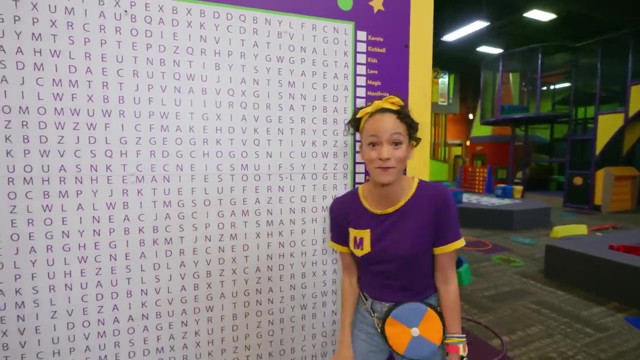 the words. See if you can find any words in here. You have to look really, really close. Oh, I found one. Look P-E-A-R. Pear- Ooh, that's a really yummy fruit. Any other words that can maybe give us a clue to the things that we're looking for? 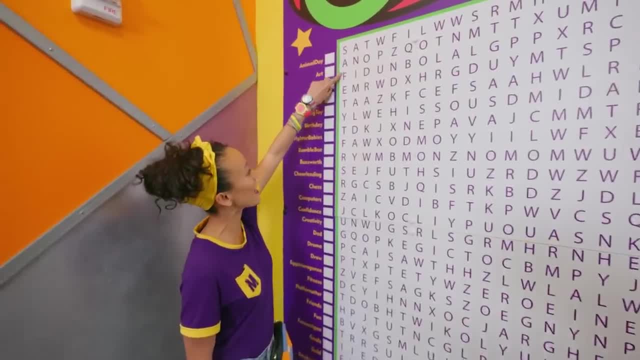 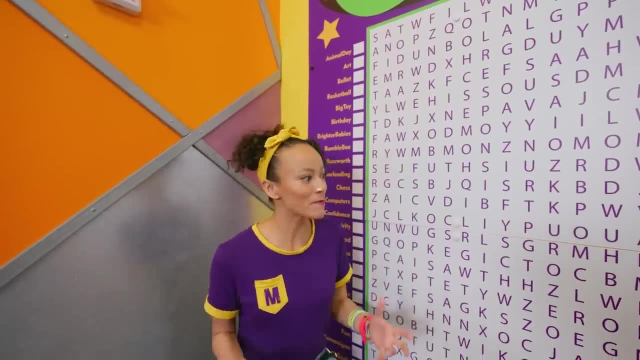 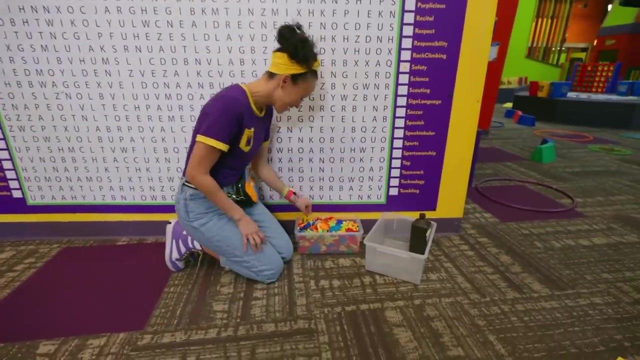 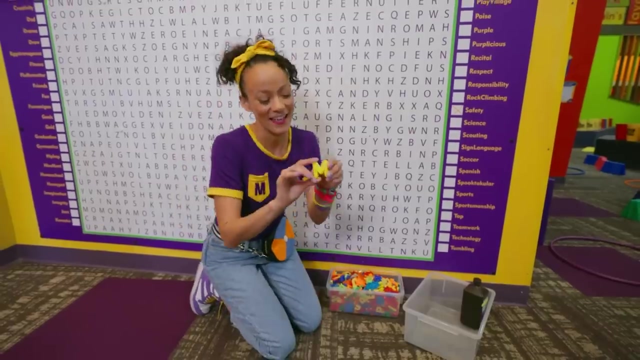 Oh, what about this word Safety? Safety Like safety goggles. Maybe there are safety goggles down here. Oh, look, there's some letters down here. Do you know what letter this is? It's the letter M for Mika, And it's one of my favorite colors, The color yellow. 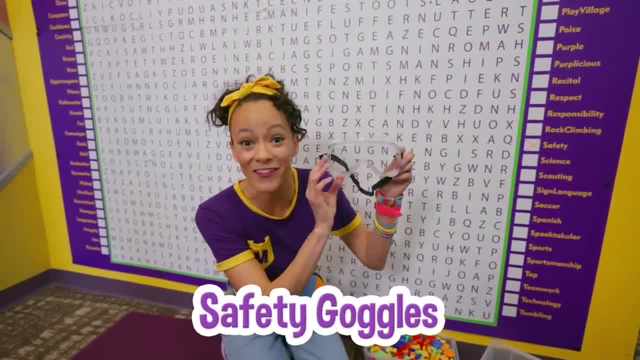 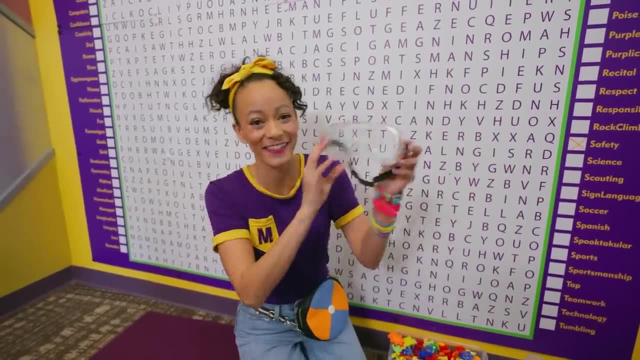 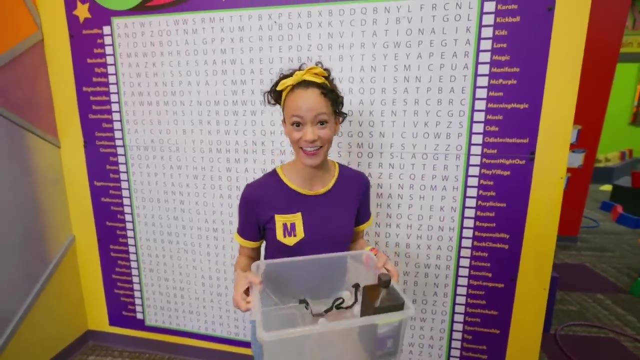 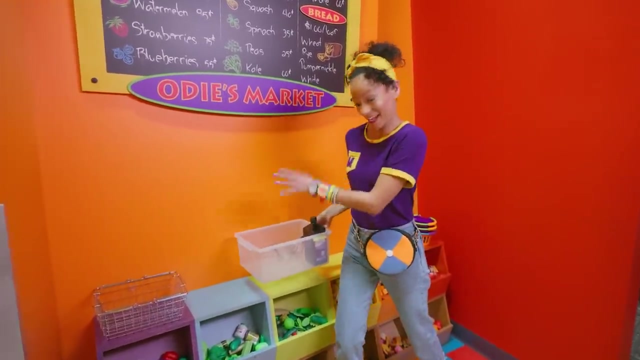 We did it. We found safety goggles. Safety goggles are really important when you do experiments because they protect your eyeballs. All right, two items down, four to go: Safety goggles and hydrogen peroxide. All right, let's keep looking. Oh wow, It's like a grocery store or a market in. 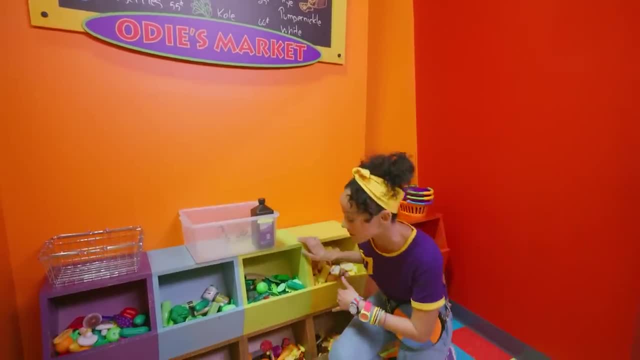 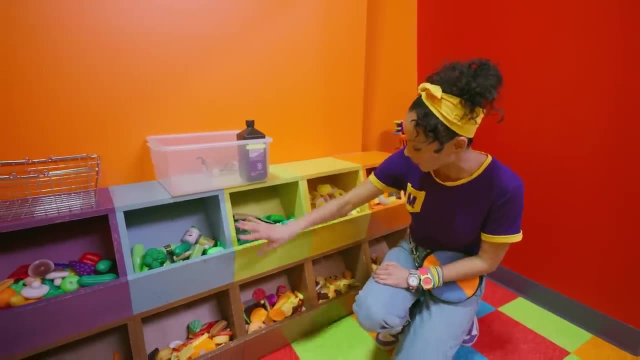 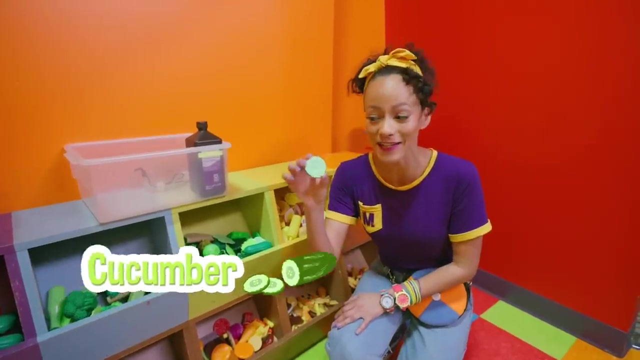 here. Look at all of this play food. Oh cool, It looks like it's organized by color. I see green and orange and yellow. Hello, Ooh, what is in here? A cucumber slice. I love cucumbers. 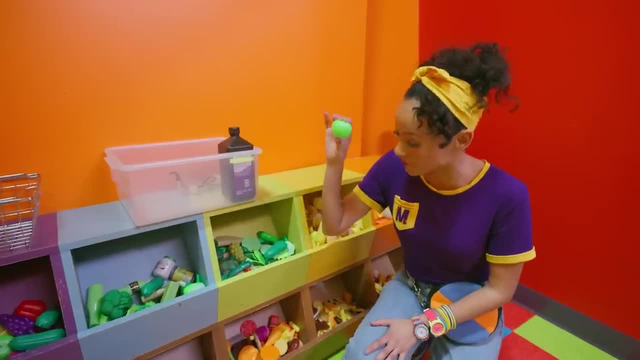 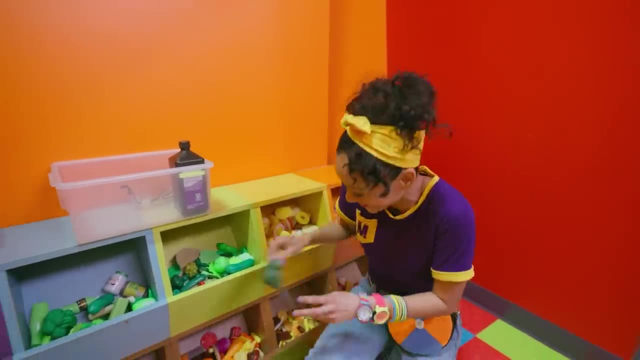 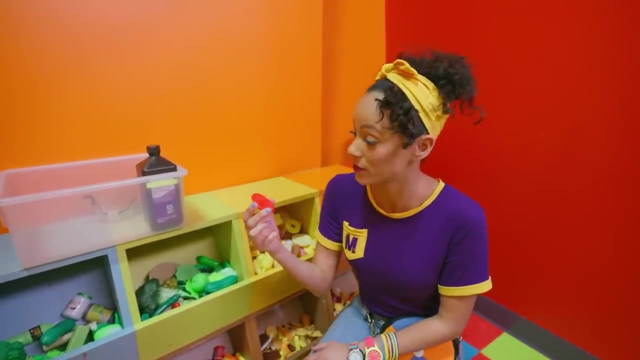 And a green apple. That's a nice healthy fruit And one of my favorite vegetables- broccoli, Ooh and a tomato slice. These are all really healthy foods. Yeah, fruit and vegetables. They have nutrients and vitamins in there. 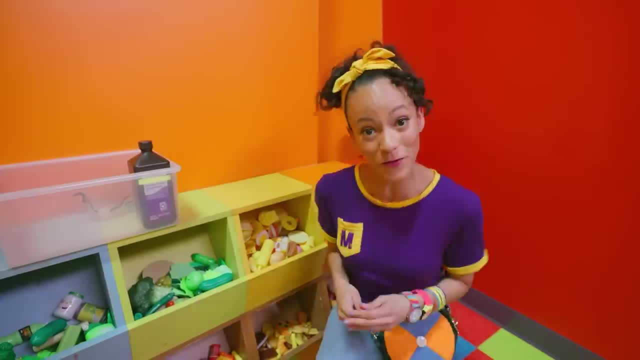 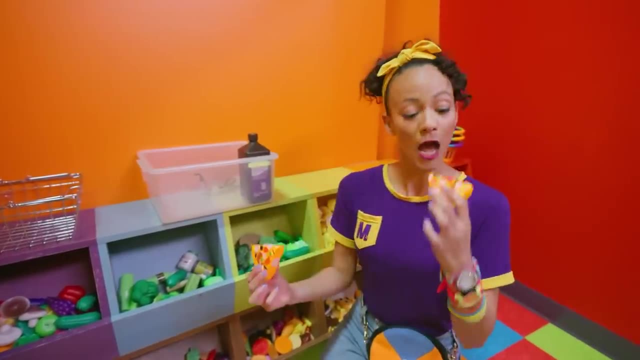 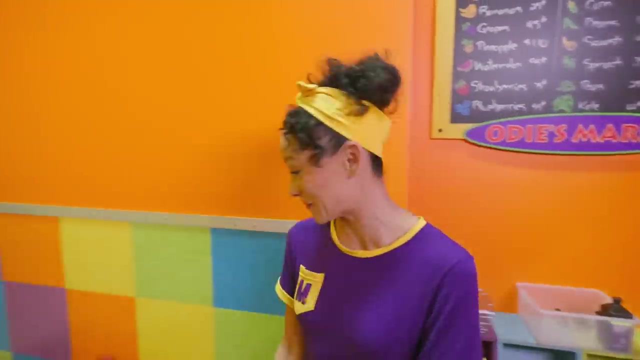 So they're what I like to call an all-the-time food. They help you grow. Ooh, what's this? Some pizza, Mm? Hey, let's see if we can find anything that we need for our science experiment. Whoa, this is like a little restaurant or a diner. 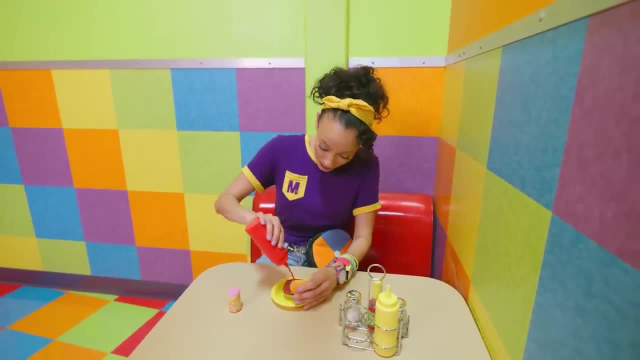 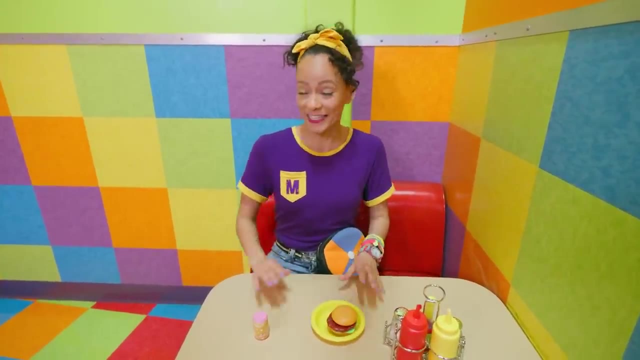 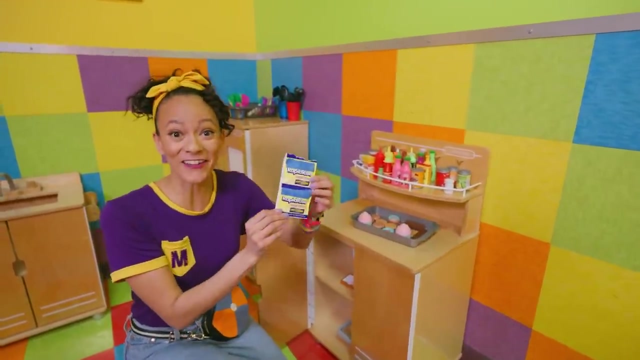 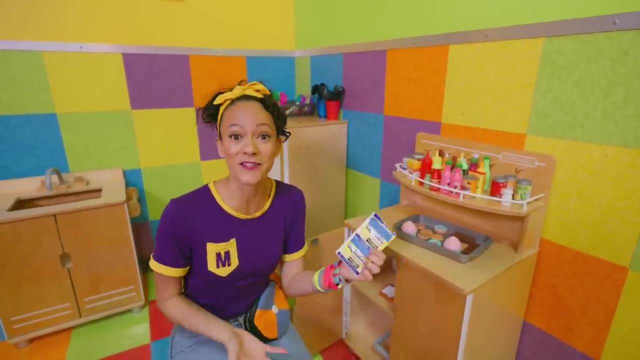 Ooh, don't mind if I do Put a little ketchup on here, Mm, Pretty tasty. See if there's anything in here. I found yeast. We need yeast in our science experiment. If you add warm water to yeast, it helps things rise. 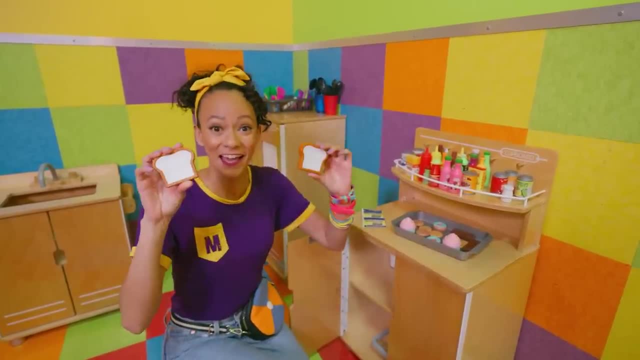 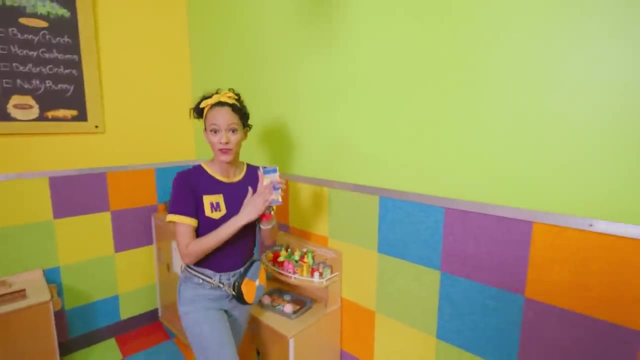 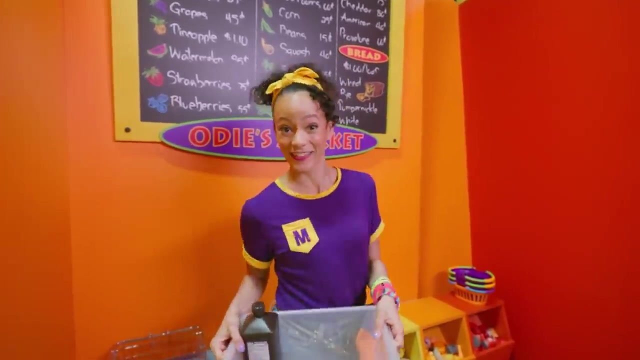 In fact, you need yeast to make bread. That's right. Hey, We're doing a great job on the scavenger hunt. Let's put this with our other things, and then we can keep looking for more items for our experiment. Good job. 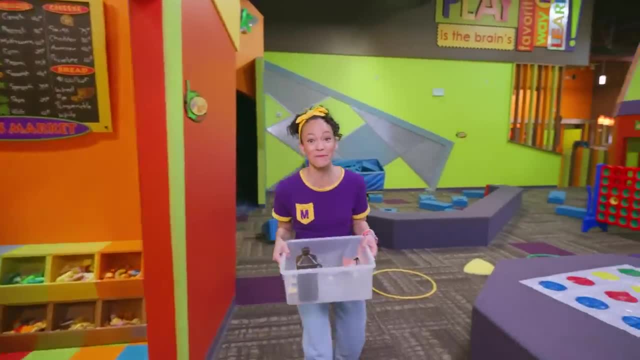 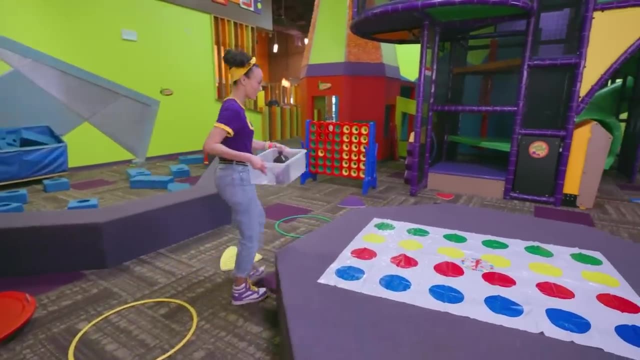 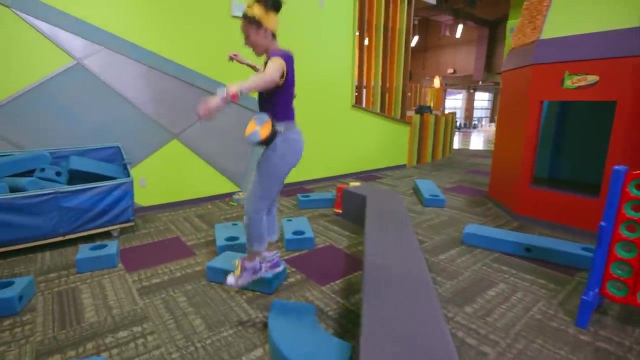 Let's keep looking. Okay, let's keep looking for more items for our science experiment. Whoa, There's a lot of fun things in here. Come over here. Whoa, look at these big blocks. Huh, Let's see. 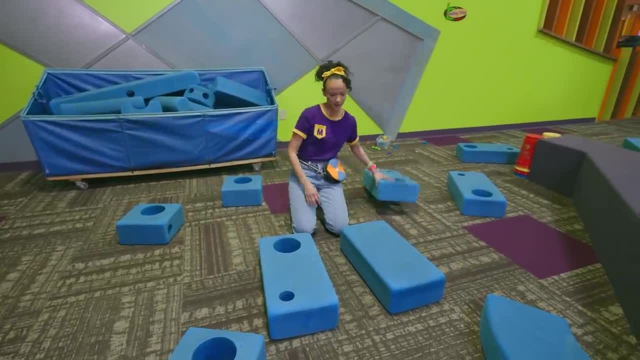 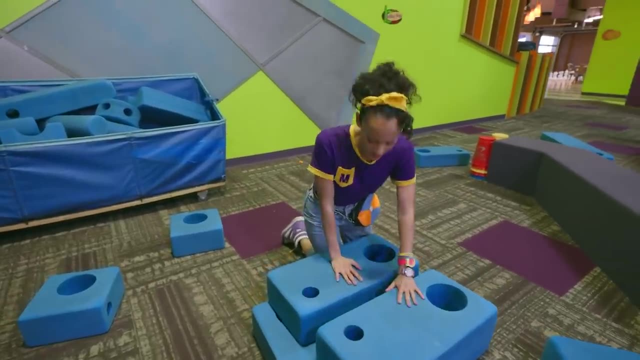 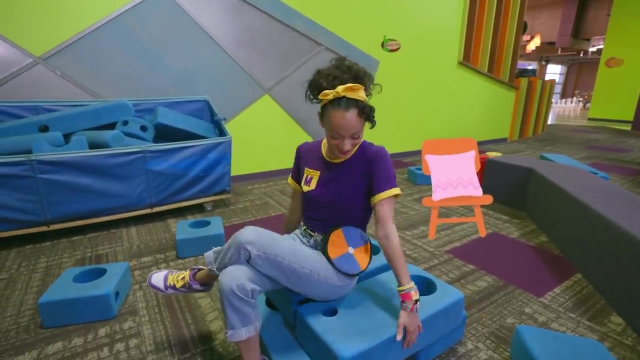 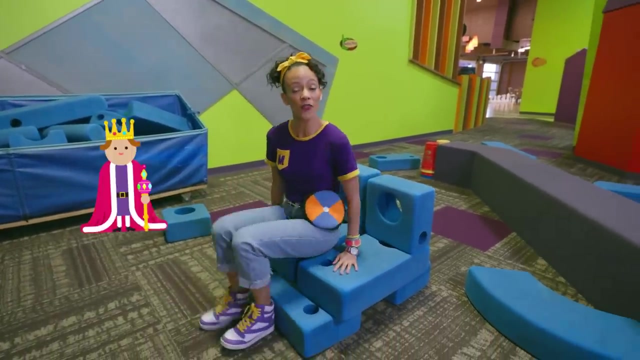 What can I make here? Okay, Hmm, Huh, Feels pretty sturdy. It could be a new chair. We can put this on it, We can put this on it, We can put this on it And this Or it could be a throne. 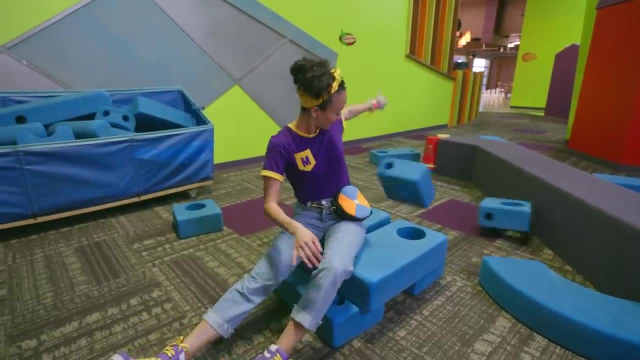 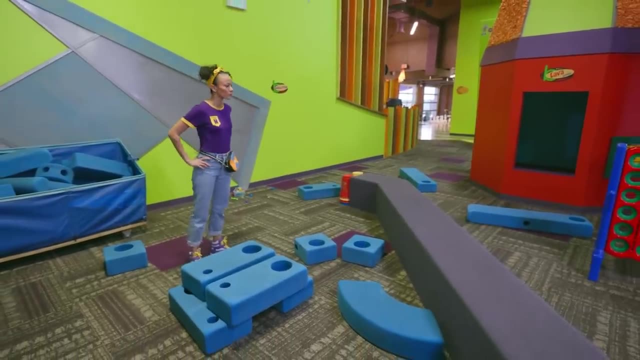 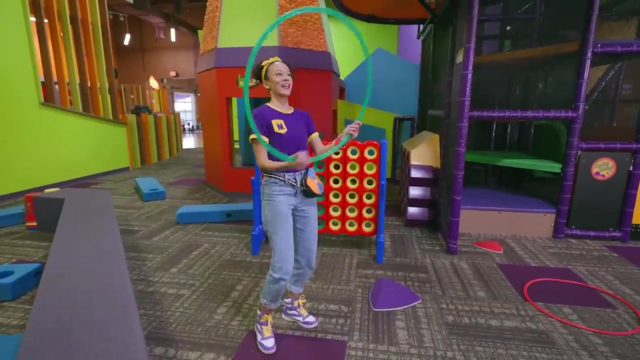 Queen Hamika. Oh, I still don't see anything for our science experiment. Hmm, Maybe there's something over here. Hey, a hula hoop. Check it out. Do you know what shape this is? That's right, It's a circle. 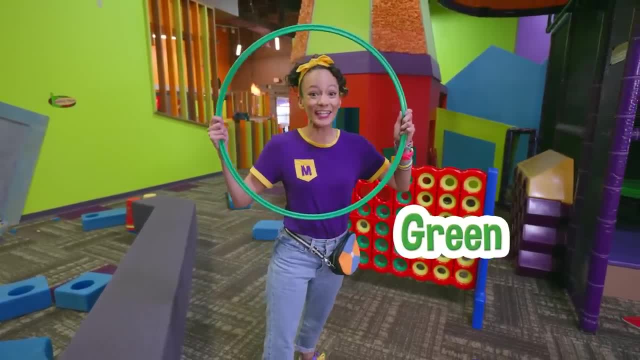 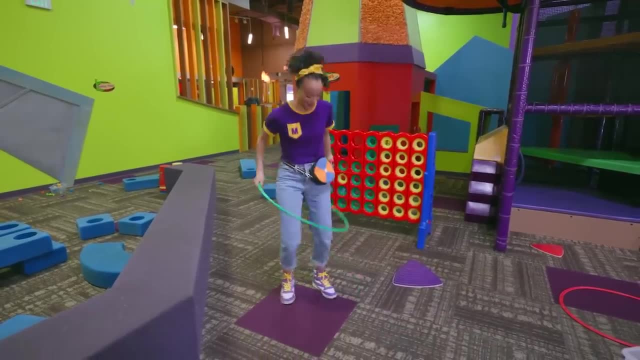 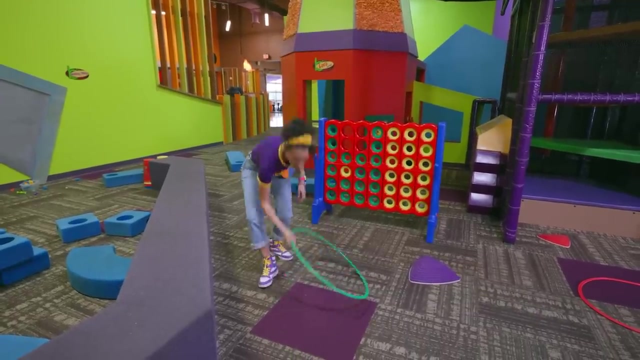 And it's the color green. Let's see if I can. hula hoop. Let me try again. Ready set, hula hoop, hula hoop. Oh, that's a little better. Look, you can also put it on your arm. 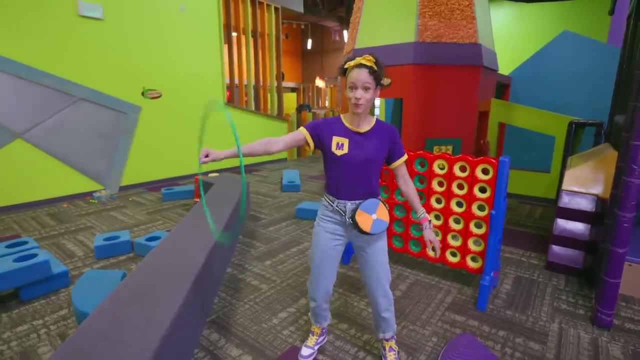 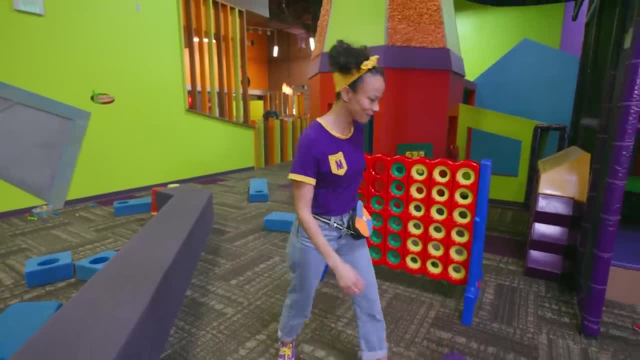 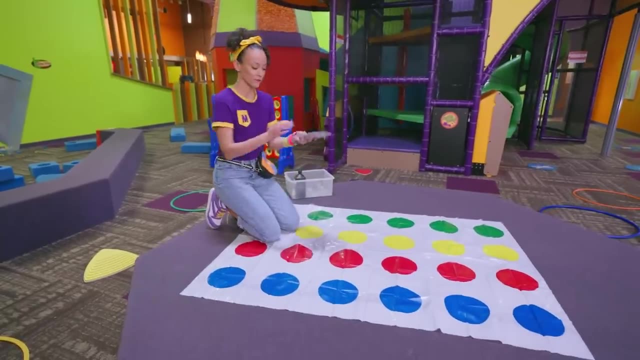 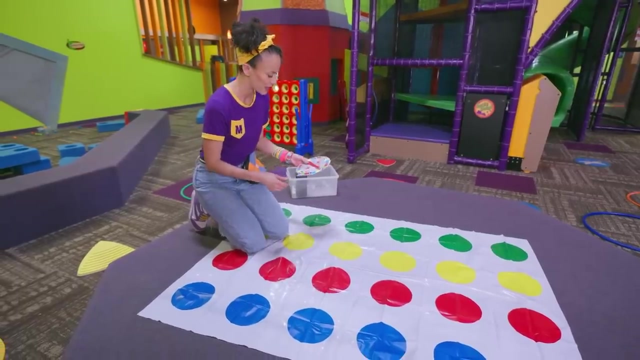 This is not something that we need for our science experiment Fun though, Hmm. Oh, this is a really cool game. Look, you have a spinner and it tells you where to put your body on the dots. Left foot yellow See. 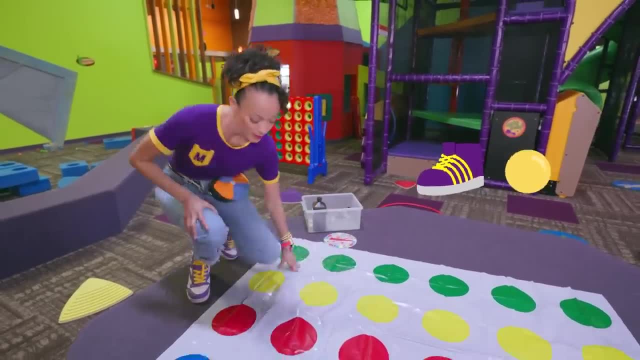 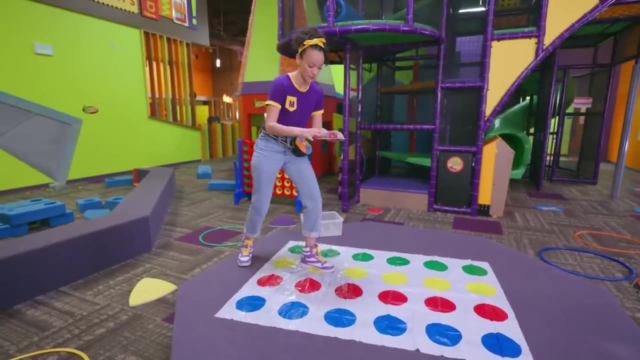 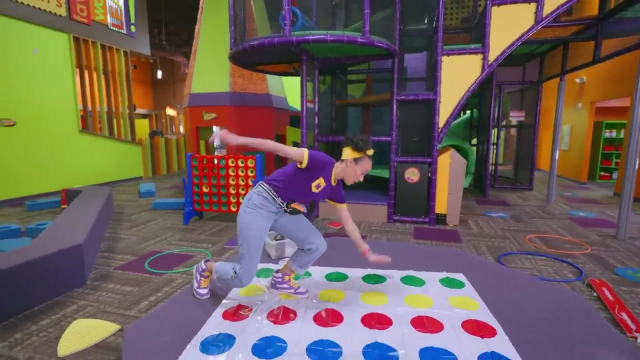 Left foot yellow. Left foot yellow. Let's see if I can do one more turn on here. Oops, Oops. This is left hand green. This is left hand green. Whoa, You have to try not to fall down, Whoa. 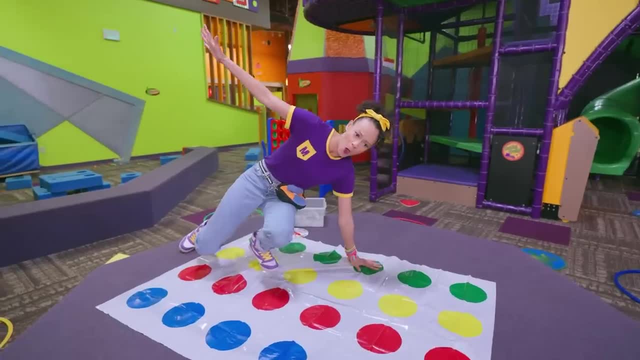 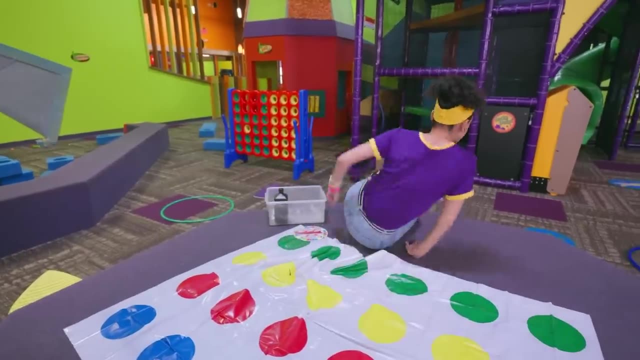 You have to try not to fall down. My mind fall down soon. Oh, that's okay. All right, Come over here. Whoa, Do you know what this is? It's a box. It's a box. It's a box. 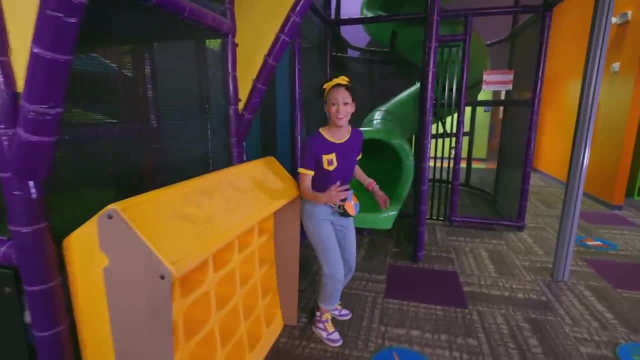 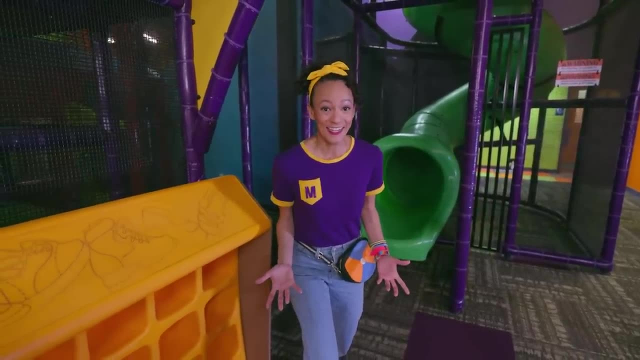 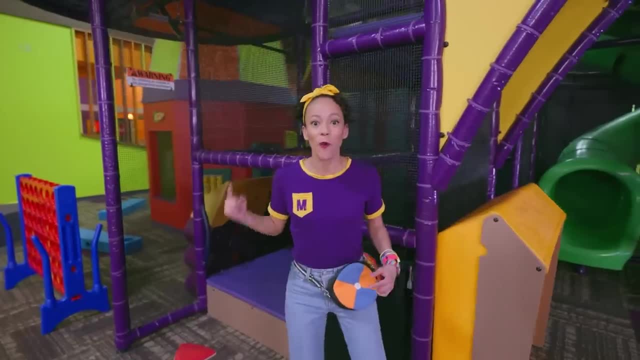 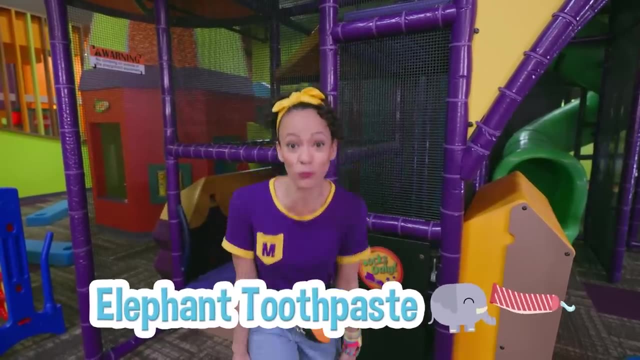 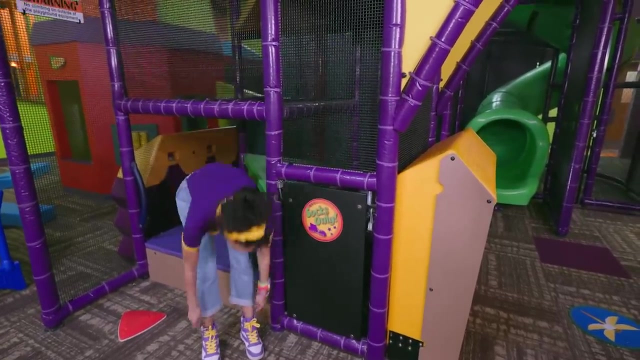 It looks like it's really high up. I wonder if there's anything at the top that we can use for our science experiment. I can't wait to make elephant toothpaste. Pfft, It says socks only. That means I need to take my shoes off. 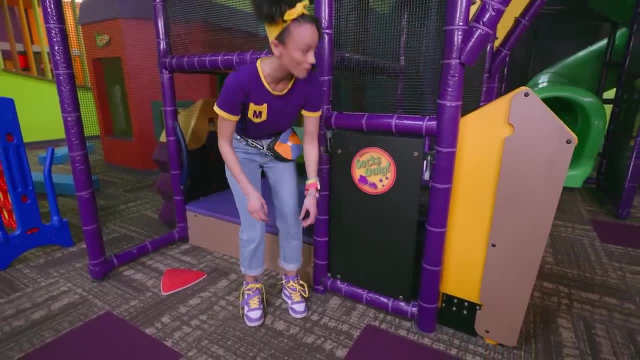 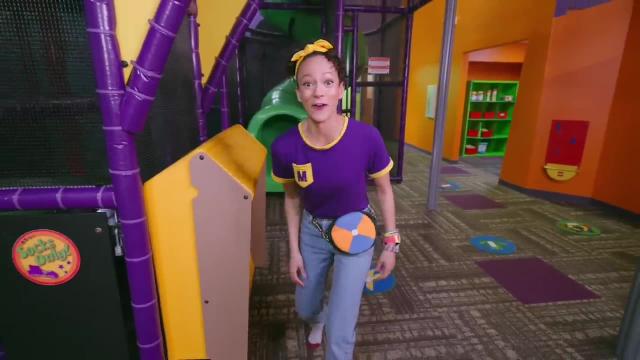 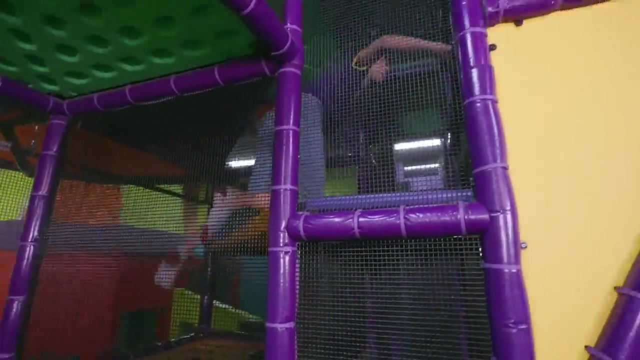 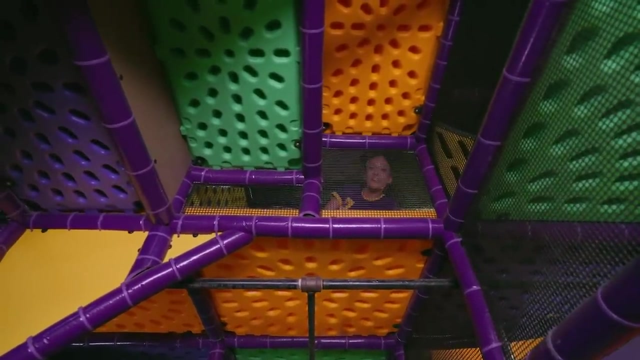 All right, Let's. Oh, they go in these cubbies over here. all right, i'm gonna go to the top and see if i can find something for our experiment. see you at the bottom. hi, i think i see something for our experiment. i'll see you soon. 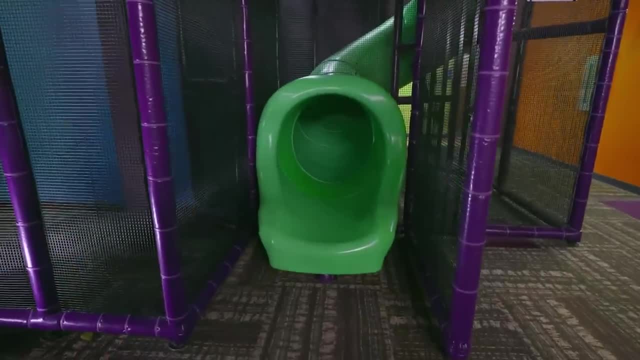 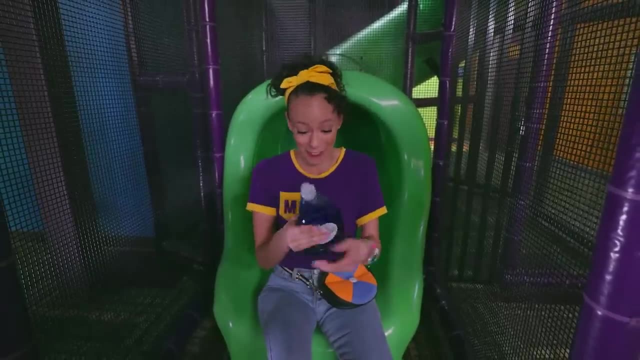 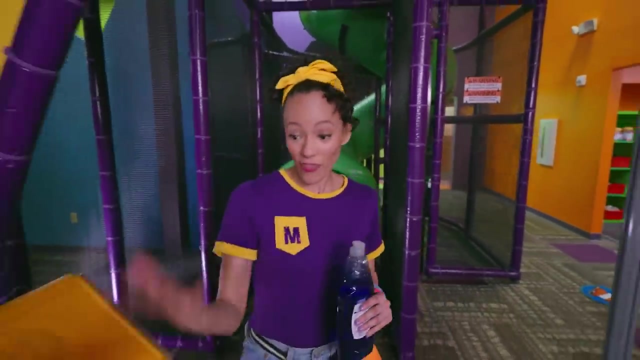 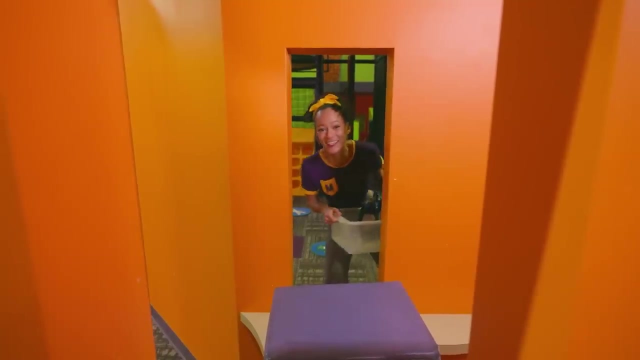 look what i found: dish soap. we definitely need this for our experiment. i'm so excited. thanks for your help. all right, i'm gonna grab my shoes and our other items for our experiment and we can keep looking. we have two more to find. come on, hello, let's keep looking. 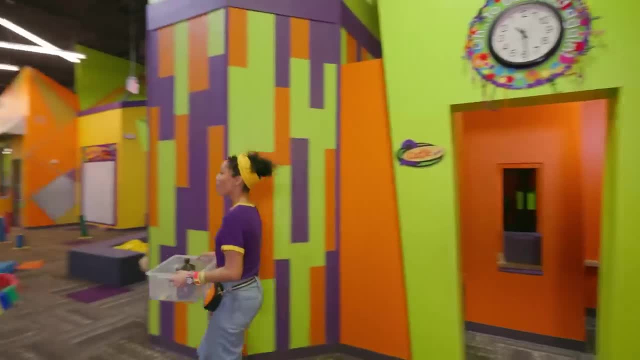 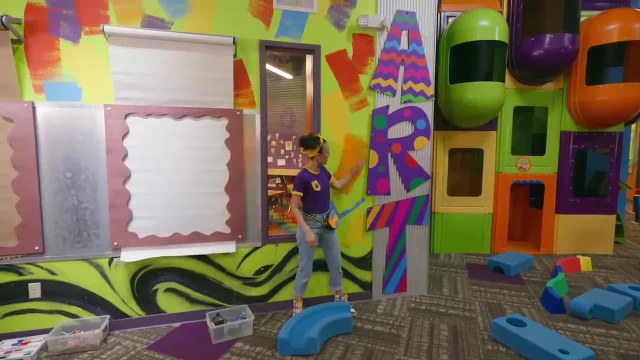 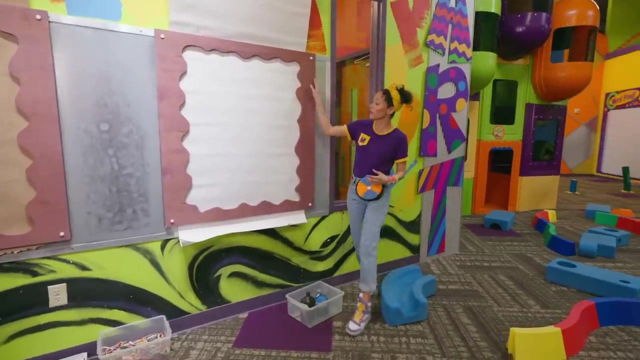 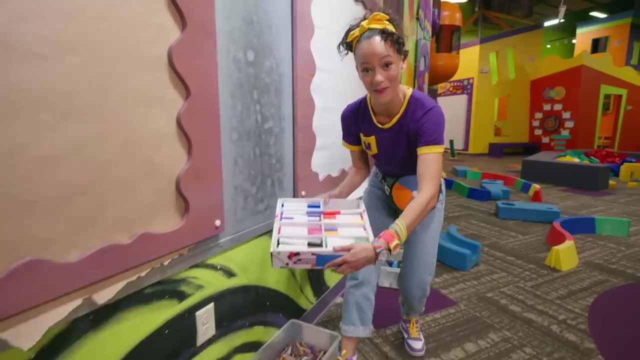 cool clock, whoa. look over here. it says a r t art. this is an art space. cool. look at this big piece of paper. oh, i could color something on here. oh, look at all of these markers. i'm gonna choose purple because it's one of my. 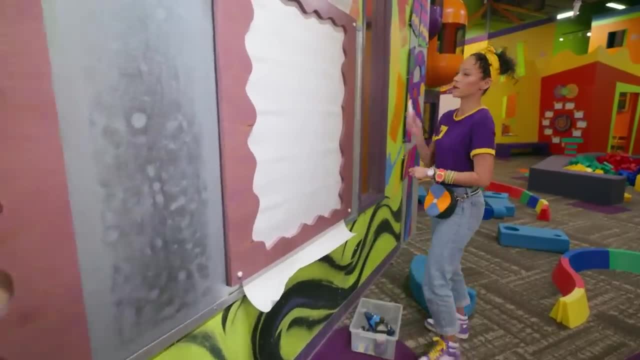 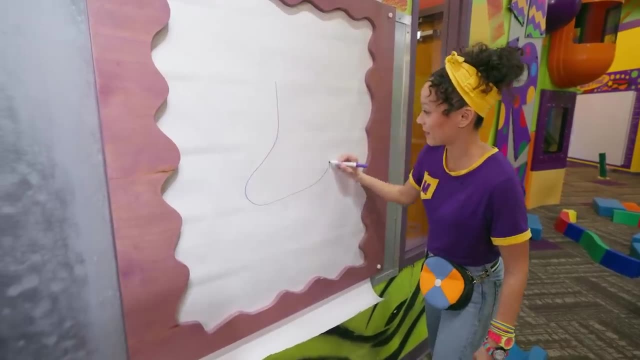 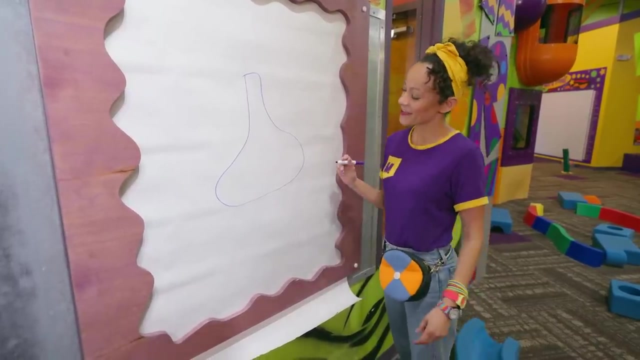 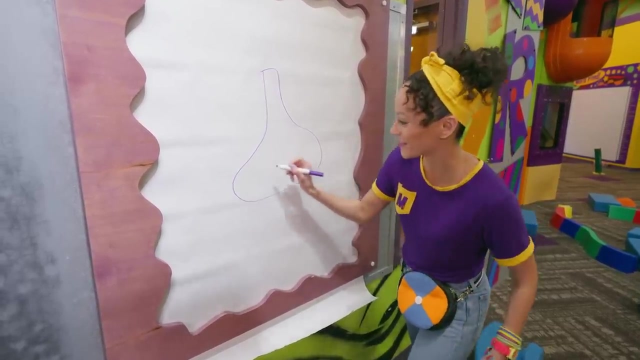 favorite colors. all right, let's. what should i draw? oh, i know, see if you can guess, it's a science flask. you can use this in a science experiment, but it kind of looks like something else. what do you think? okay, i'll give you a hint. do you know now? 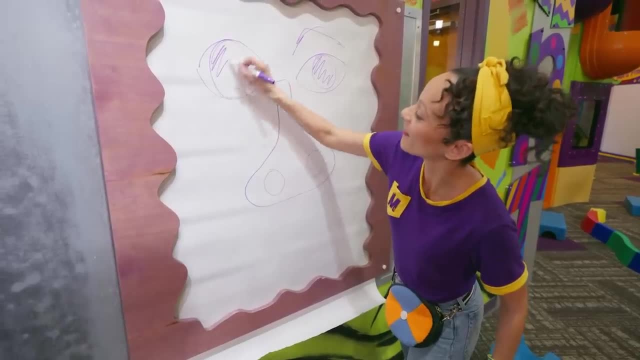 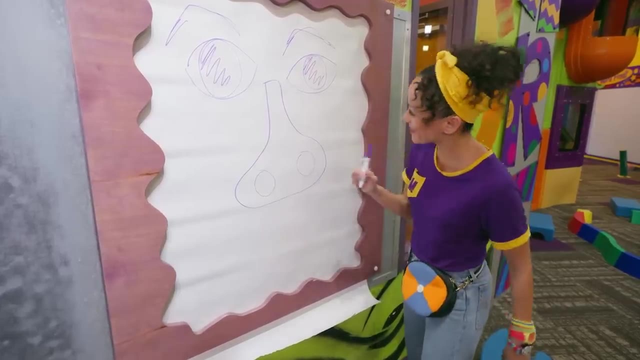 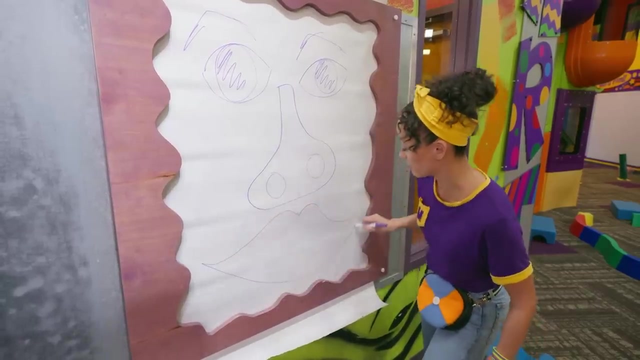 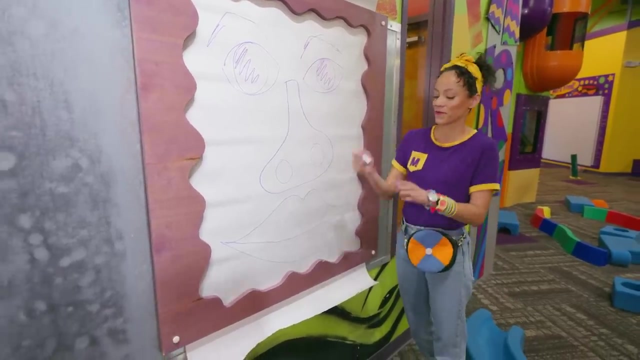 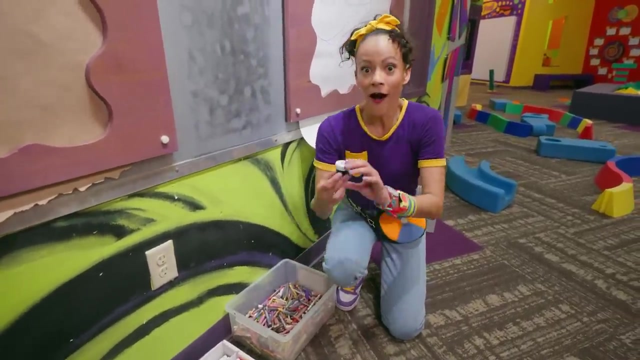 it's two eyes and a nose. what else does it need? oh right, a mouth. give it a big mouth, a big smile. hello, oh, there's crayons too. maybe i could put something else on here and choose a different color. let's see, um, oh, i found the food coloring. 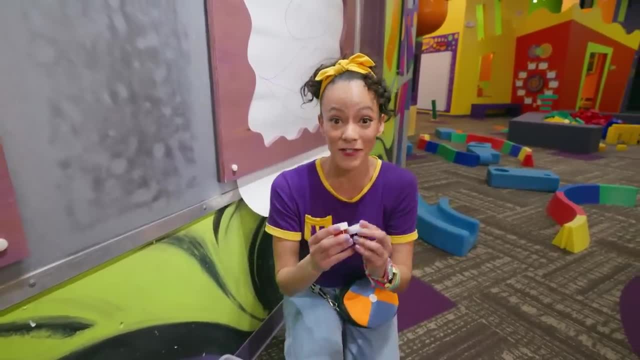 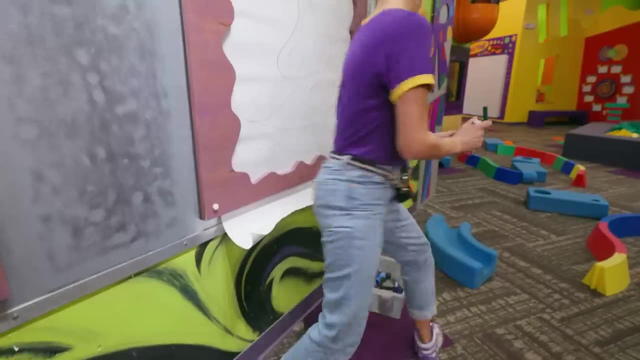 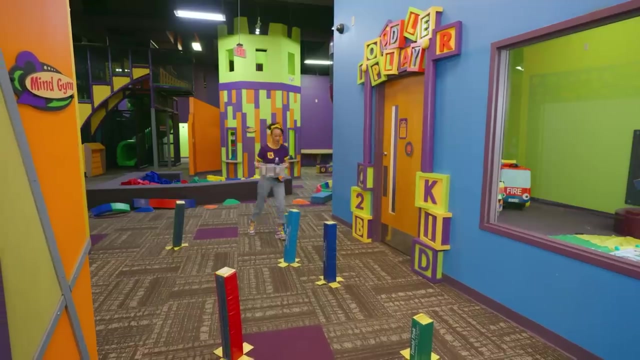 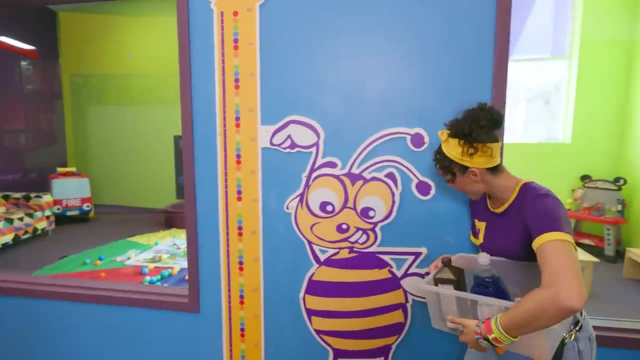 look, oh, and it's my two favorite colors, purple and yellow. we're getting closer and closer to finding everything we need for our science experiment. one more item to find: come on, whoa, hey, look at this hello cool bee. wow, it looks like this bee's measuring something. 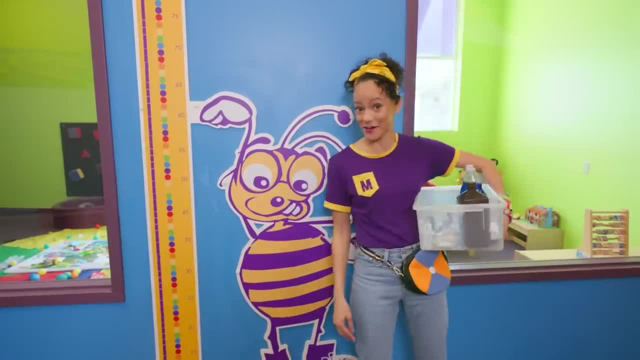 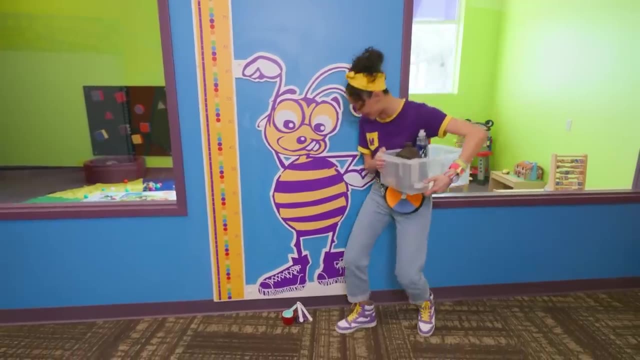 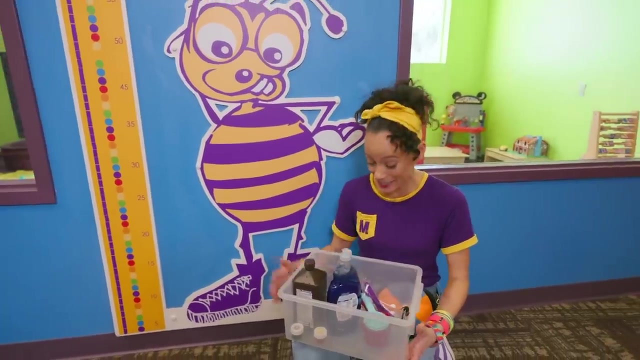 hey, mr b, i like your style. purple and yellow, two of my favorite colors. hey, it looks like we even have the same kind of shoes, measuring cups- that's the last thing we need for our science experiment. we found everything. let's head into the science lab, come on. 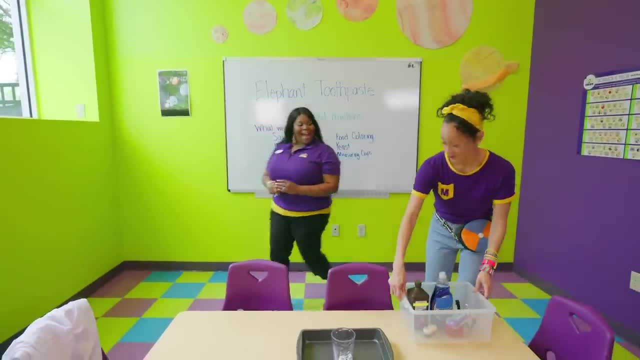 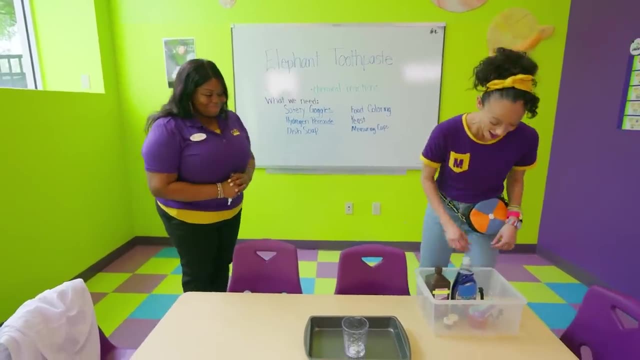 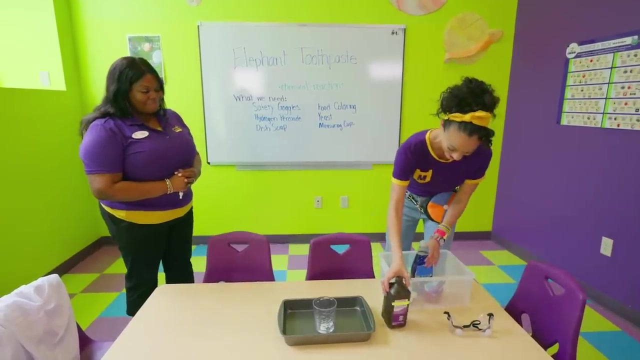 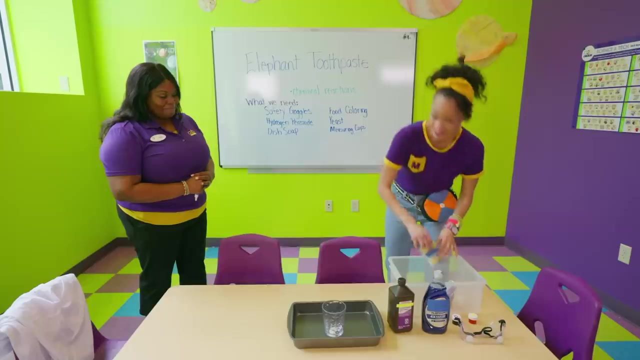 hey, Trudy, hi, Mica, welcome back. thank you. i think that i found all of the items i need for the science experiment. yay, may i see them? oh yeah, i have safety goggles, hydrogen peroxide, dish soap, food coloring, yeast and measuring cups. congratulations, Mica, you did it. you did it, Mica. 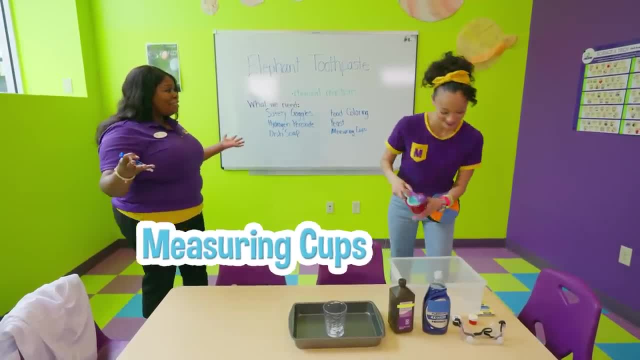 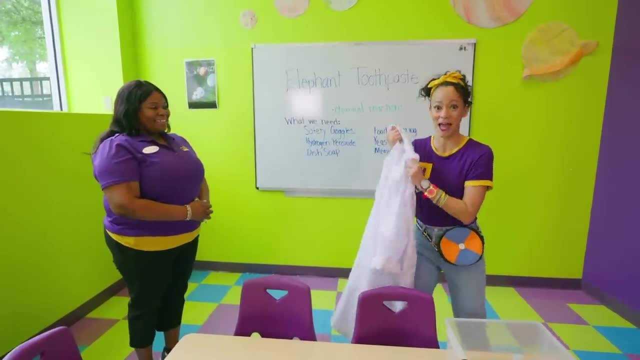 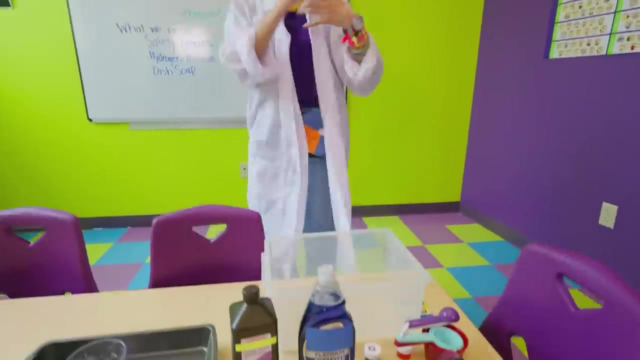 here you go, thank you, thank you, you did it, thank you, thank you, thank you. you are ready for the experiment. wow, really you go. oh, thank you so much. an official lab coat- awesome, enjoy. thank you. i'm so excited to do this experiment. okay, everyone, safety first. 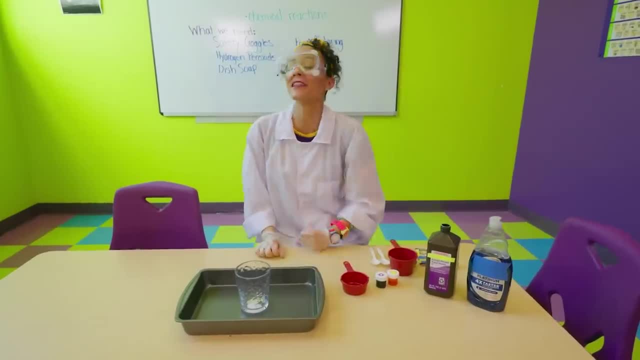 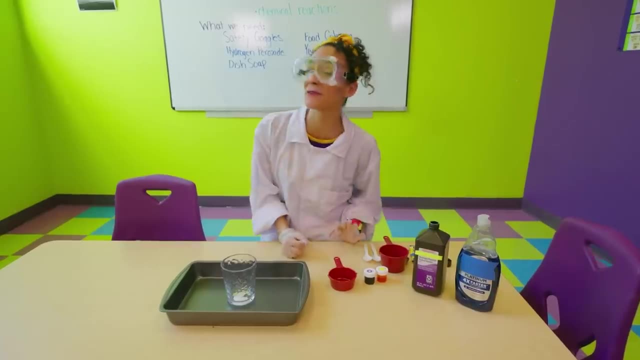 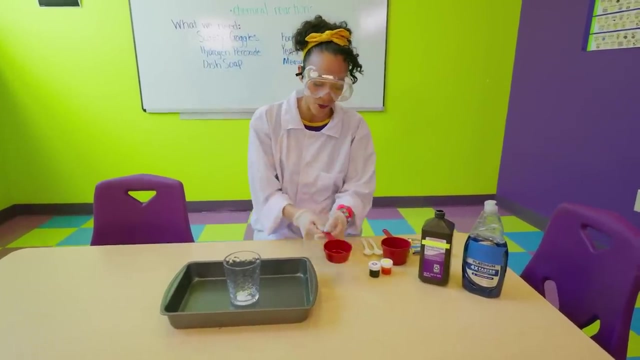 if you're doing this experiment at home, please make sure to do it with a grown-up. we are going to make elephant toothpaste, but remember, it's not really toothpaste, so please don't use it on your elephants. the first step is we need to pour half a cup of hydrogen peroxide. 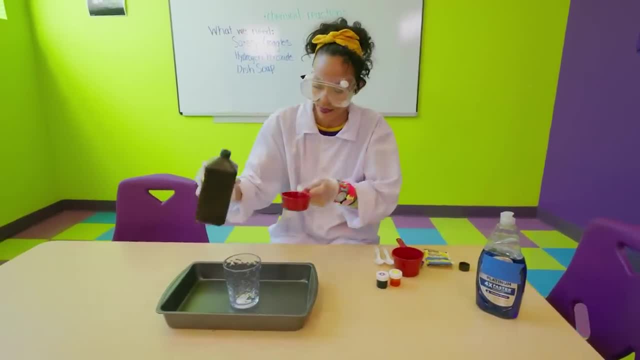 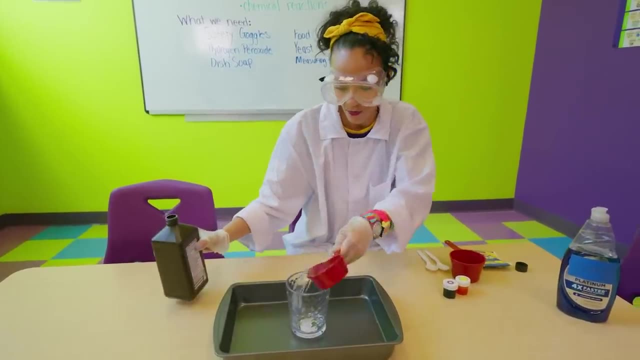 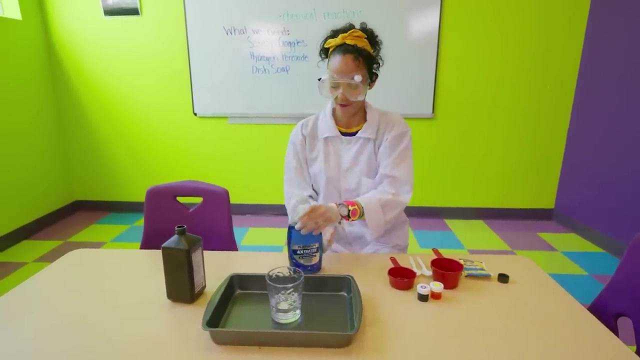 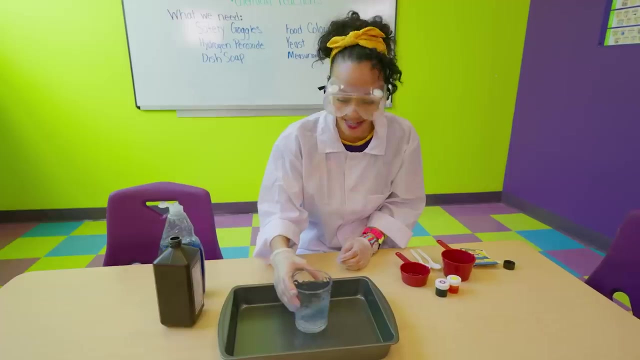 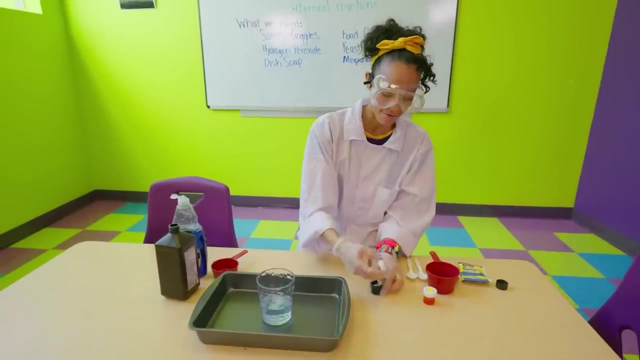 into this glass. okay, and be nice and careful and pour it to the top. okay, step one, complete second: we need our dish soap. okay, squirt of dish soap in there and you swirl it around, make sure it mixes a little bit together. okay, that looks pretty good, and now i'm going to add two of my favorite colors: purple and yellow. 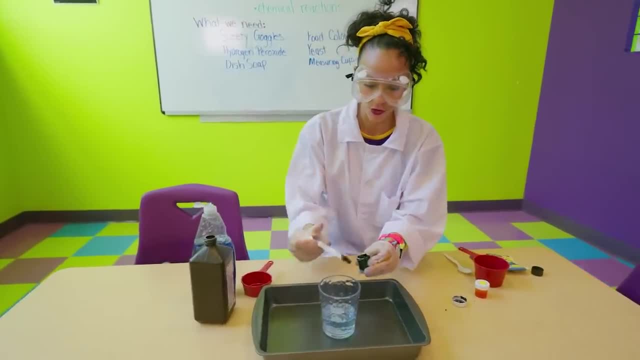 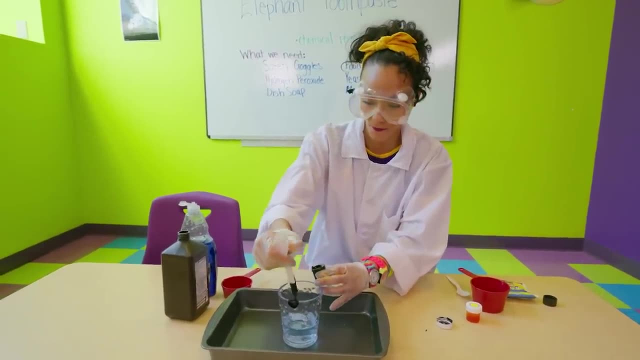 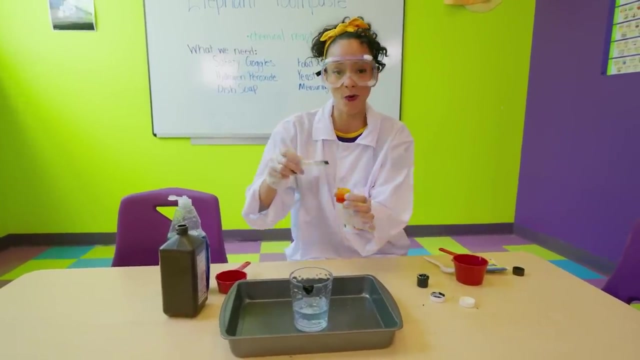 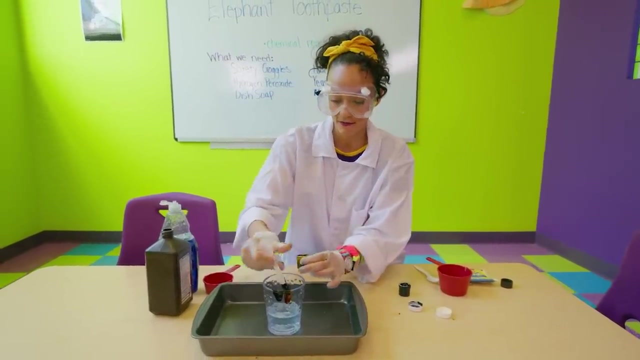 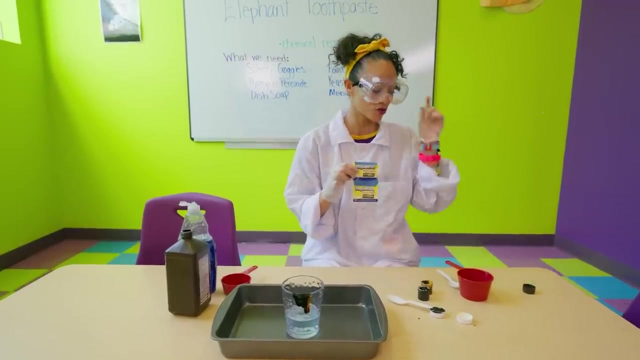 okay, get a little goop there. it looks black, but once it all mixes together it's going to look purple and yellow and look the yellow looks orange, but once it comes out of the cup it's gonna look yellow. okay, all right. next we are going to add our yeast to some warm water, and i already have some. 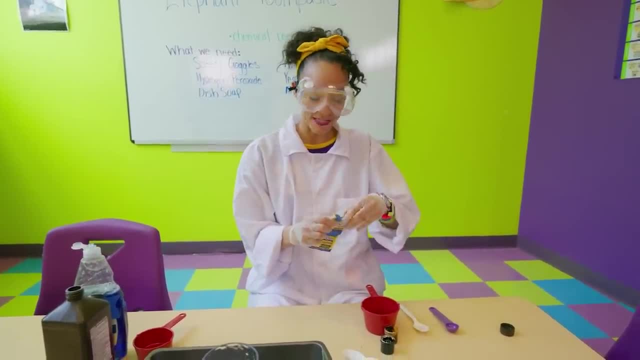 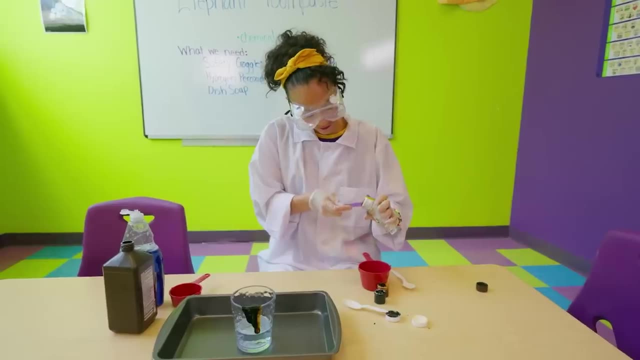 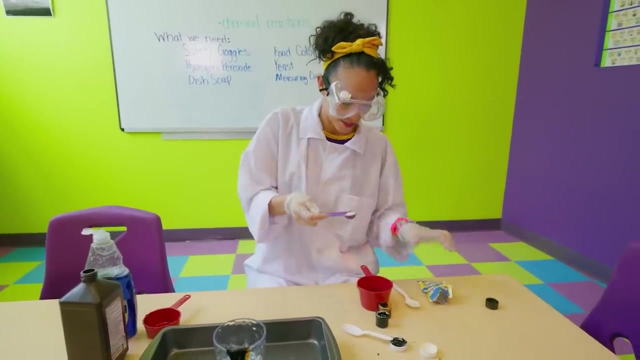 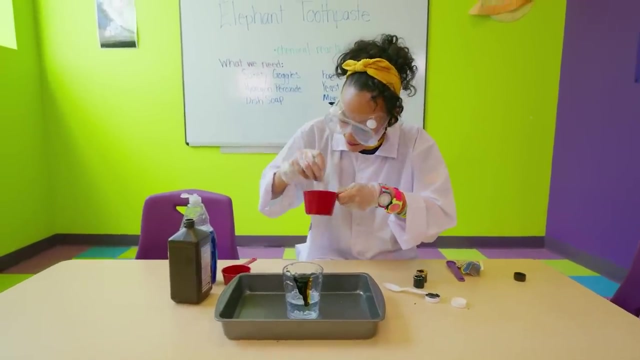 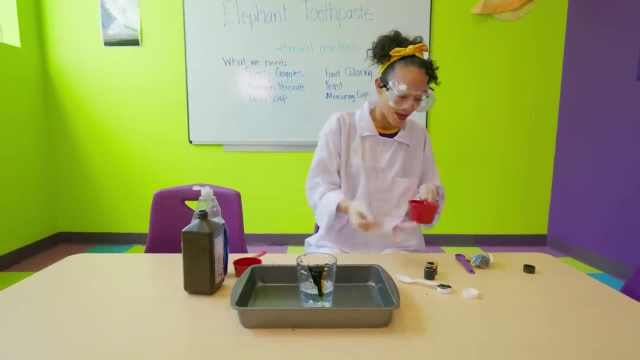 warm water right here and you only need one teaspoon. let me open this up and get one teaspoon of yeast. okay, there we go, one teaspoon, add it to the water and stir it around. see, it's all mixing together, okay, and then we're gonna add it to the glass and hopefully we will see our toothpaste in action. 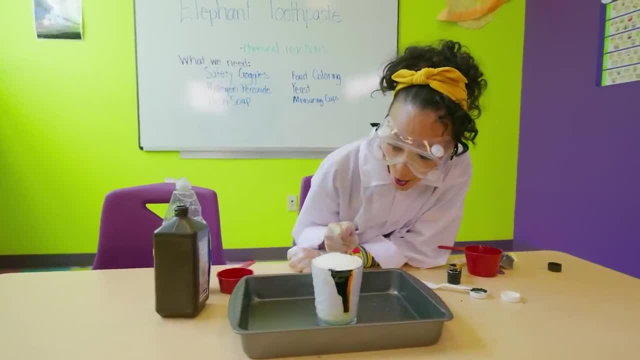 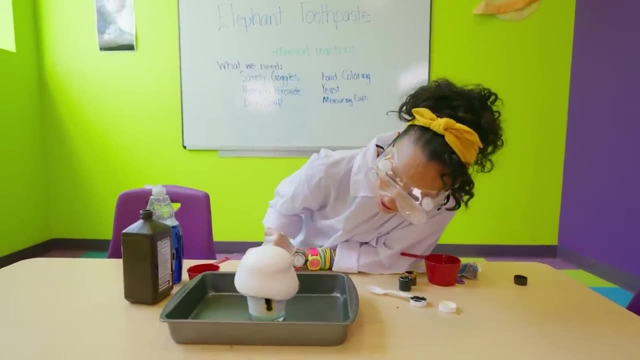 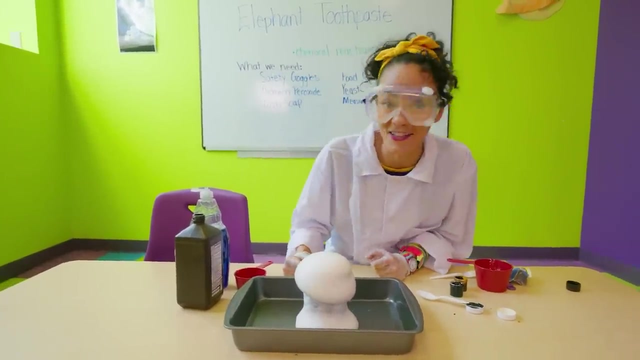 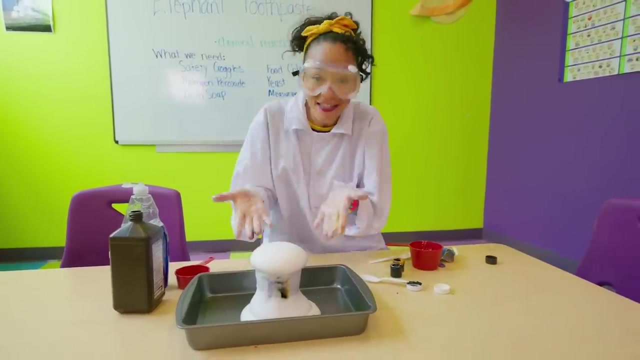 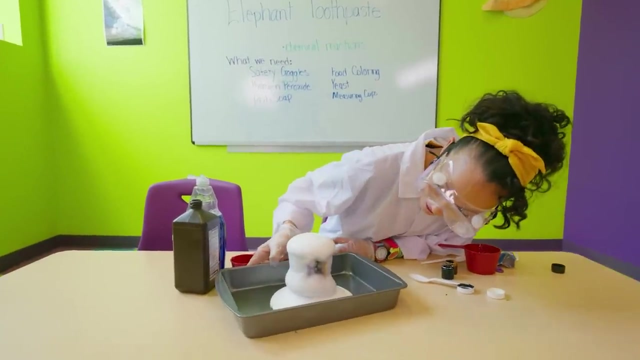 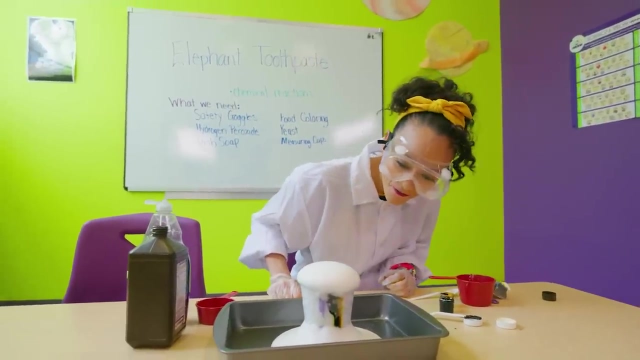 oh, it's going to the top. that's so cool. whoa, did you see some of the colors? wow, it really looks like toothpaste. oh, science is so much fun, isn't that cool? whoa, it's still going blue. there are the colors right there. oh, that was so fun. hey, thanks for helping. 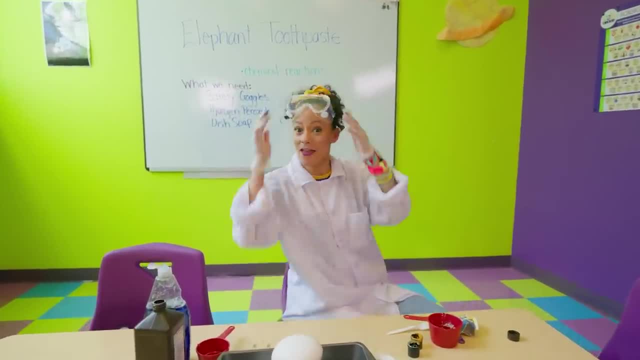 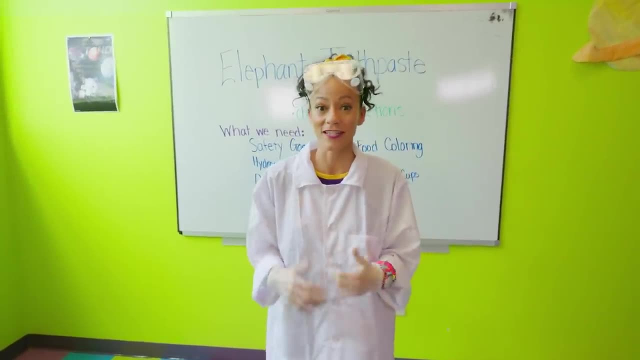 me find all of those items for our science experiment. you were very helpful. science is so fun and we had a lot of fun today. right, we went on a scavenger hunt, we did a word puzzle. oh, i went down a really cool green slide and there was a pretend grocery store. 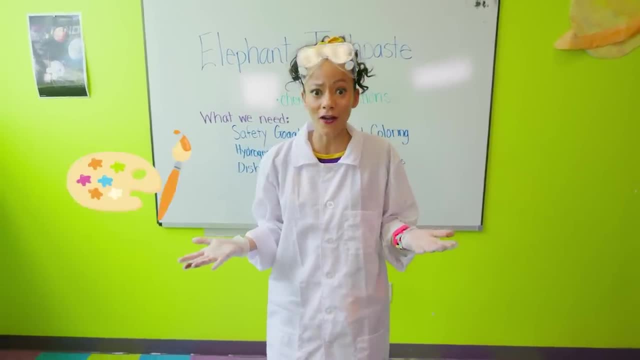 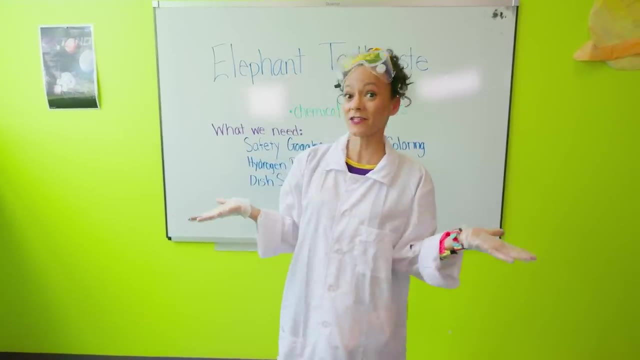 yes, i'm telling you, Grocery store and art. we did a lot today, All for the love of science. Well, that's the end of this video. If you wanna see more of my videos, all you have to do is search for my name. 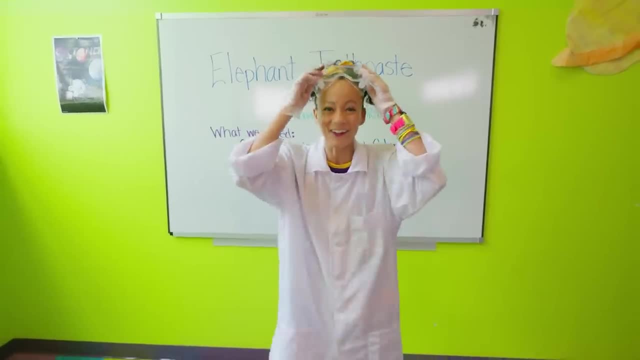 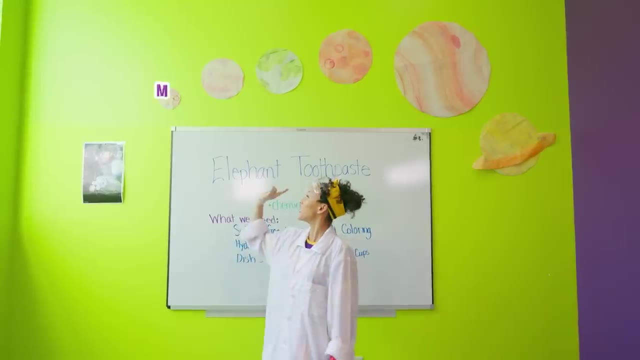 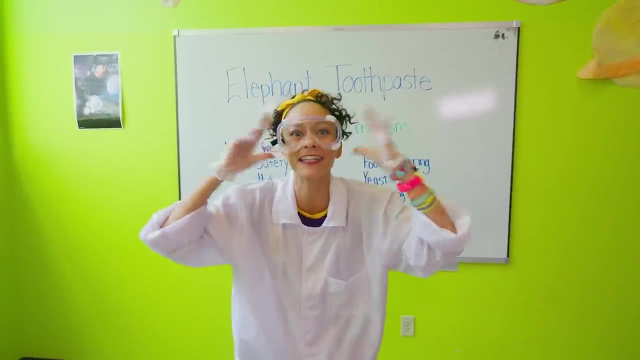 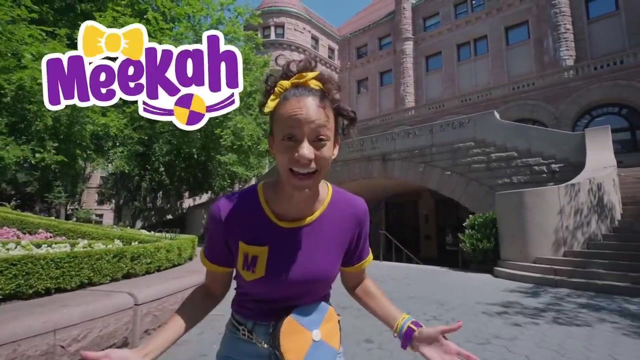 Hey, will you spell my name with me? Cool, Should we spell it on the planet science style? Let's do it M-E-E-K-A-H. Mika. Thanks for learning with me. See you soon. Hi, it's me Mika. 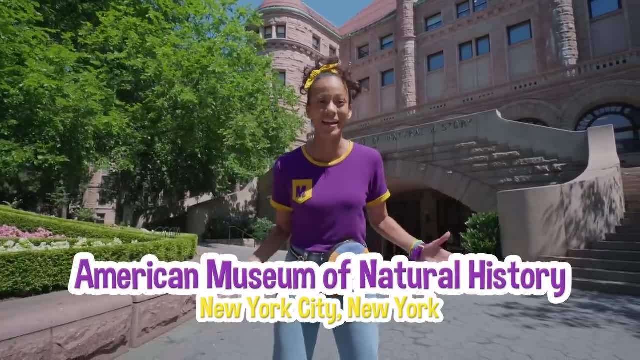 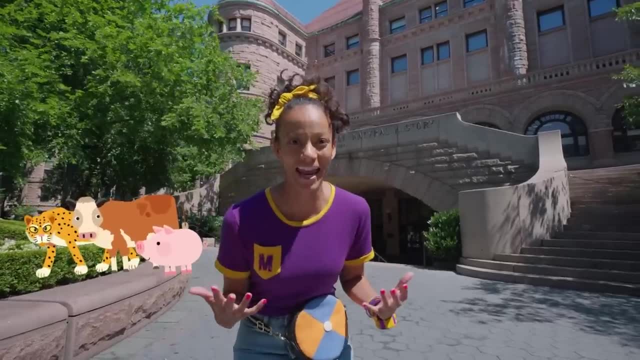 And today I'm at the American Museum of Natural History in New York City. Do you know what's inside of this museum? All different kinds of animals and dinosaurs, And I heard that they have one of my favorite dinosaurs, a T-Rex. 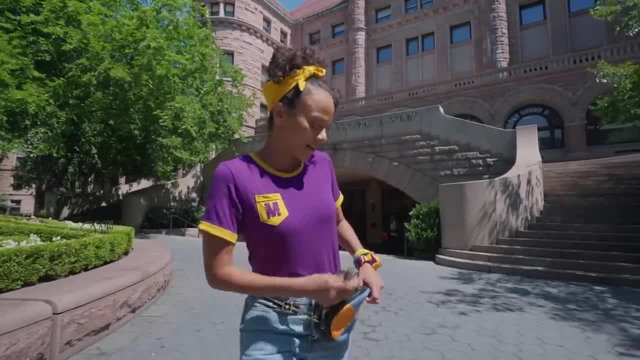 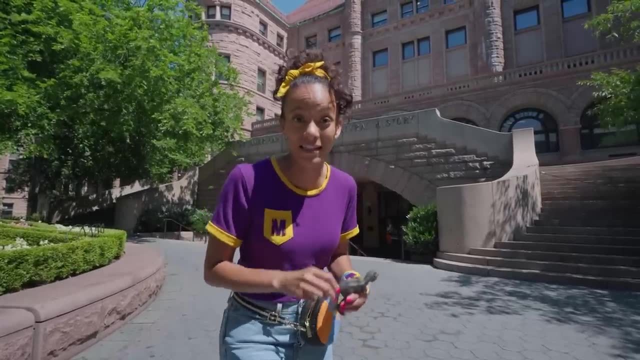 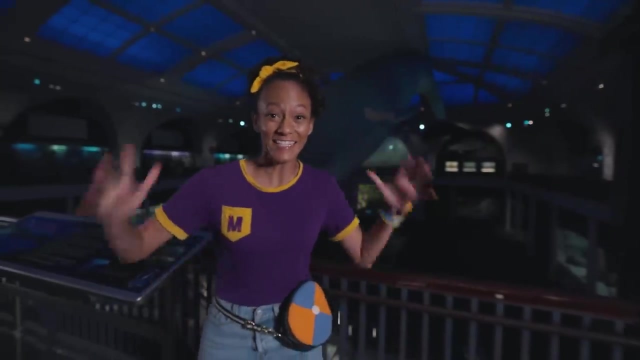 Do you know what a T-Rex looks like? I have one in my jam pack. Whoa, here it is. Hey, will you come with me and see if we can find a T-Rex inside? Let's go. Whoa, I'm inside of the museum. 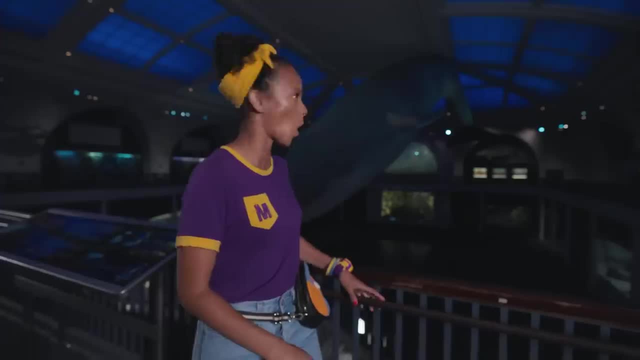 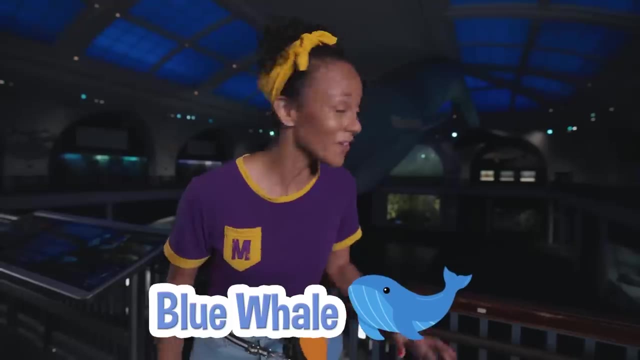 I can't wait to find the T-Rex. Whoa, that is definitely not the T-Rex. Do you know what that is? It's a blue whale. Oh, and look, I see a bandage on that whale. Even whales get boo-boos. 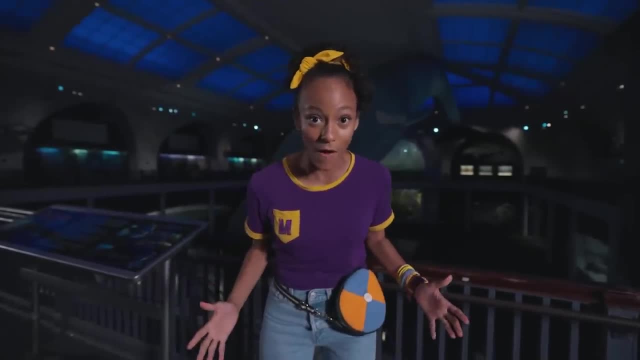 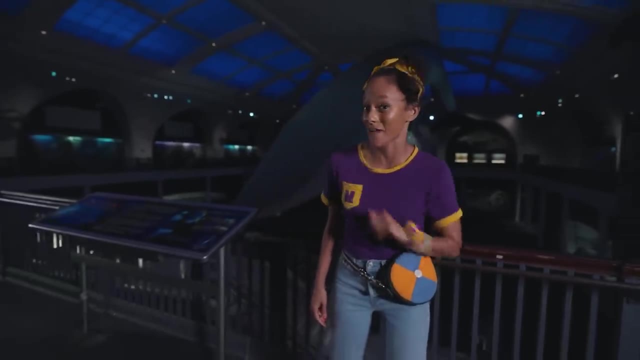 Did you know that the blue whale is the biggest animal on the planet? It's so cool. Oh, I see someone over there who works at the museum. I bet they have more whale facts. Come on, Oh hi. Hello, I'm Mika. 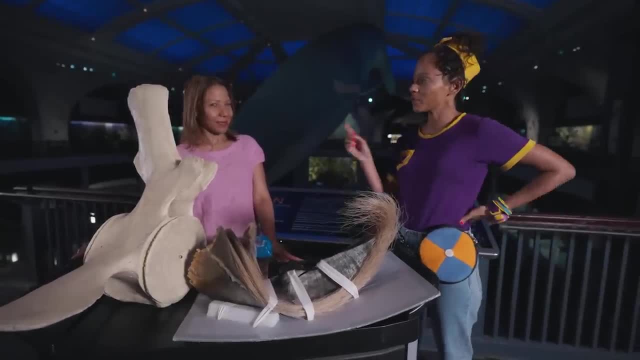 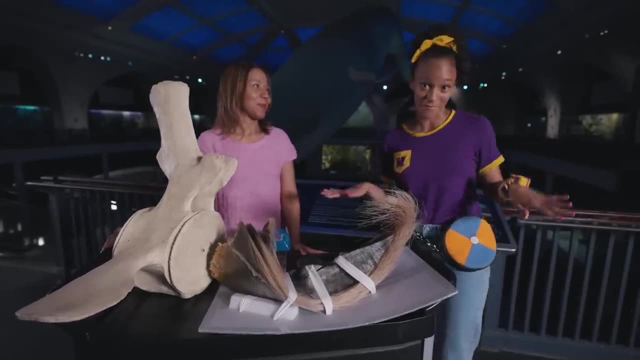 What's your name, Alexandra? Hi Alexandra, So I bet you know something about the blue whale. Yes, You do. What do you do here? I'm an educator, Oh, an educator. So, yeah, you definitely know What do blue whales eat? 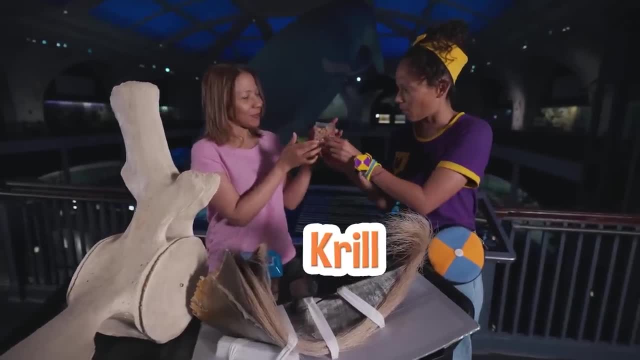 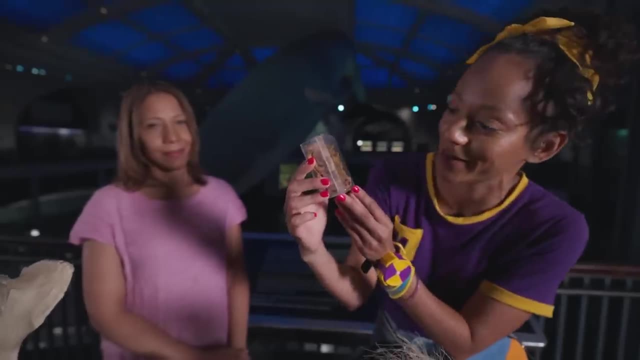 Blue whales eat tiny krill. Whoa, Look at these tiny shrimps. Can you believe a big blue whale likes to eat these tiny little shrimps? Wow, do blue whales have teeth like us? No, they don't have teeth. 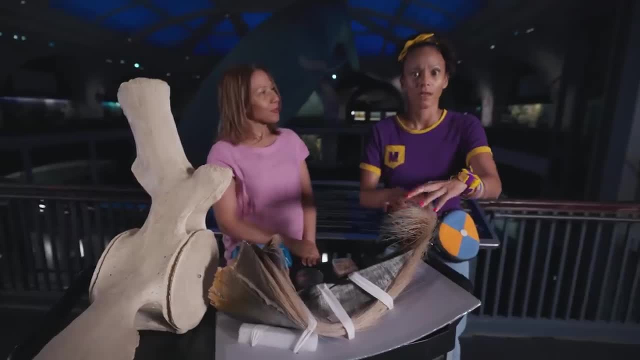 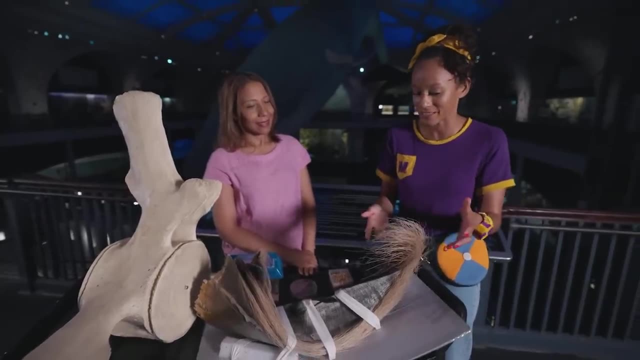 They have baleen Baleen, Oh whoa, It feels like straw. Can you imagine if you had straw in your mouth instead of teeth? Ugh. So how do they eat? They open up their mouth. OK, Very, very big. 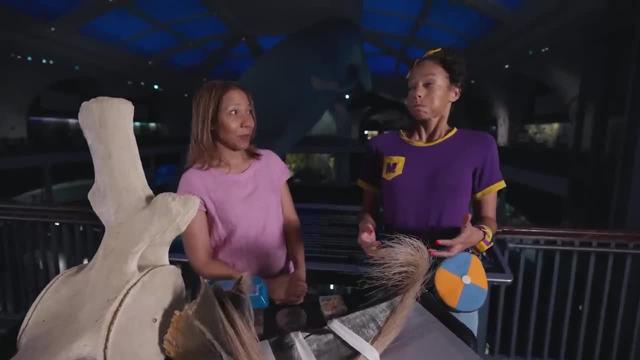 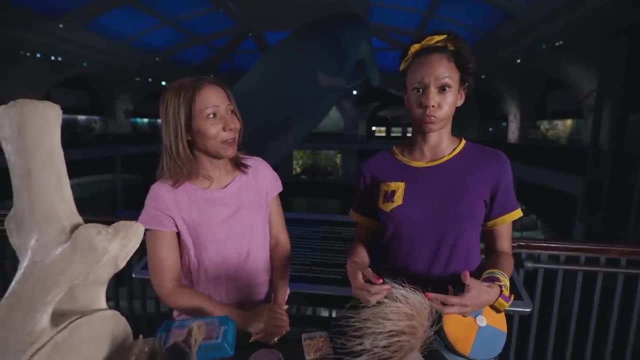 Uh-huh, Uh-huh, Uh-huh. They take a gulp of water, put krill in it, Then they push the water out with their tongue And what's inside The krill? Oh cool, That seems really complicated. 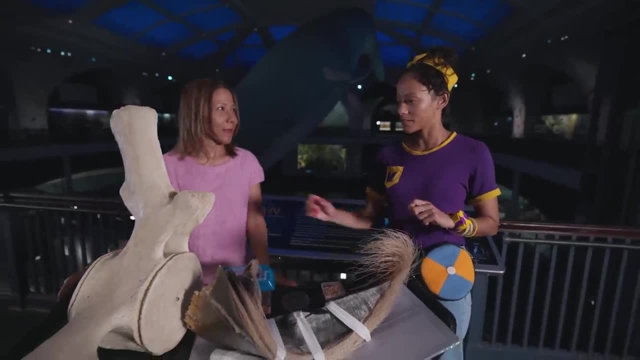 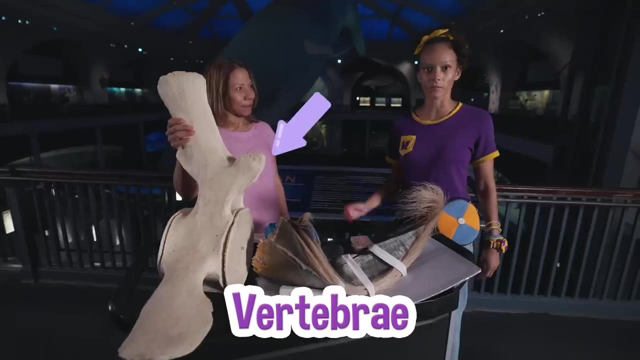 That is not how I eat at all. Wow, And what is that? It looks like a big bone. This is a part of the well vertebra, The vertebra- Well, we have those. You can feel it in your back. 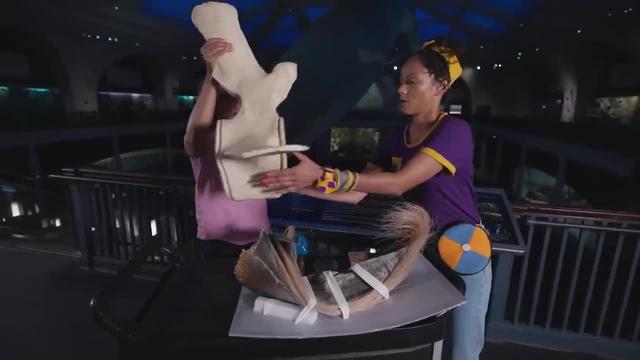 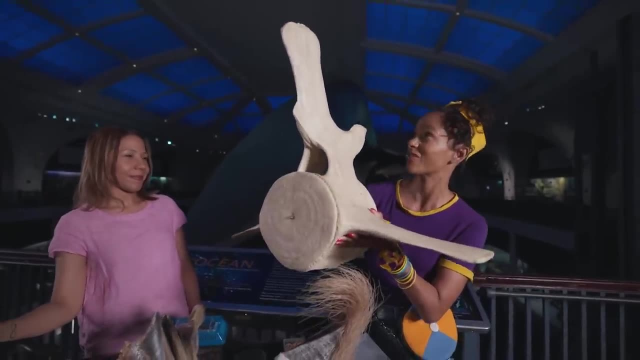 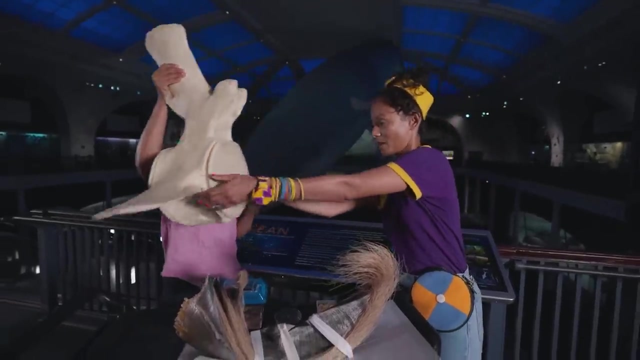 Yeah, Can I hold it? Yes, sure, Whoa. Oh, this is so heavy. Look how big this is. Ours are so tiny. Blue whales are huge. OK, Here I'll give that back to you Wow. 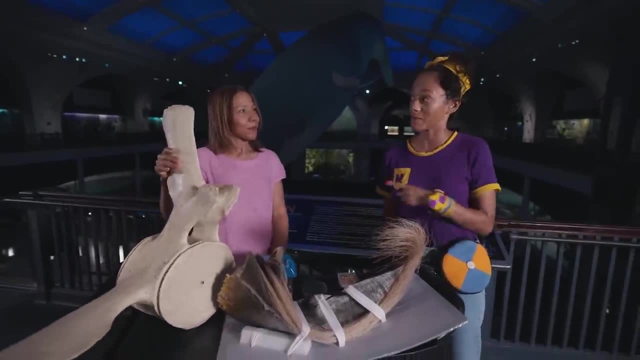 Well, thanks for sharing those facts with us. I'm going to keep exploring, but maybe I'll see you later. See you later, All right, Awesome, Come on. Where is the T-Rex? Where is the T-Rex? 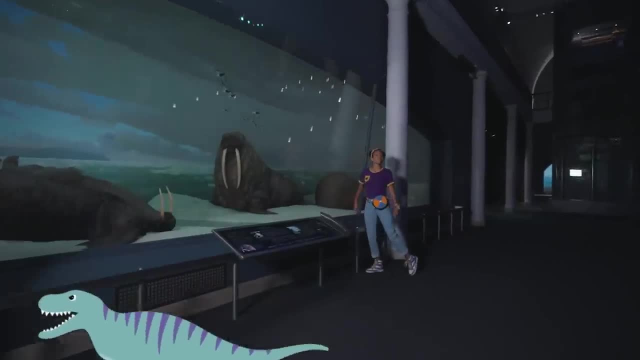 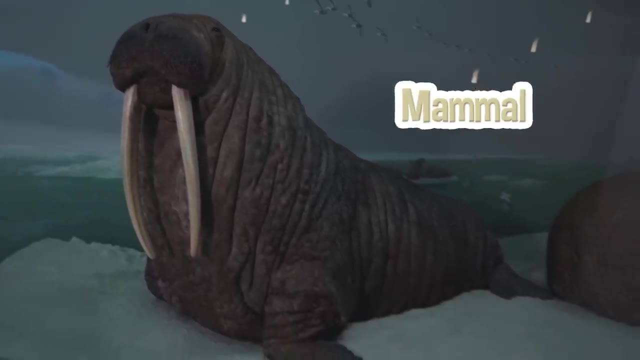 Where? where is the T-Rex? Whoa, That is not the T-Rex, but it is a very large mammal. Do you know what it is? It's a walrus, Not a real walrus. This is just a model. 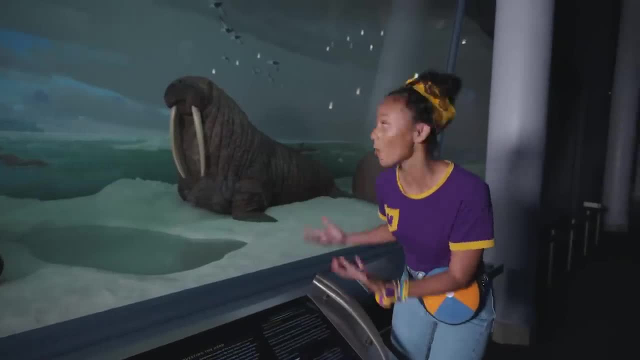 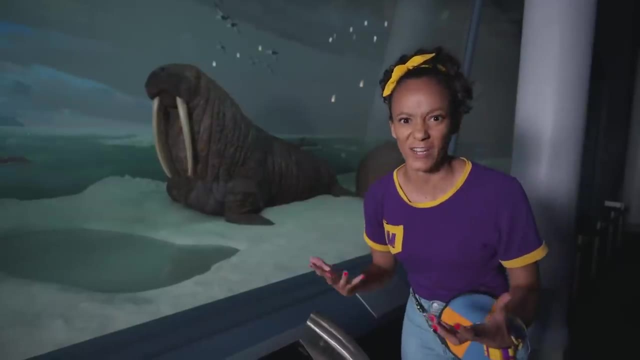 But this looks pretty much exactly like a real walrus. Whoa, Do you see those big tusks? They're made out of ivory and they're really strong and really sharp, And that one looks like the size of my arm, maybe even bigger. 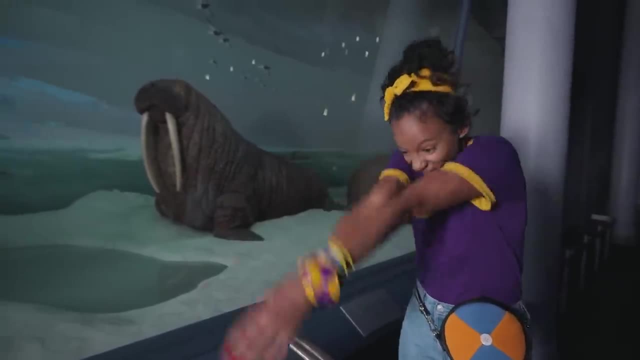 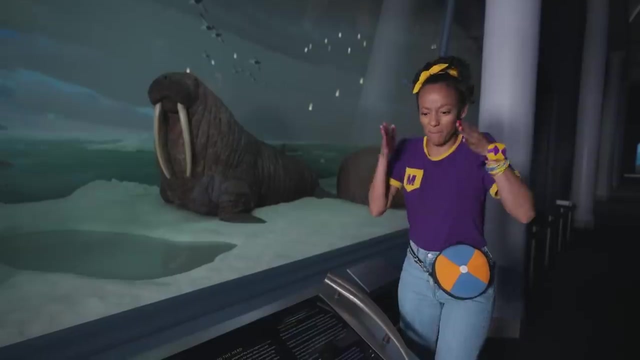 Whoa, Can you imagine if you had something that big hanging out of your mouth? Could you even find a toothpick big enough to clean that thing? Whoa, They can use them when they're in the water to poke into the ice and pull their bodies up. 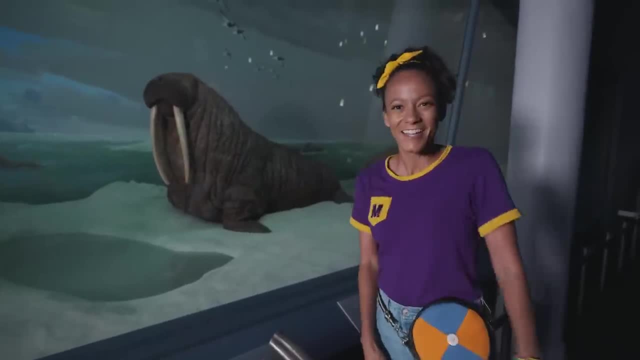 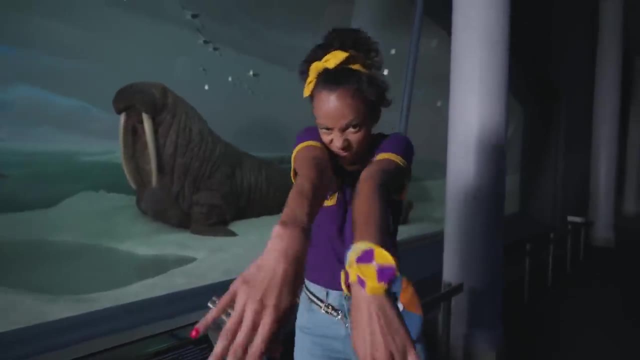 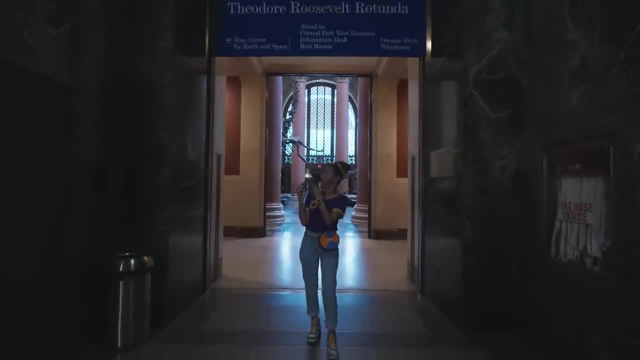 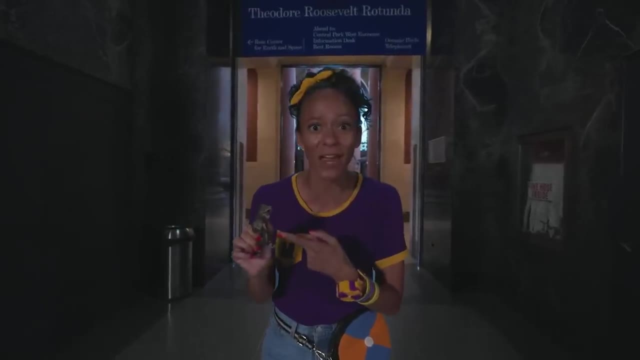 Mm, mm, mm, mm. oh, you're so funny. That's why you're my favorite. That is why you are my favorite dinosaur. Oh, hey, I'm still trying to find the T-Rex, but I don't see any dinosaurs anywhere. 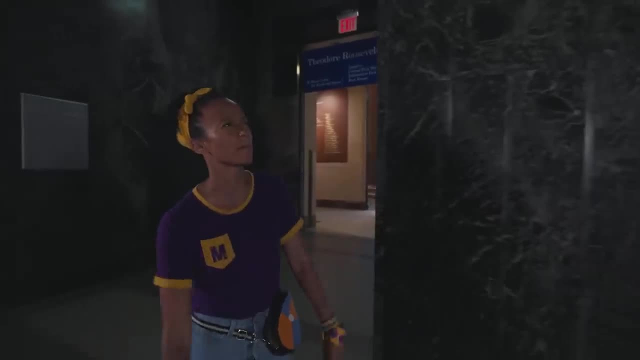 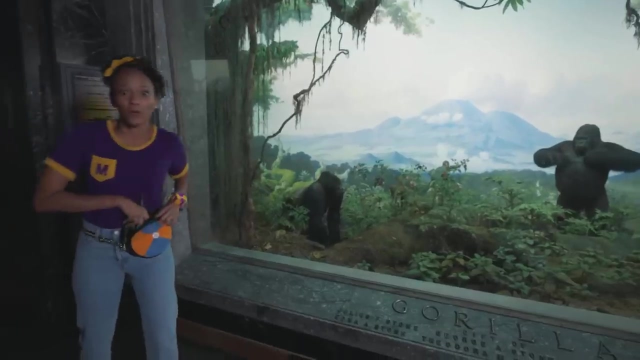 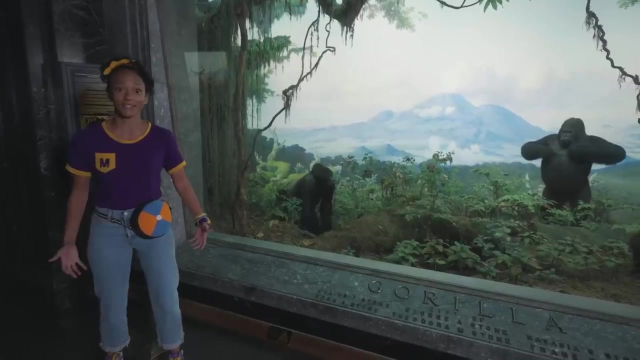 Let's keep looking over here. Maybe we can find something. Whoa gorillas. Gorillas are super cool. They're really big, They're really strong, They're hairy, They can stand up tall just like humans, But the male gorilla is 10 times stronger than a human. 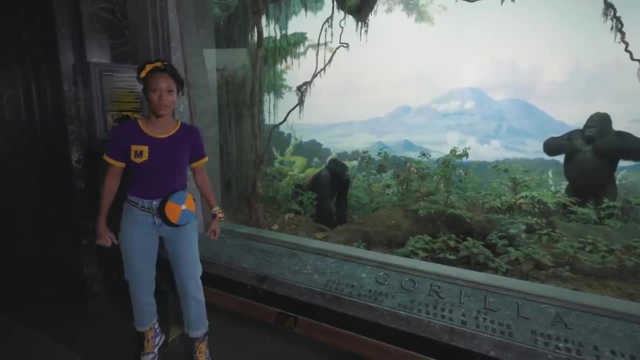 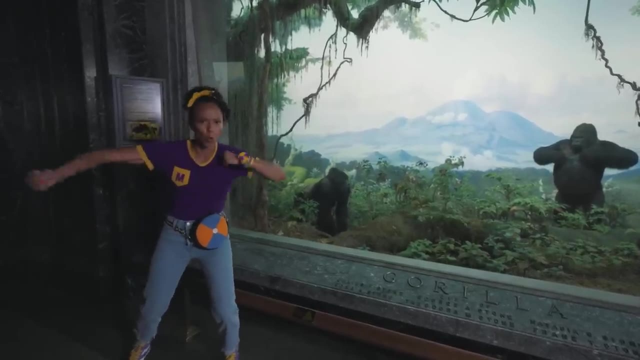 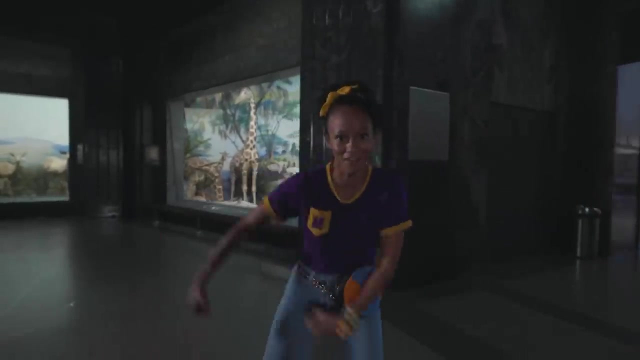 That's pretty strong. Will you act like a gorilla with me? All right, let me see your muscles Pound your chest. Let's keep looking for more animals. Whoa, yeah, I feel strong, just acting like a gorilla. 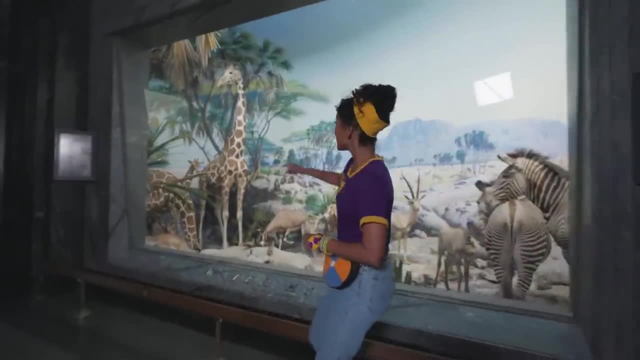 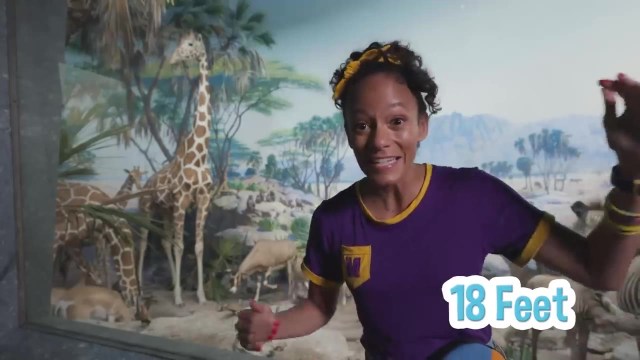 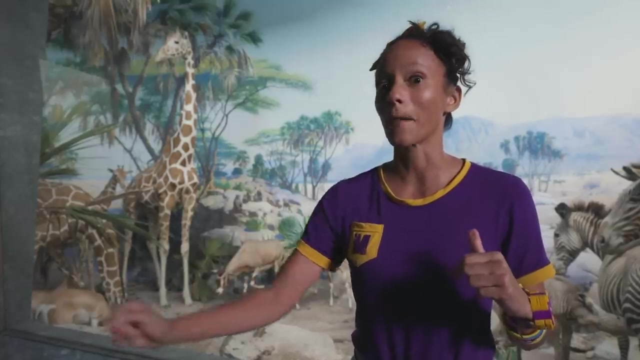 Whoa, check it out. See In the back there a giraffe. Giraffes are so tall, They can get up to 18 feet tall. That's really really, really, really, really tall And they have super long black tongues. 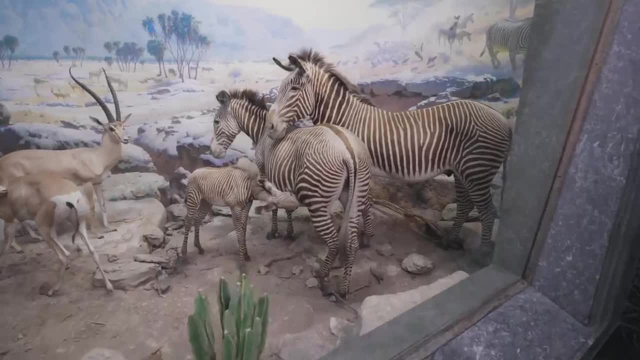 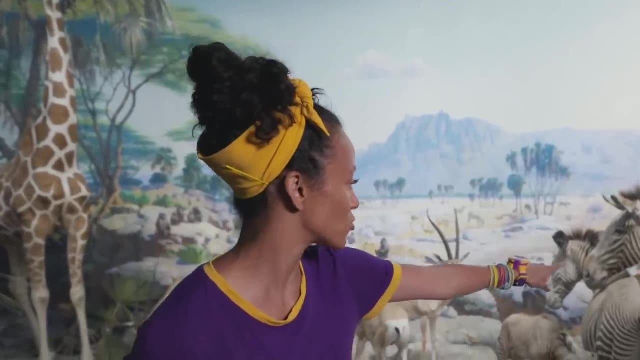 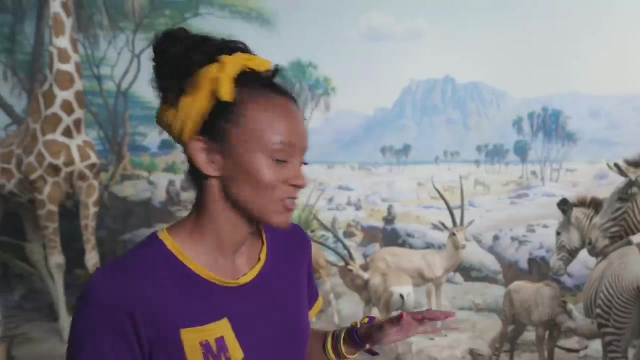 Isn't that cool. Do you know what that animal is? That's right, a zebra. Zebras are awesome. They have black and white stripes and a group of zebras is called a dazzler. Isn't that amazing? Check out that dazzle of zebra over there. 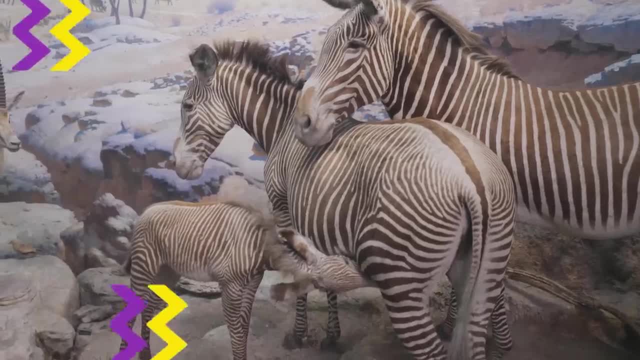 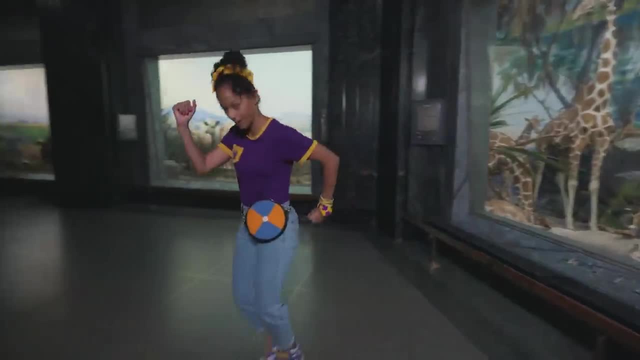 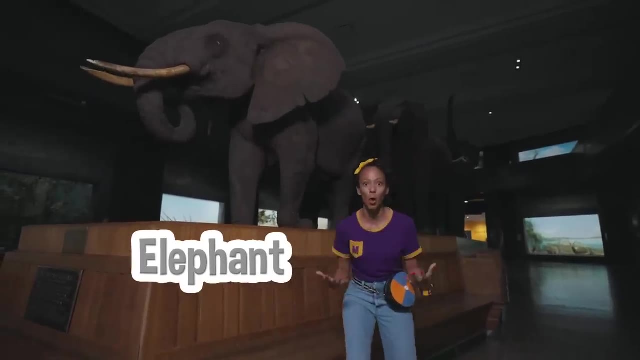 They run super fast and they can run in zigzags. Will you zigzag with me? All right, let's go Run and zigzag. Whoa. elephants are so big so they have to eat a lot of food. 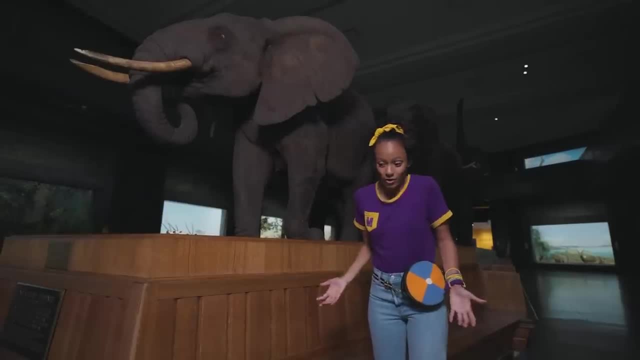 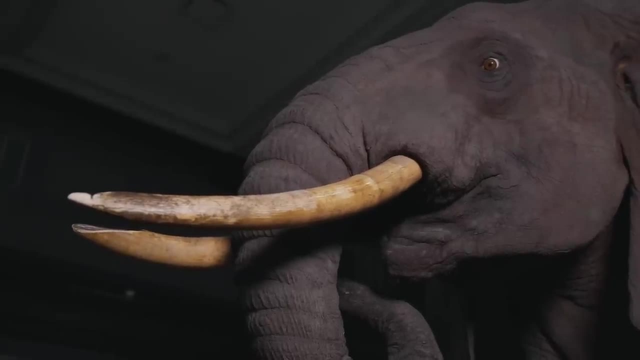 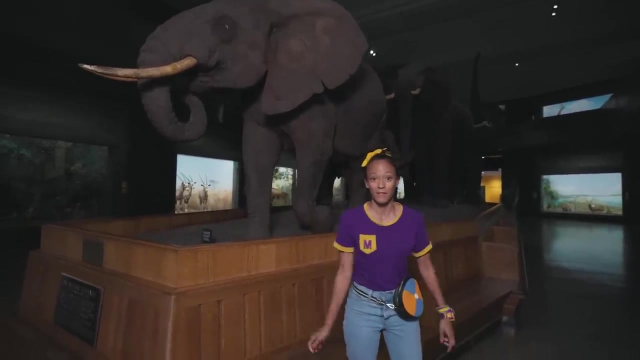 Actually, most of their day is filled with eating. They're herbivores, so they're vegetarians. They don't eat meat. Oh, and look, big tusks, just like those walruses. Hey, will you act like an elephant with me? 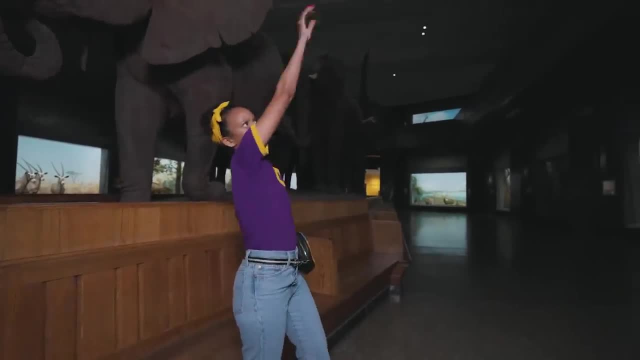 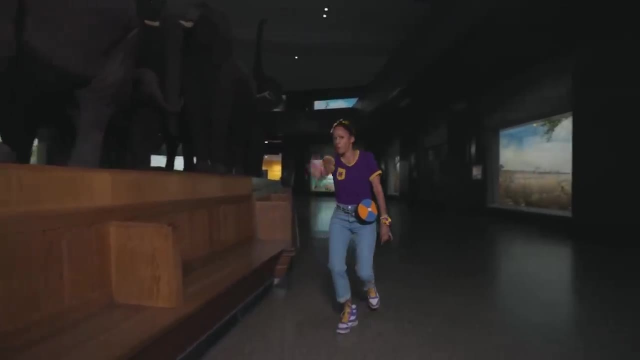 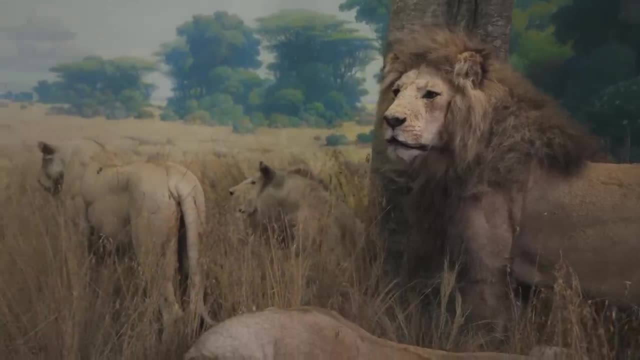 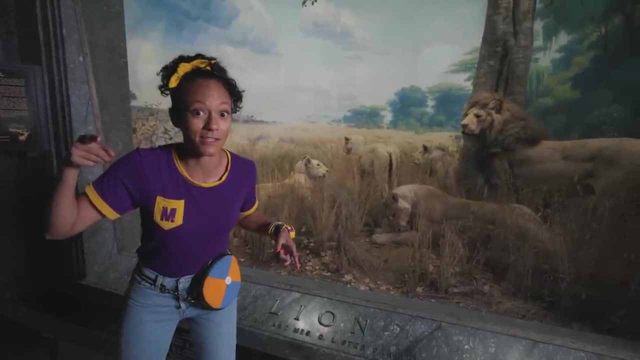 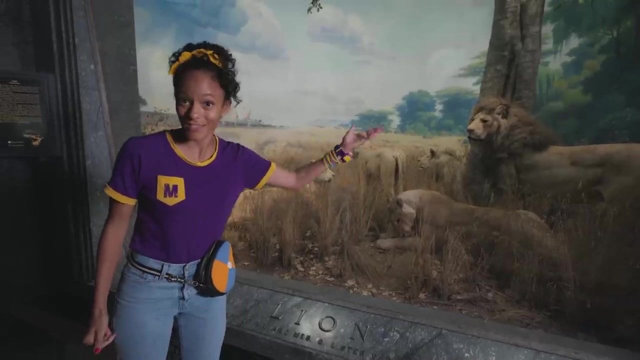 Hey, these really big cats are lions. I love lions because they have really big, Kind of like the T-rex. See that one with the mane, all of the hair. That's a male lion, That's how you know, because it has a mane. 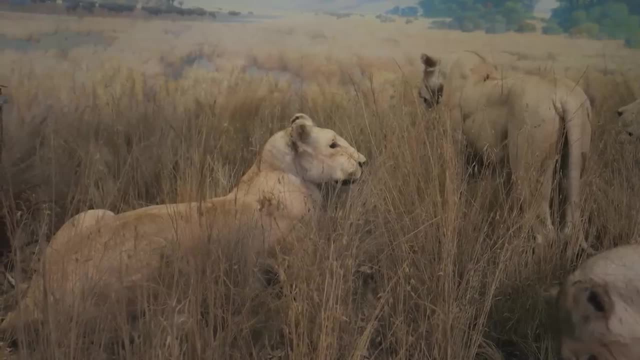 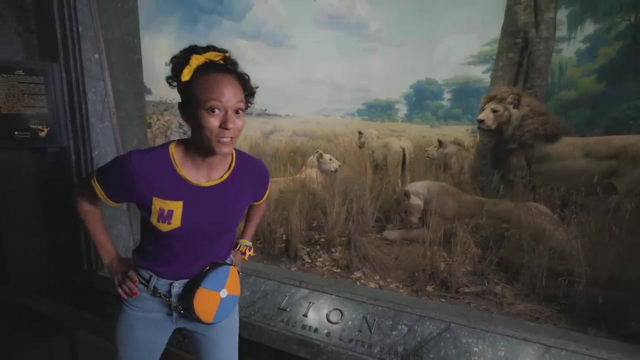 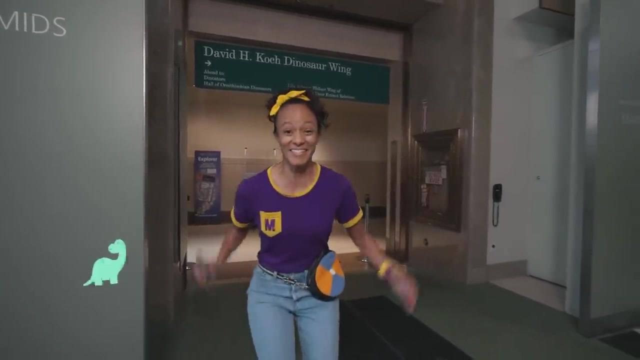 The other lions that don't have manes are females, and a group of lions is called a pride. I still don't see any dinosaurs, though. Will you keep looking with me? All right, come on? Wow, we're in the dinosaur room. 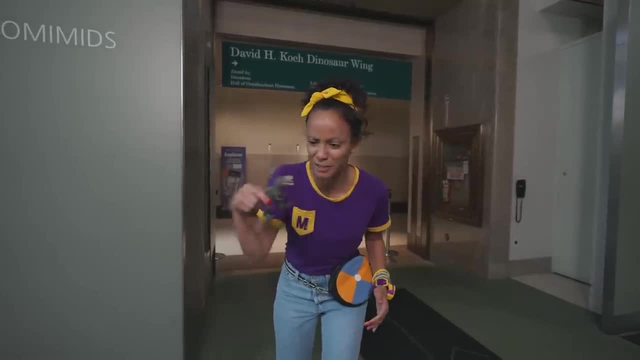 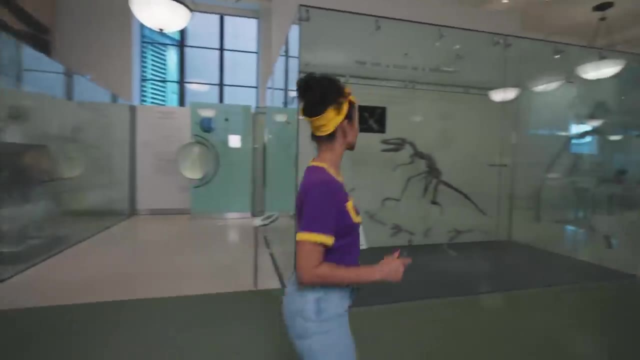 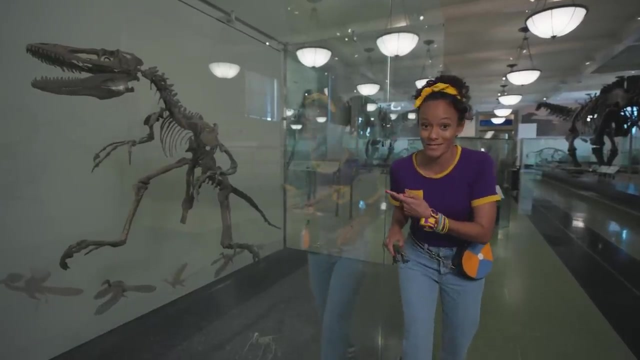 There has to be a T-Rex here, right? That means yes, Let's keep looking. Oh, there's a dinosaur over there. Ah, long tail, lots of teeth, but that's pretty small. A T-Rex is way bigger than that dinosaur. 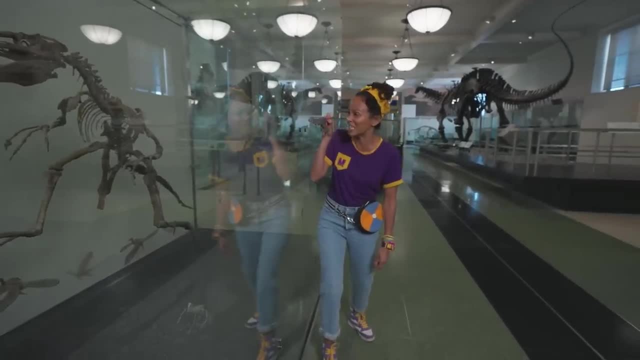 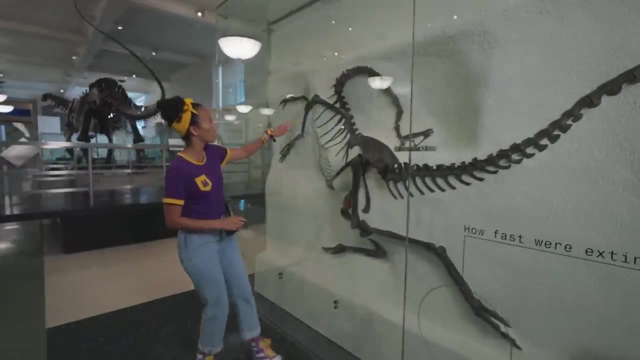 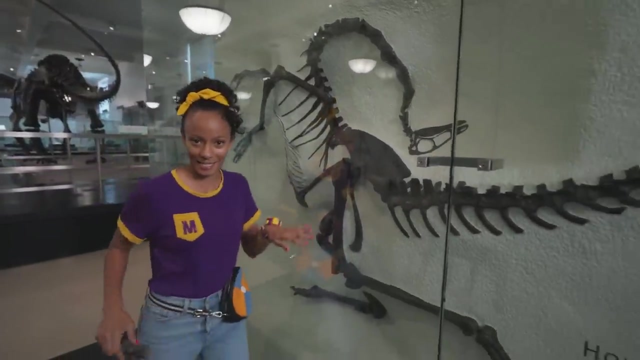 It's almost as little as this toy dinosaur. Hello, Oh, look at this dinosaur. Whoa has a long neck. Its head is going back really far. Oh, I wonder if it's a dancing- Nice move, But not a T-Rex. 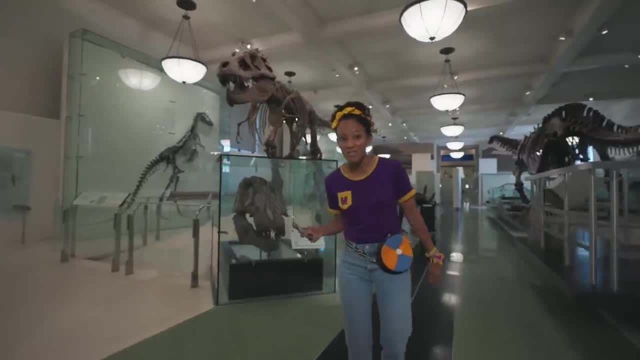 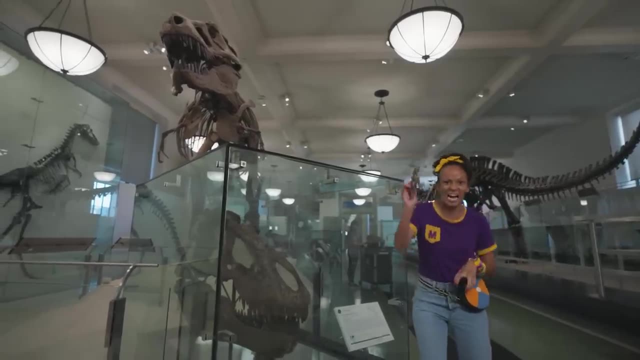 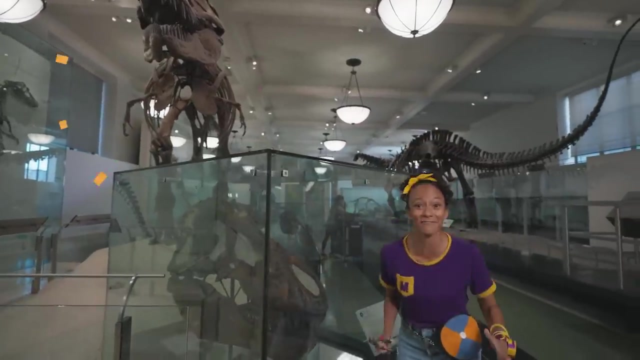 I can't see the T-Rex anywhere. Do you see? a T-Rex Looks like this big head, so many teeth, really big talons. It's right there, the T-Rex, my favorite dinosaur, Whoa. look how big the head is. 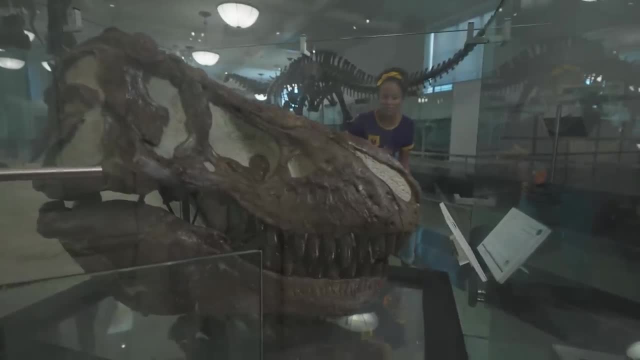 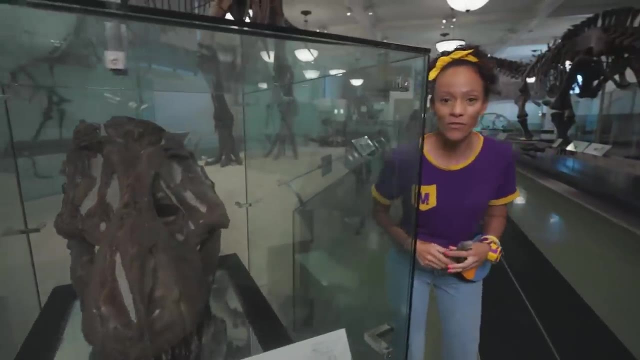 Whoa, See those big jaws with tons of teeth. Wow, they're so sharp And there's so many of them. Did you know that the T-Rex could have up to 50 to 60 teeth in its mouth? That's a lot of teeth. 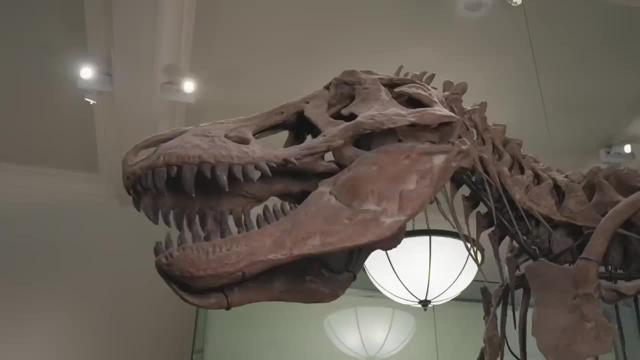 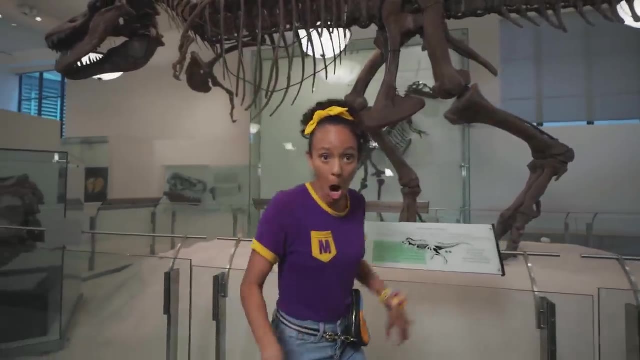 Whoa, you can see the whole body of the T-Rex: The head, the ribs, the big legs, the big feet. Roar, roar, Oh, hello, Hi, Oh, hello, Hi, Hi. I'm Mika. 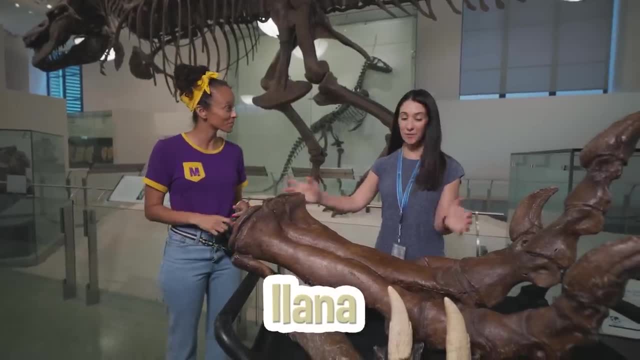 What's your name? Hi, my name is Alana. Hi, Alana, What do you do here? I'm a museum educator, Whoa, a museum educator, So you must know a lot about dinosaurs. I do, Oh, cool. 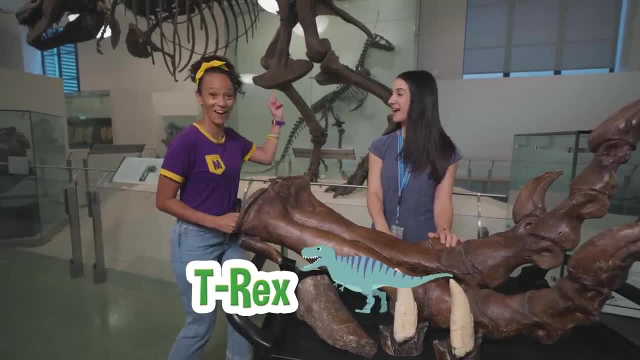 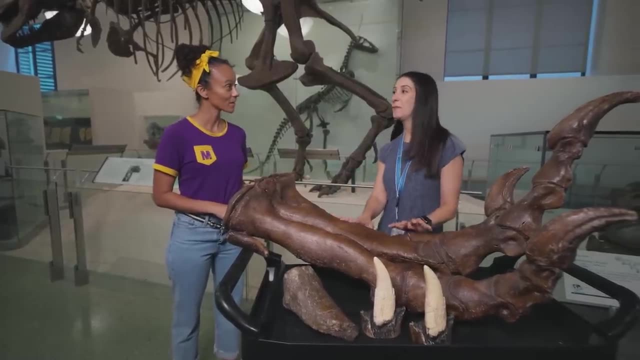 Well, I'm really excited because my favorite dinosaur is the T-Rex. I really like the T-Rex also. Oh yeah, What's one of the reasons you love the T-Rex? I like the T-Rex because it was one of the biggest predators. 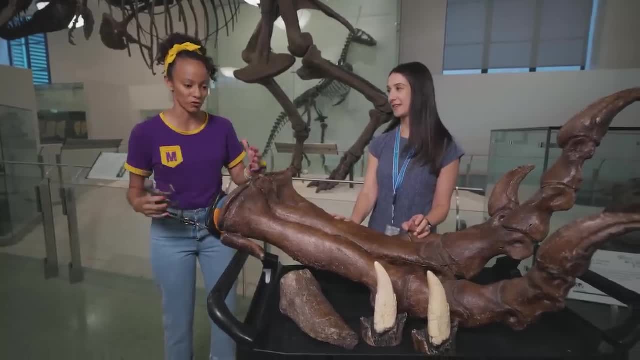 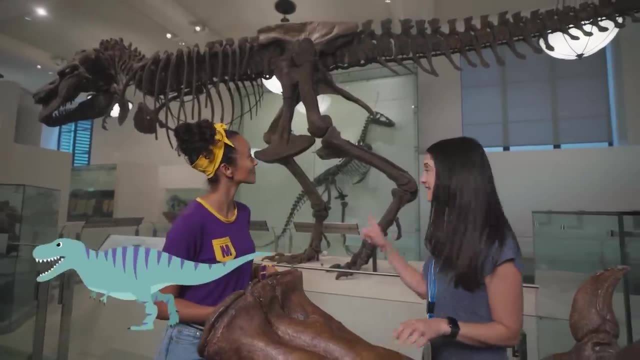 Oh, I know It's very cool. The T-Rex is huge, has a really big head and legs and a really big tail. You know they use that big tail to help them balance. Oh yeah, that's right. 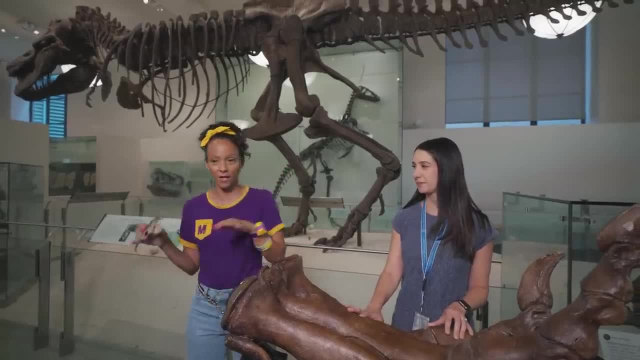 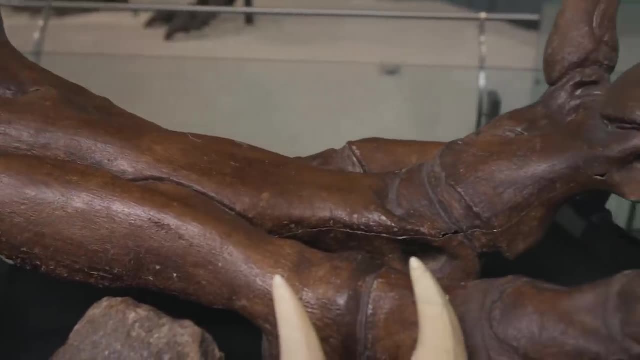 because their heads are really heavy, right, Really big heads, Yeah, so the tail helps them balance like that. You know what else I like about the T-Rex? What? Look at this big foot here. Whoa, is this a real foot of a T-Rex? 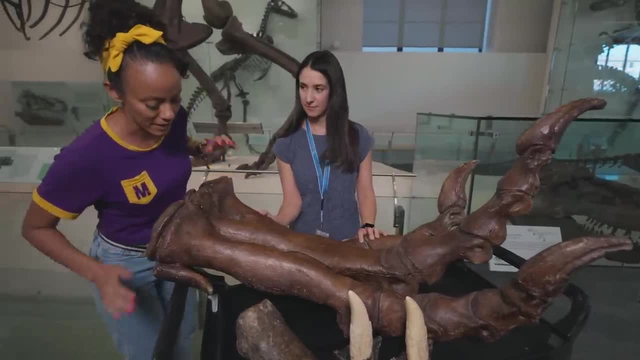 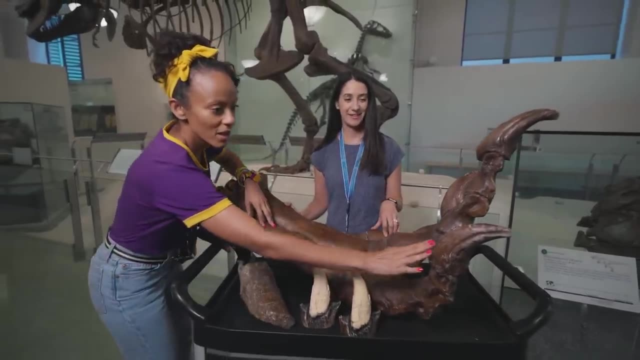 This is a model, Okay, okay, But this is like an exact replica. Yeah, you can see how big it was. Whoa, am I allowed to touch it? You can touch it, Okay. Look at these toenails. They're so big and pointy. 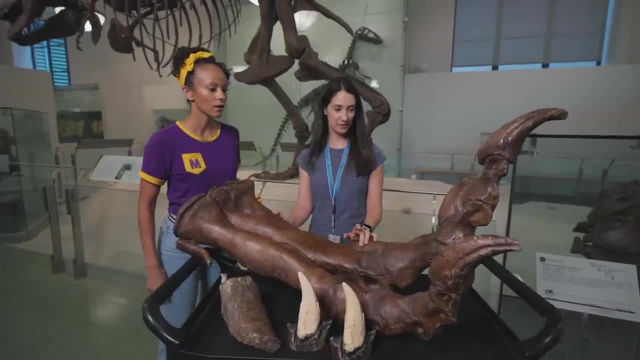 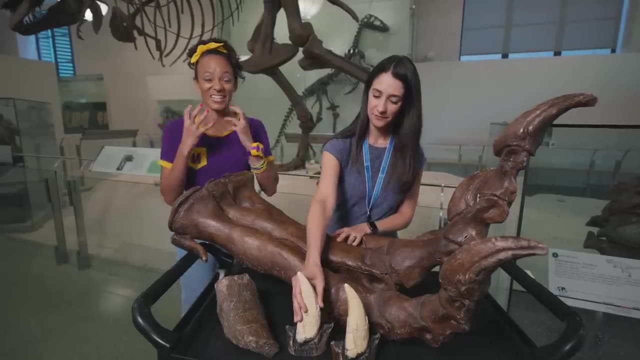 So they had three big toes on their back foot. You know what else I like about the T-Rex? What, How big their teeth were. Oh yeah, they have really big teeth. Look at this Whoa. look how big this tooth is. 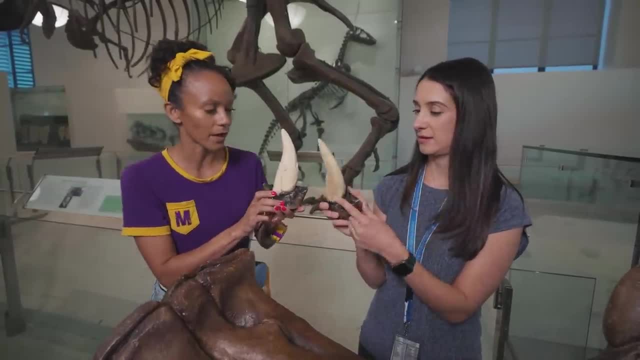 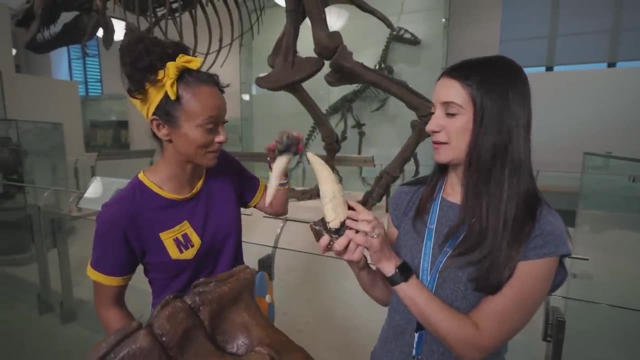 This is a model of a real T-Rex tooth. Wow, can you imagine if your teeth were this big? Look, is it this thing? That's really big. What do you think they might have liked to eat with a tooth this big? 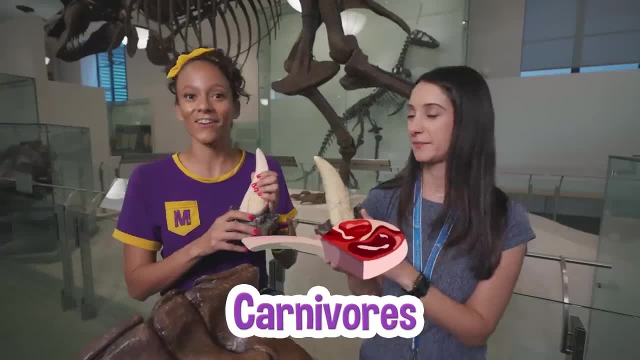 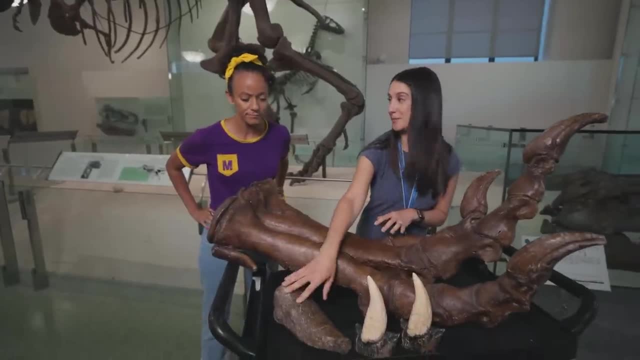 Oh, probably meat, right, Yeah, they were carnivores. Oh, so they were meat eaters. cool, And what's this? It looks like a big rock. It is a rock, except it's a very special rock, Oh, why. 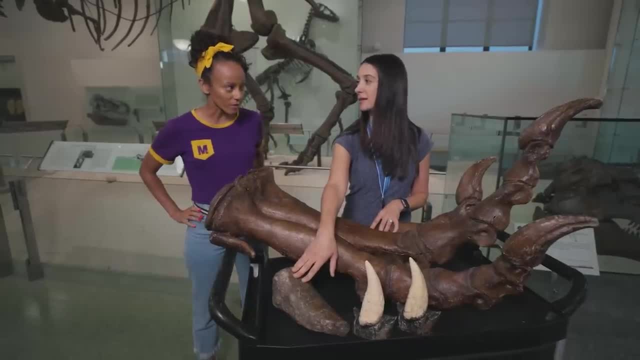 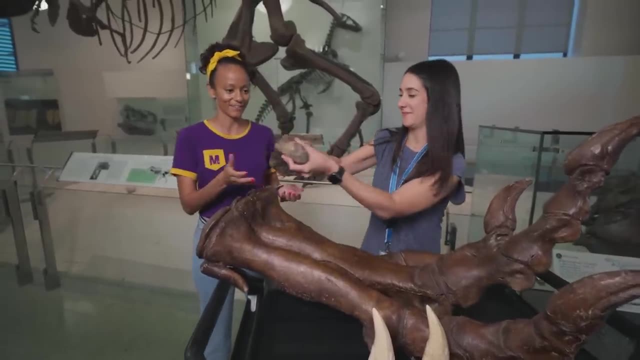 This is a fossil of a dinosaur bone, A real dinosaur bone, A real dinosaur bone. Would you like to touch it? Yes, please, It's heavy. Okay, Whoa, let's see. Let's see. Okay, all right, it's a little heavy. 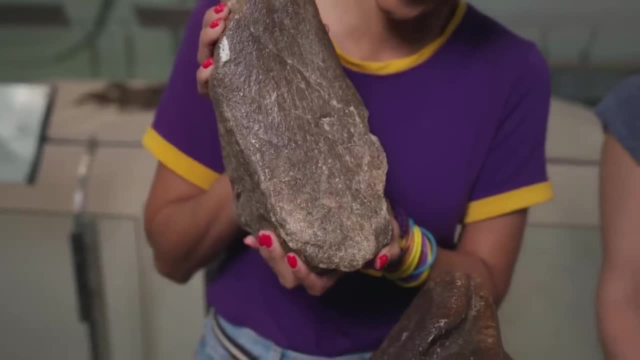 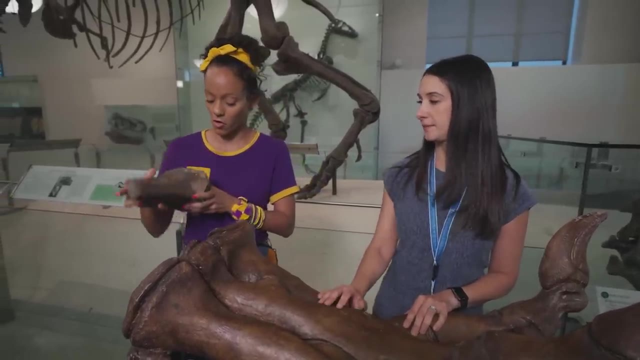 but it's a real fossil of a dinosaur bone. That's amazing. And what part of the dinosaur is this That was from their leg or their thigh bone? Oh, so like down here Right there? Wow, that's amazing. Thanks for sharing this with me. 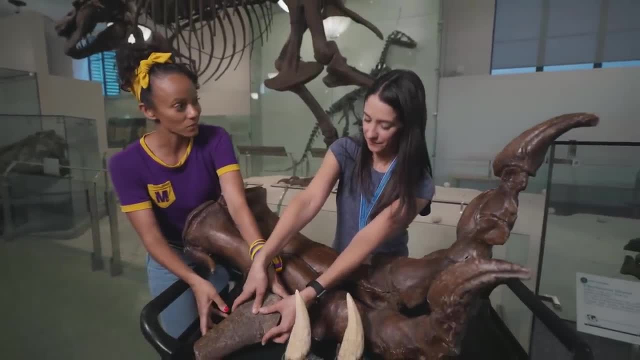 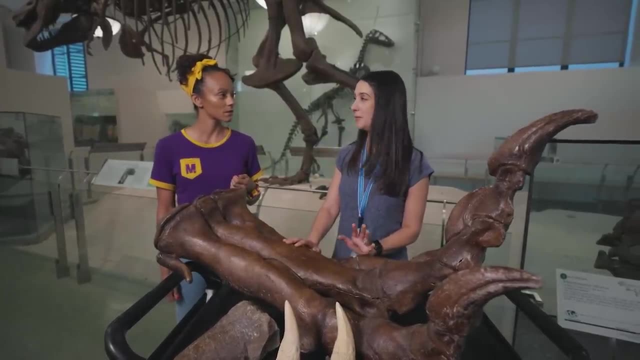 Yeah, So is the T-Rex the biggest dinosaur. It wasn't the biggest dinosaur, but this museum has a model, A model of one of the biggest dinosaurs. What Can we see it? You want to go see it, Yeah. 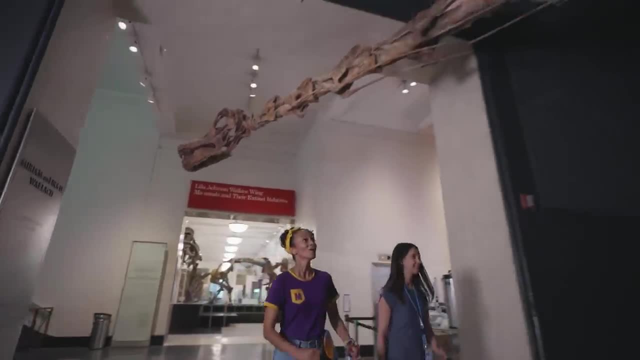 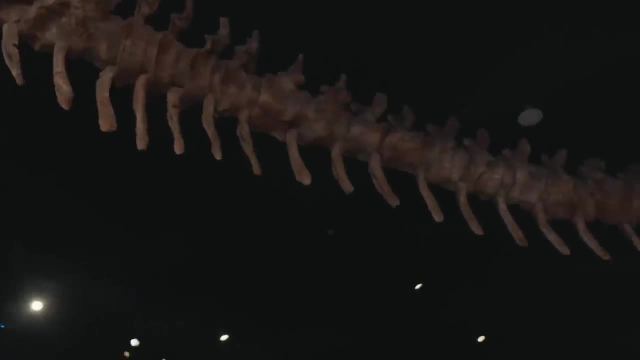 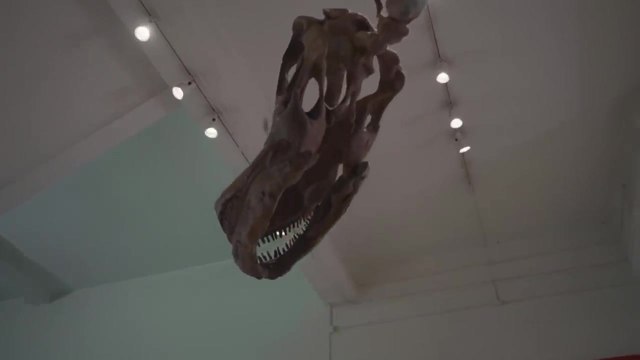 Let's go. All right, come on. Wow, Whoa, it's so big, Whoa, it keeps going and going and going. This is called a titanosaur- Titanosaur- wow, it's really cool. So the titanosaur family was a group of dinosaurs. 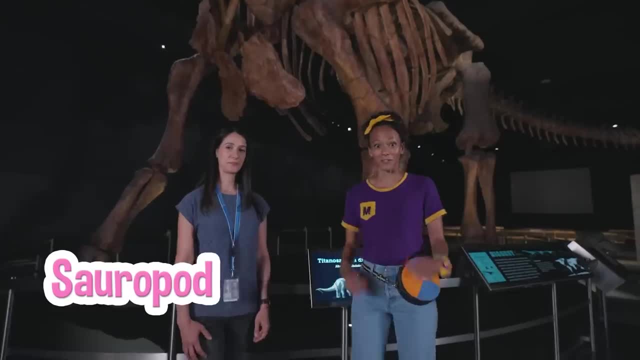 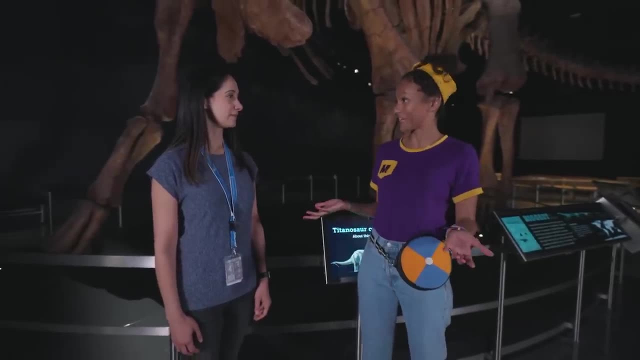 that were sauropods And herbivores. Oh, I know what a sauropod is. That means it walked on four feet, That's right, Whoa. And an herbivore means that it was a plant eater, That's right. 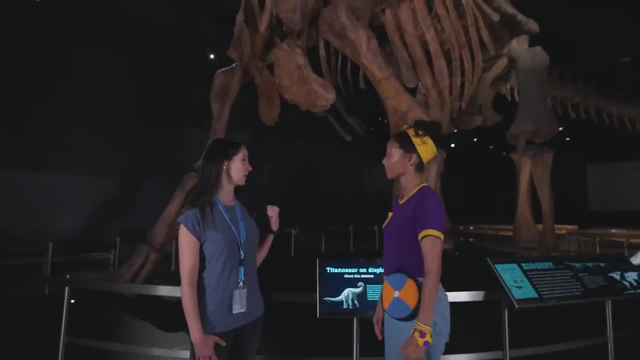 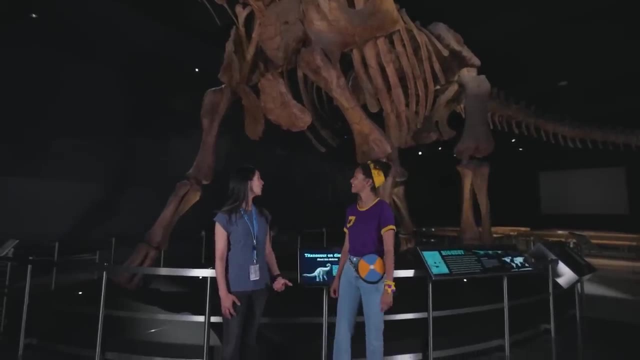 Yeah, very neat. Now, this titanosaur is over 120 feet long. Whoa, or 37 meters. That's really long, And it weighed almost as much as 10 elephants. Whoa, 10 elephants, that's very, very heavy. 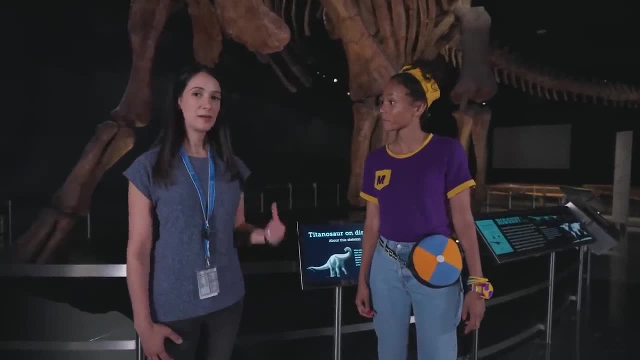 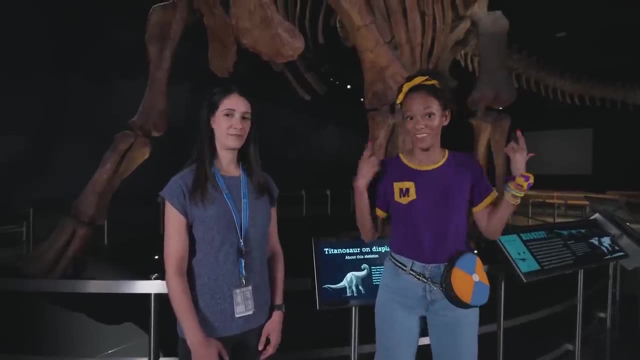 Wow. But you know what's cool about this? This one, This one, was just a juvenile, which means it's kind of like a teenager Whoa, so it's not even fully grown. It gets bigger than this. It does. 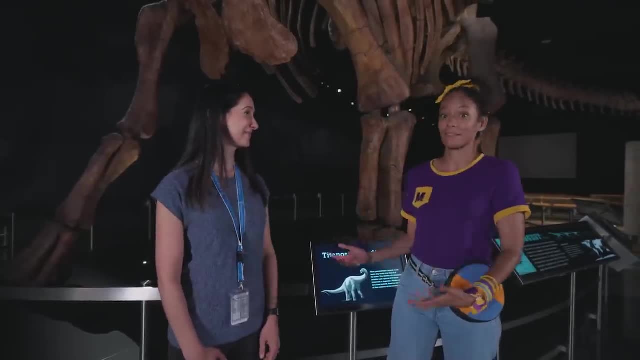 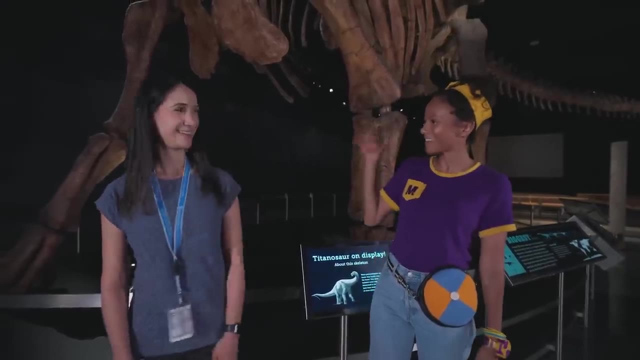 Wow, that's incredible. Thank you so much for showing me this titanosaur. I had fun with you. I have to go teach a class, Oh, But I'll see you soon. Okay, see ya. Thanks again. Wow, what a fun day. 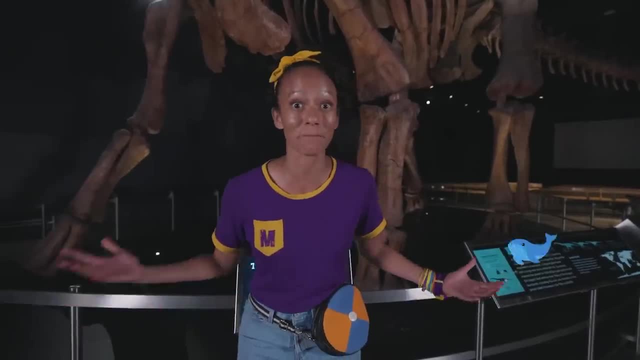 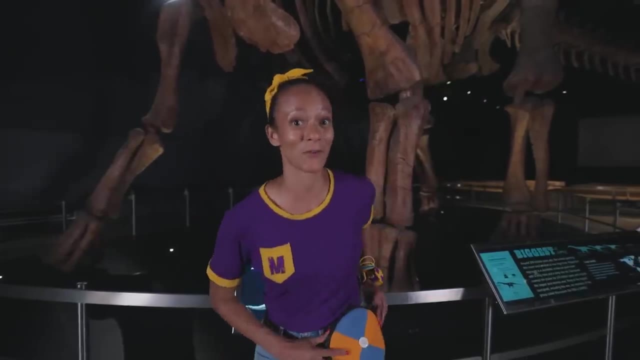 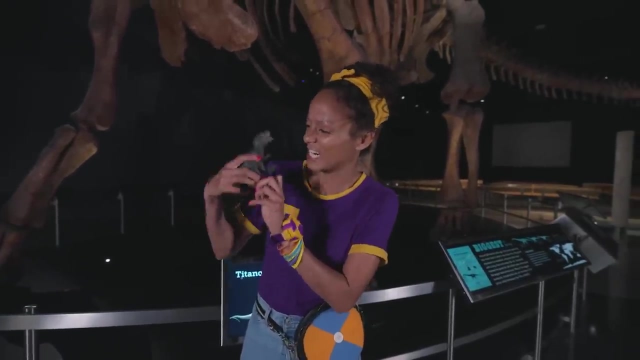 We got to see so many cool animals like that big blue whale and walruses, Oh, And lions, and we got to see my favorite dinosaur of all time, the T-rex. Did you have a fun day Me too? Well, this is the end of this video. 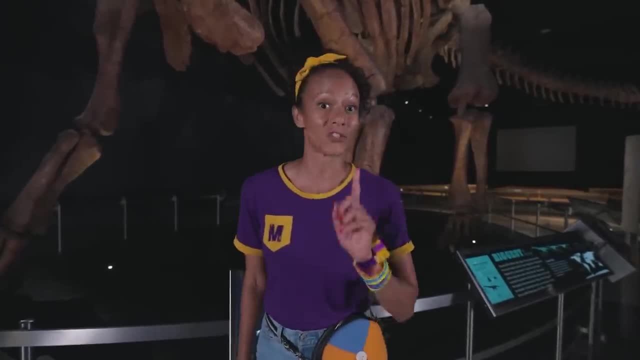 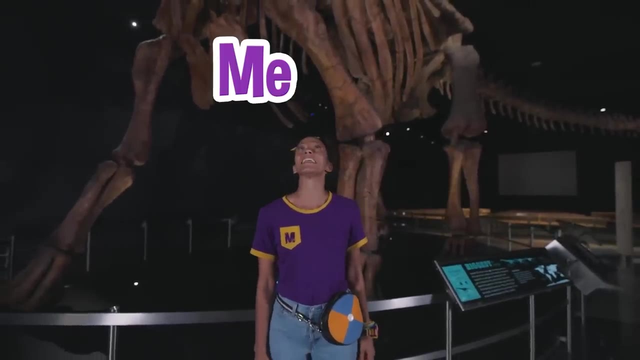 But if you want to have more fun and see more of my videos, all you have to do is search for my name. Will you spell my name with me? Cool, M-E-E-K-O, A-H. Mika. All right, we'll see you next time. 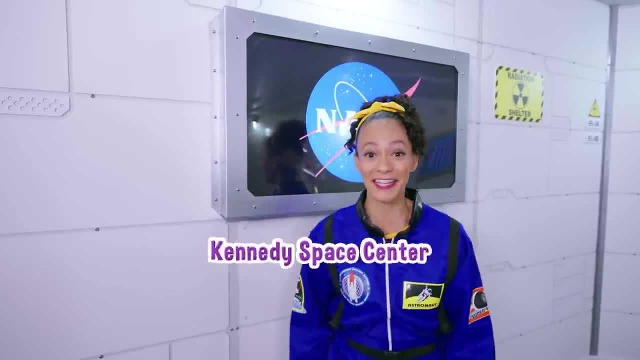 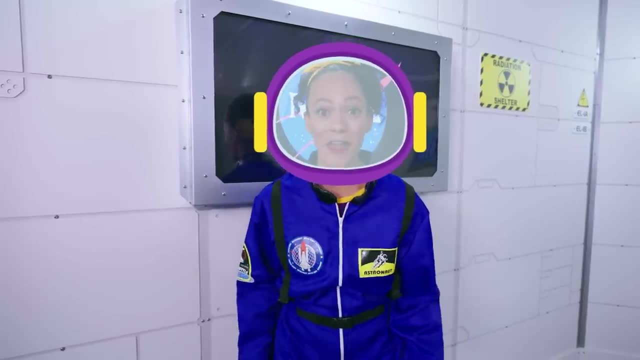 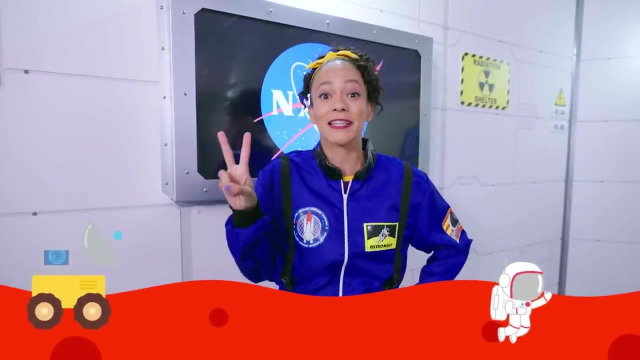 Hey, it's me Mika, And today I'm at the Kennedy Space Center in Merritt Island, Florida. Look, I'm even wearing a space suit because I'm going on a very special space mission. My plan is to experience a spacewalk experience landing. 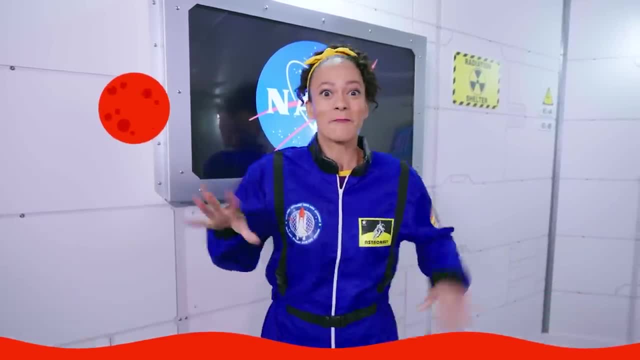 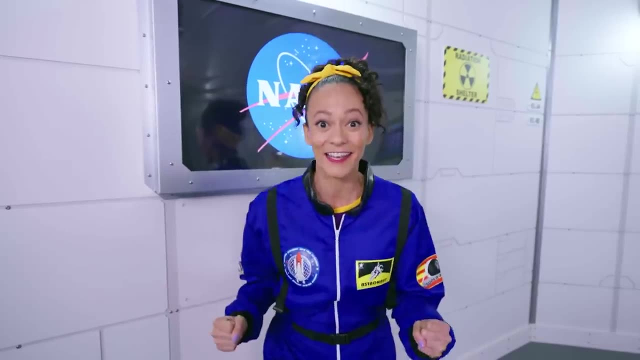 and driving on Mars And going to Mars space, but it's all simulation style, which means I'm not really going to space. But if you're going to feel like it, will you come with me, Let's go. Hey, Hi. 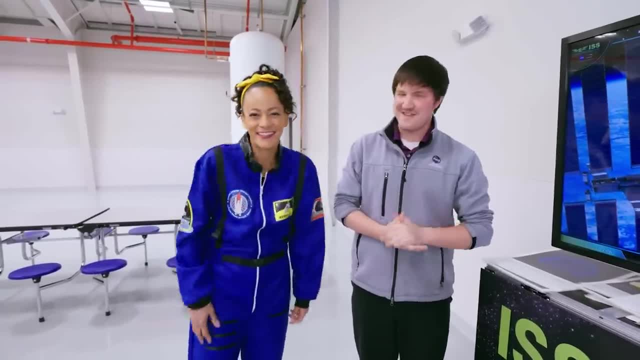 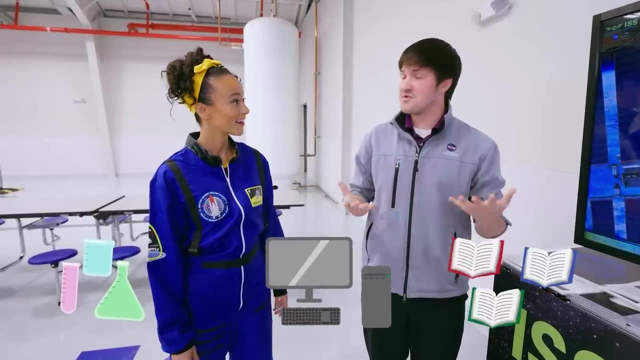 Who are you? I'm Daniel. Oh, hi, Daniel, I'm Mika Hi. So what do you do here? I'm an educator here at Kennedy Space Center, So I teach kids all about science, technology, history- a lot of really cool topics. 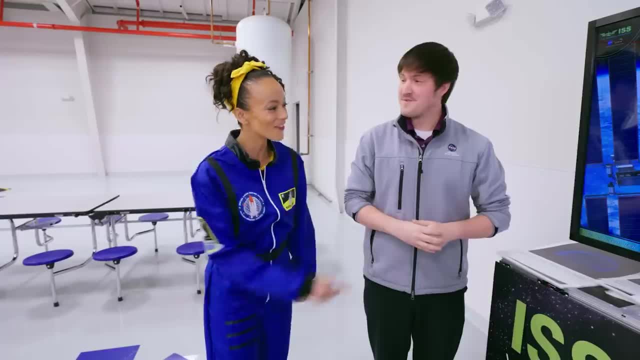 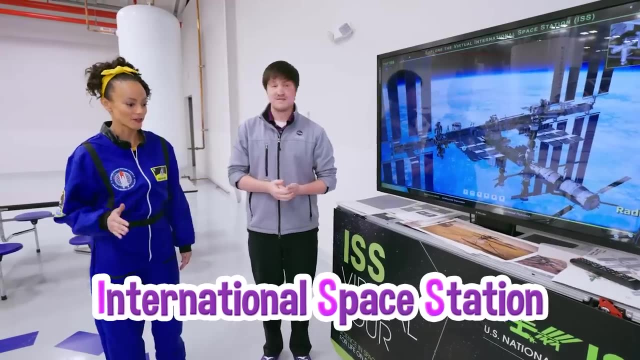 Wow, you must know a lot. Yeah Well, what is this? This is actually a 3D model of the International Space Station, the ISS. ISS- OK, so that stands for International Space Station Station. You got it. 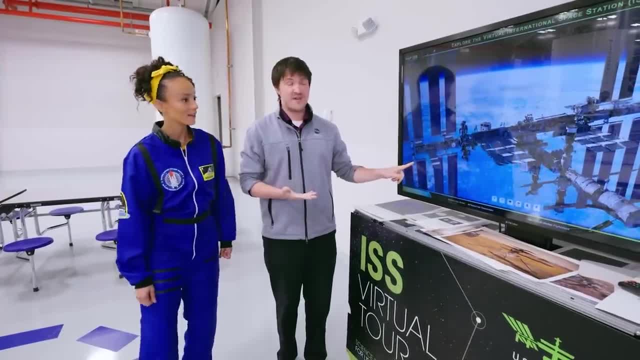 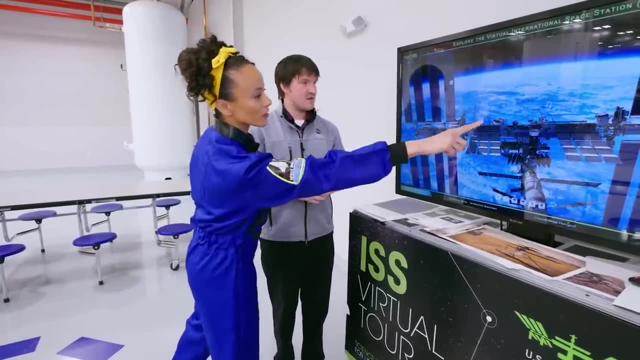 ISS, Cool, Oh yeah, Now it's really really big. It's about as big as a football field. Whoa, that is really really big. Yeah, And what's this long part in the middle here? So the long part in the middle is called the truss segment. 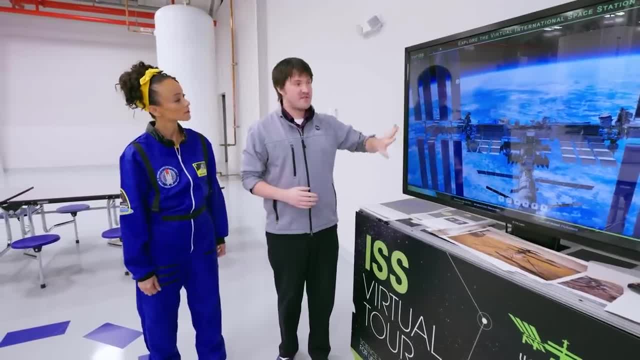 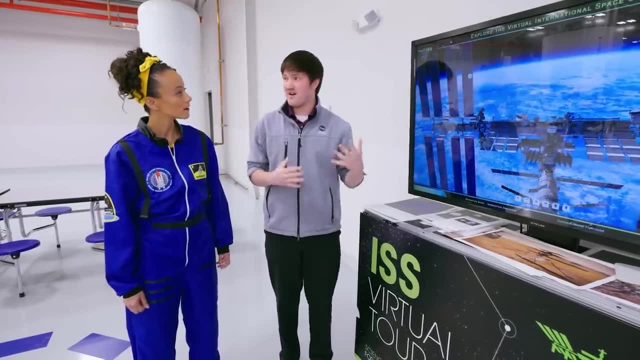 Oh, the truss. OK, and what does that do? So that holds the things like the solar panels, a lot of cool instruments and experiments. The astronauts usually just live in the middle. They don't usually go out there all that often. 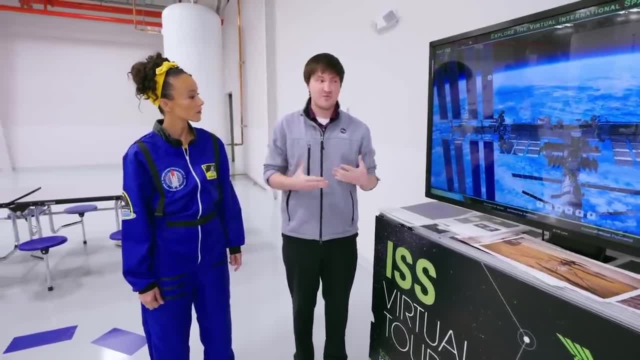 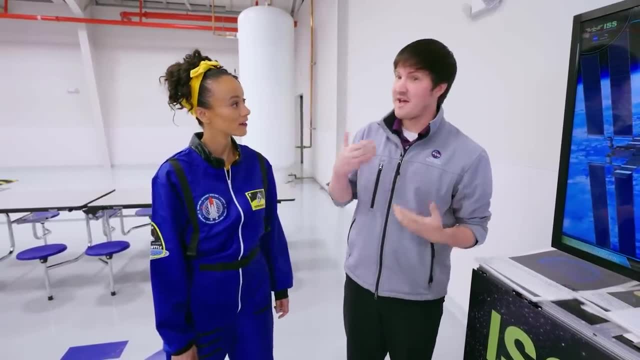 Why would they need to go out there? Well, sometimes you got to repair stuff or replace things. Oh, that's cool. Yeah, Now something we also have that's really, really cool. here is a simulator that'll kind of show you how astronauts 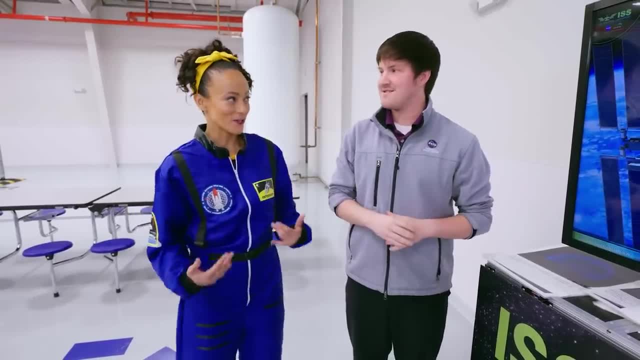 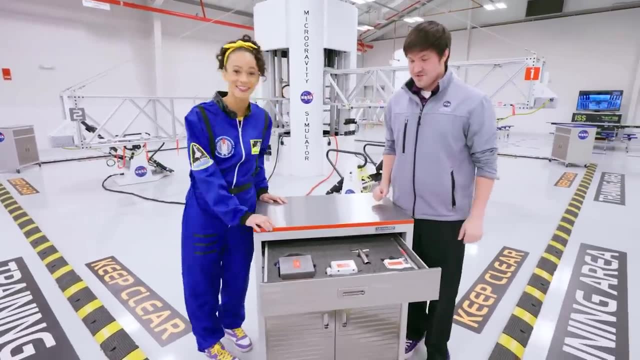 actually train to go out there Really? Yeah, Could I try Totally. Oh, let's do it. Whoa, Daniel, What's all this? So these are all our tools and equipment and replacement parts that we're going to use in our simulator. 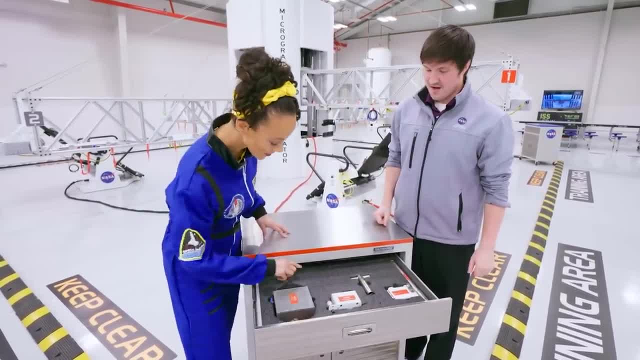 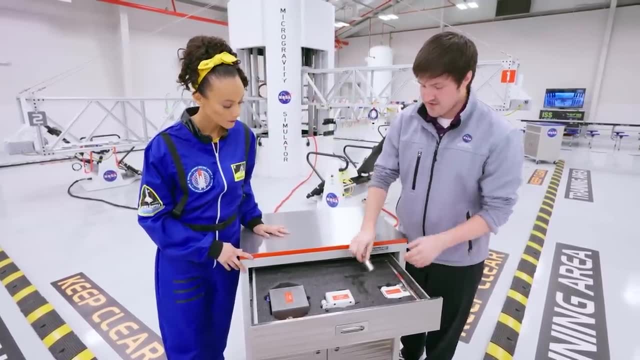 Wow, that's going to be awesome. Oh yeah, What's all in here? So there's tons of different things. We have different wrenches and different equipment. One that's very important that you're going to use today is this one right here. 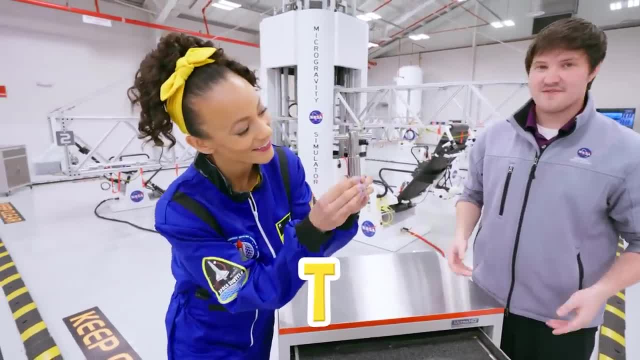 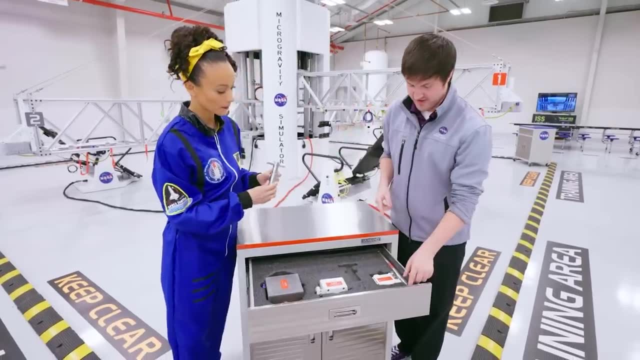 Oh, hey, it looks like the letter T. Yeah, that's actually where it gets its name. It's called the T-handle wrench. Oh, makes sense, T-handle wrench. OK, We actually have a bigger version of that. It's this one right here. 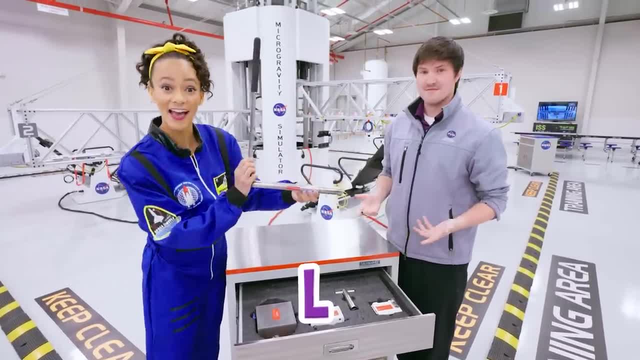 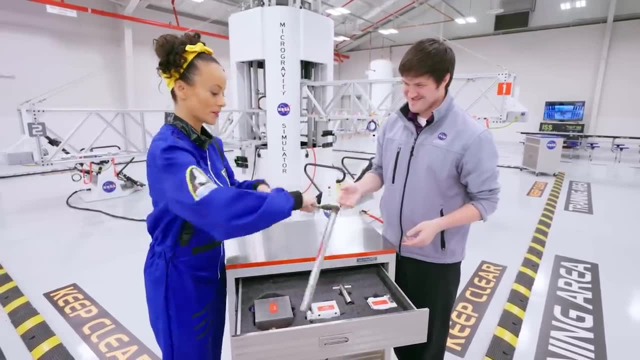 Whoa, and look at this, It looks like the letter L, And that's what its name is: L-handle wrench. Oh, L-handle wrench Works out Easy to remember. Oh, yeah, This way, There you go. 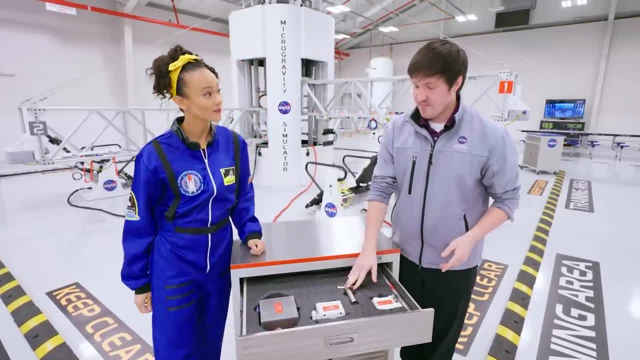 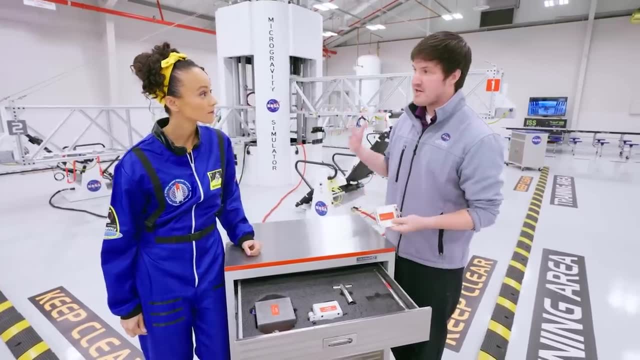 You got it OK. Now we're just going to use this little one today, But we have other things that we can use to replace stuff. We have something right here called a dust environment. This one is to try to capture micrometeorites and particles. 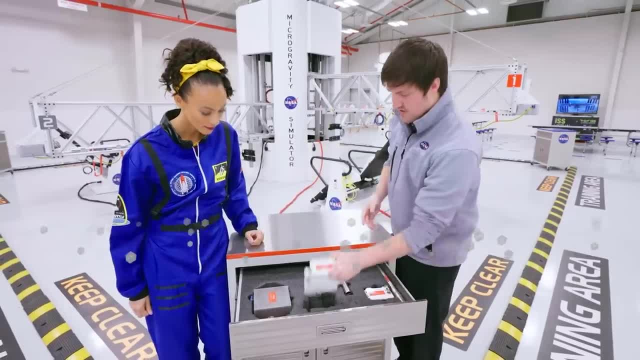 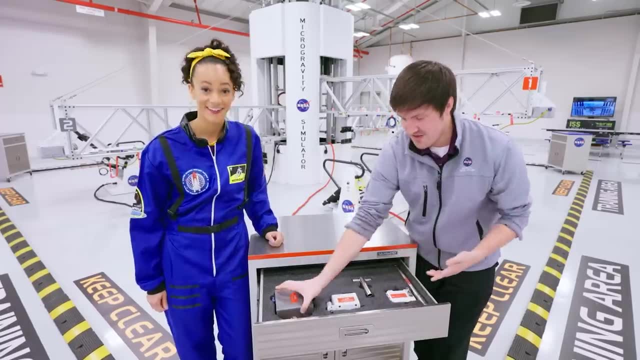 in space and dust and debris. Wow, We have this little one right here. It's an electronics module. It's for computers and stuff like that. Looks complicated, Yeah, But I'm going to give you an easy one to deal with. 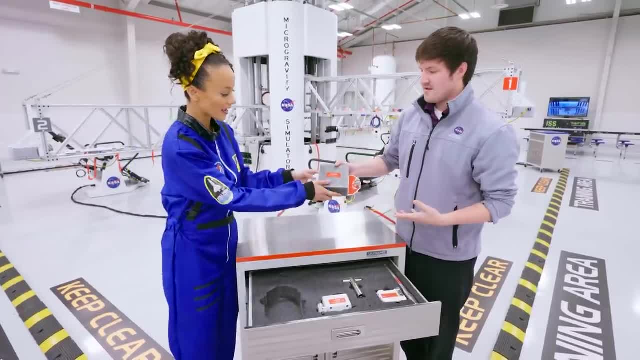 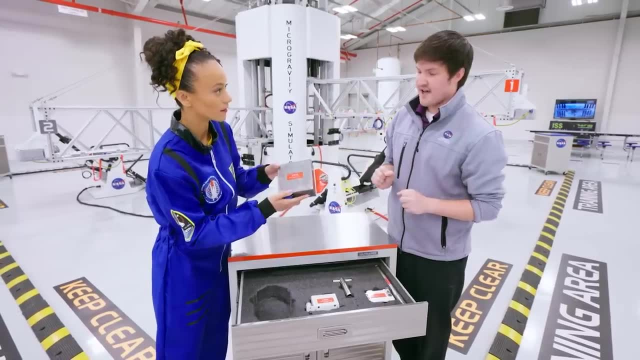 It's called a vibration detection system. Whoa, what does that do? Careful, It's very heavy, OK. OK, So that detects if the station shakes or shimmies or anything kind of crazy like that, And that would be bad. 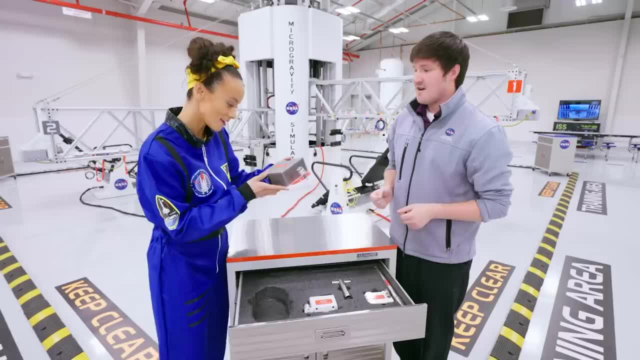 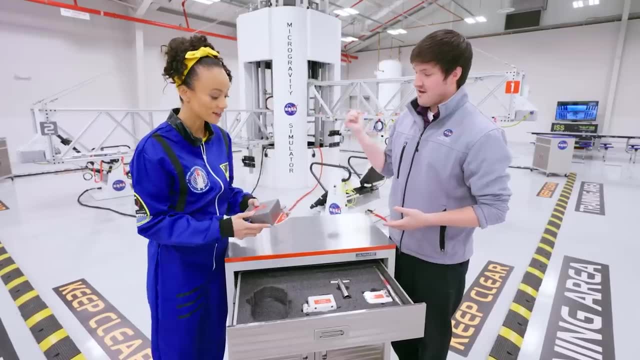 Yes, OK, It would be very bad. OK, So this is super important. Yes, OK, So what's going to happen is that when I put you in the chair- OK, we're going to find that on the truss. 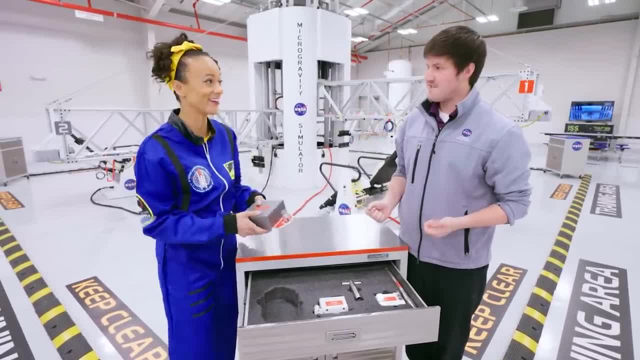 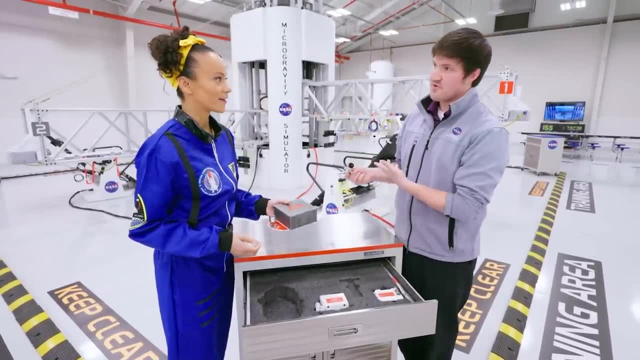 And then you're going to replace it. Wow, Cool. Yeah, I can't wait And I'm going to give you this little one to replace it. We can test it right now so you get a little better understanding before we go. 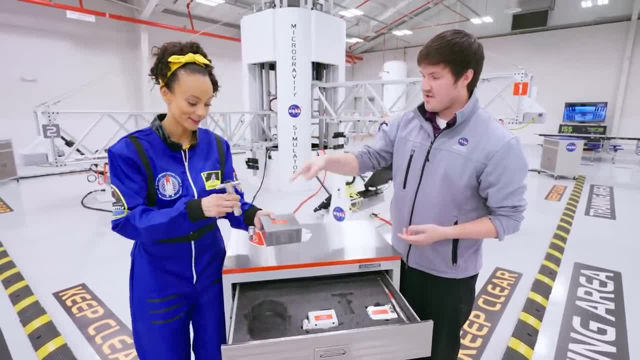 OK, Let's test it out. So you're going to grab onto that Uh-huh. Now, when you put it inside, it's kind of like a screwdriver: You put it in and push it straight down. There you go. 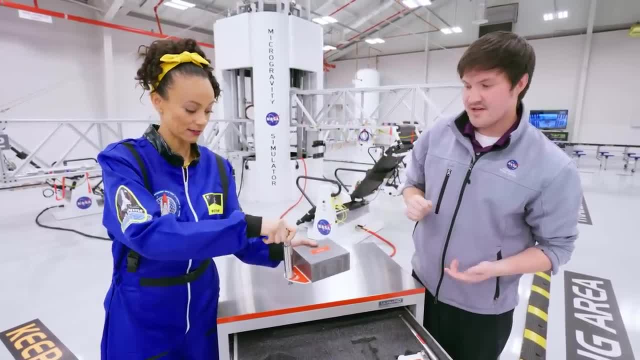 And then you're going to turn it halfway, Halfway, like that: Yep, There you go. Now, when you do that, it's going to come out and it's going to fall down. OK, good to know. So make sure not to let it fall. 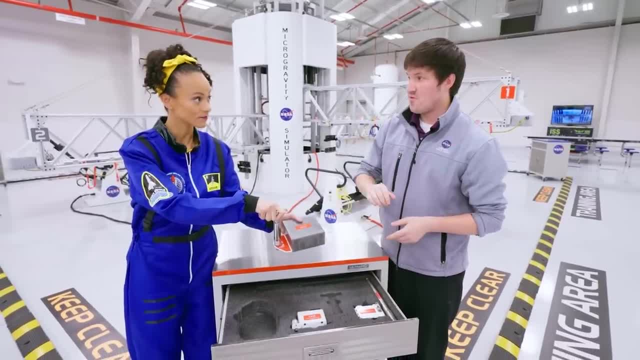 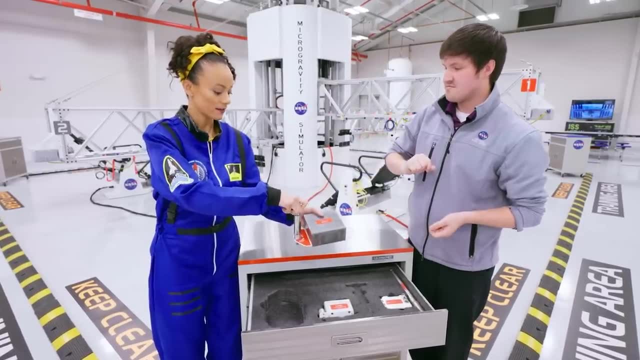 OK, OK. Then I'm going to give you the new one, You're going to give me the old one, OK, OK. And then, when you put the new one in, you're going to do the same thing. You're going to push and half turn. 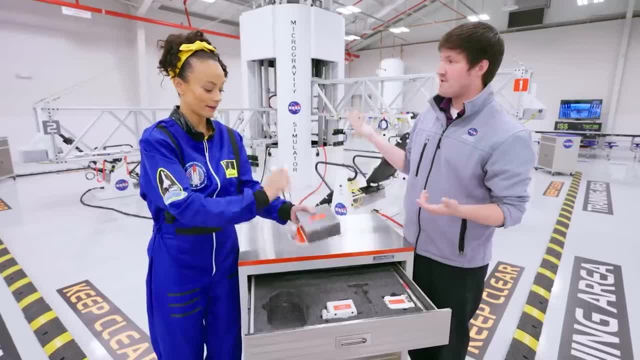 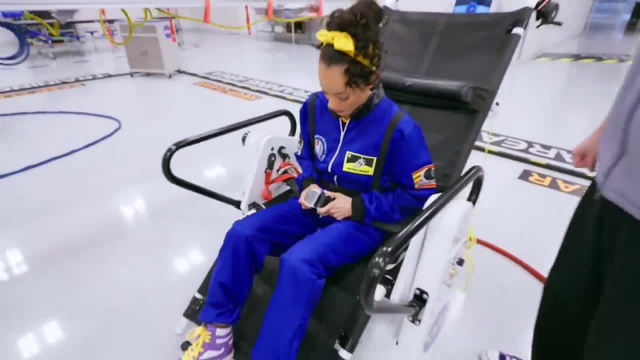 The other way, Yep, And then that new one will be in place And you've replaced something. Oh, awesome Works out. OK, well, let's do it. Yeah, All right. buckling in The seat belt is very much like the one. 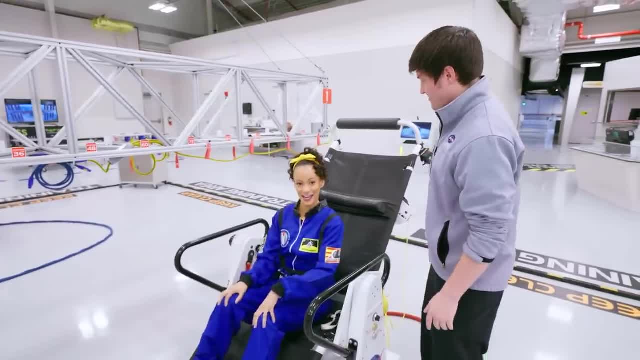 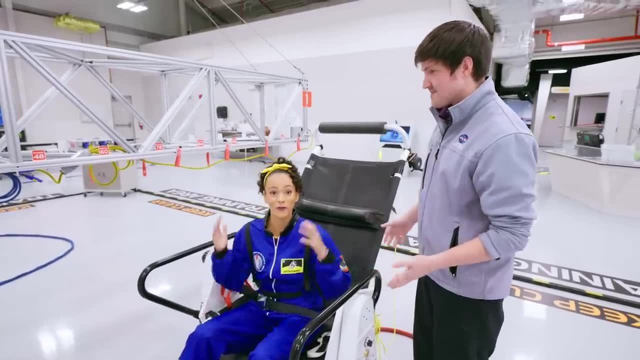 you would use on an airplane. Yeah, exactly, OK, nice and tight. Now you're in our microgravity. This is what we're going to use to kind of simulate our spacewalk. Yeah, that's right, Microgravity. 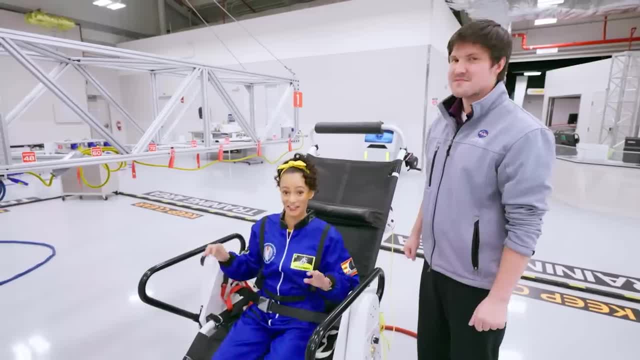 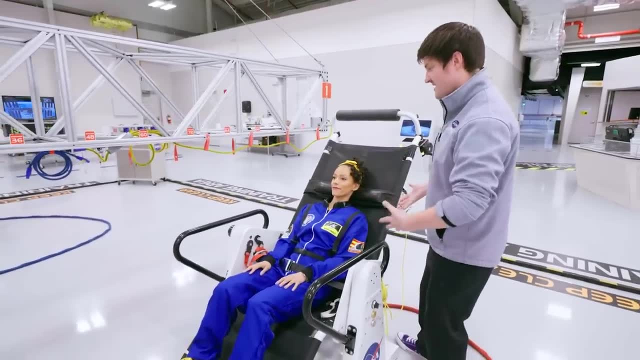 And for a spacewalk you use your hands, not your feet. Yeah, OK, Now I want you to have your head all the way back against, like that little pillow. OK, I'm going to rock you back. It's going to feel like being in a dentist chair. 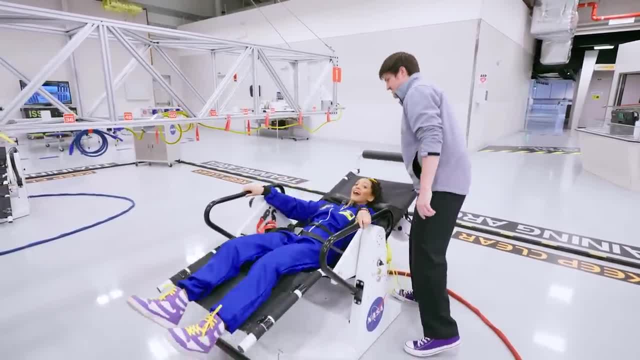 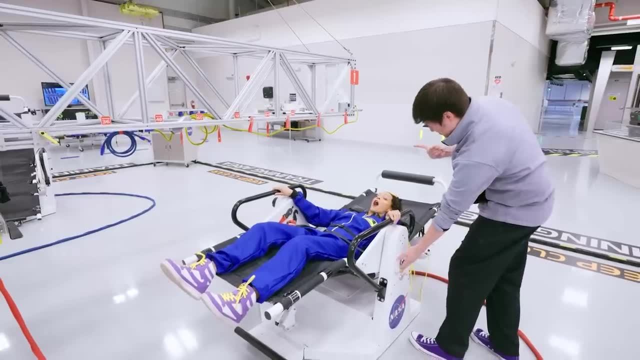 Oh, OK, So rocking you back, OK, All right, Feel OK. Yeah, nice, and cozy You ready. Yeah, OK, starting in three, two, one. Now it's really loud. Oh yeah, it's a little loud. 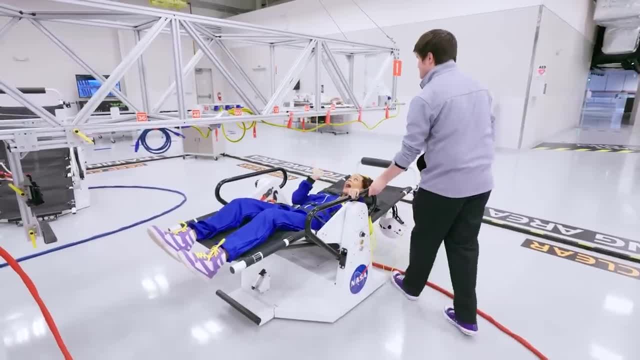 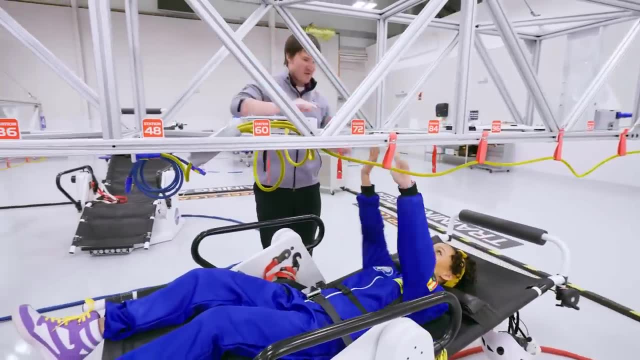 Yeah, Now I'm going to push you underneath. Whoa, OK, Now you can reach your arms up. OK, OK, And I want you to catch the truss There. so you got it. Got it. Now you can try moving up and down. 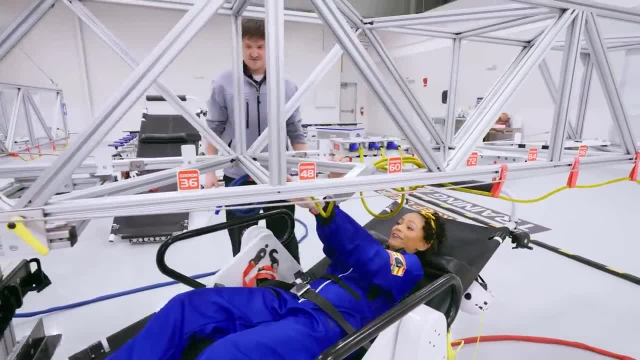 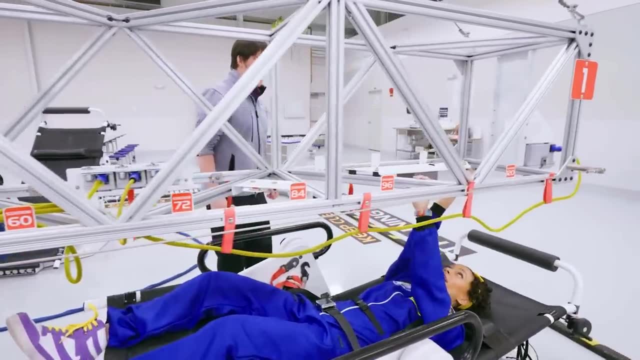 OK, Just use your arms, though Remember no feet. Woo, Yep, So you're at the bottom. Now try moving all the way up to the top. Notice how easy it is to move. Yeah, Yeah, It's really fun. 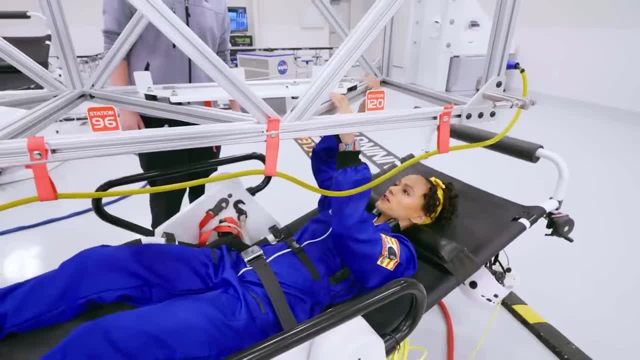 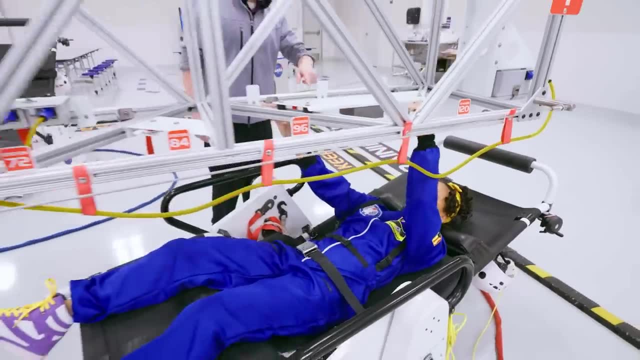 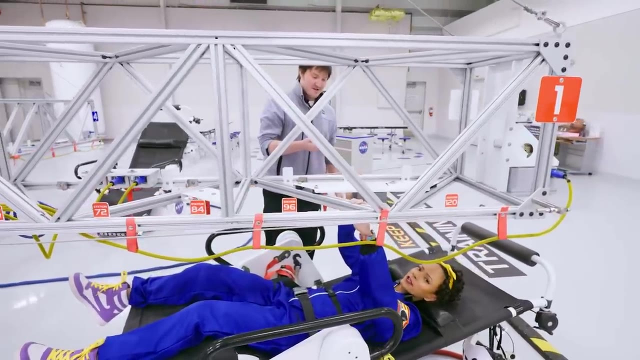 Yeah, Cool, And it feels like I'm floating, Wow, Wow. So I want you to come right here to station 108.. 108. Because we got a job to do, not just having fun. OK Yeah, Here it is 108,. ready for my job? 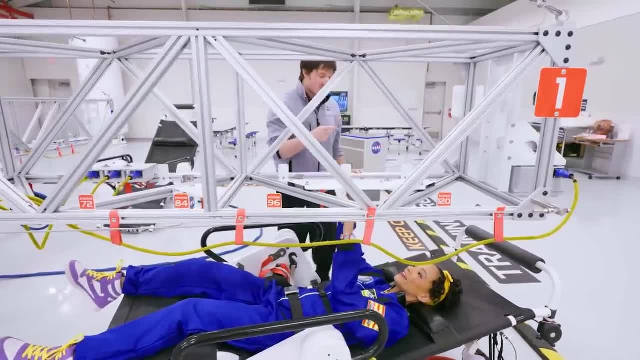 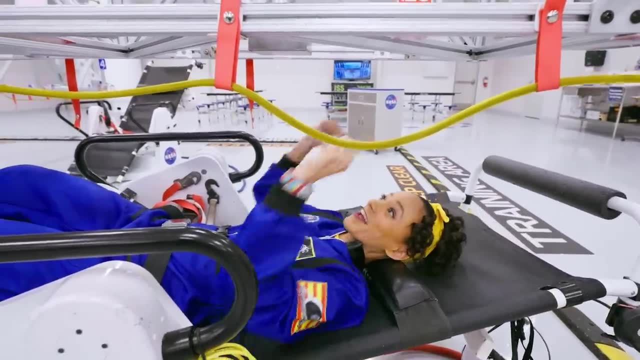 Yeah, So we're going to replace this instrument right here, OK, OK. So I'm going to give you some tools, remember? This is awesome. I'm working on the truss Like a real astronaut. So do you see the old vibration unit in front of you? 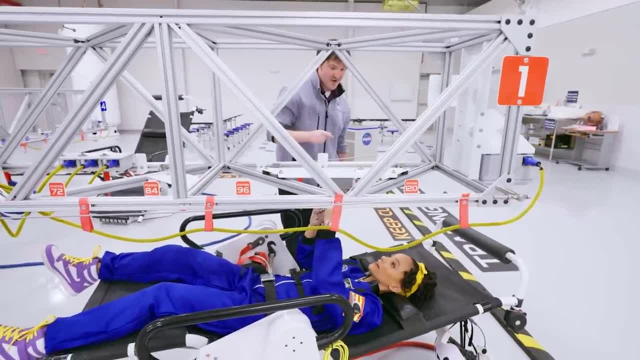 Yep, I'm going to give you the T-handle wrench, OK, And you're going to take it out. Remember, don't let it fall on you, All right, OK, So push up. Yeah, this needs to be replaced. 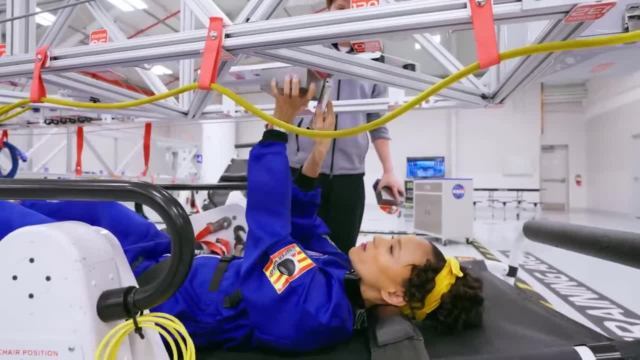 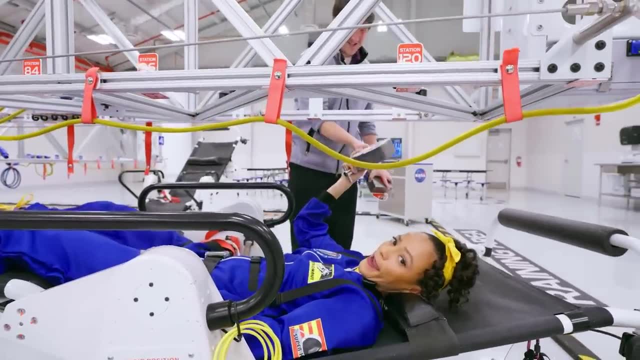 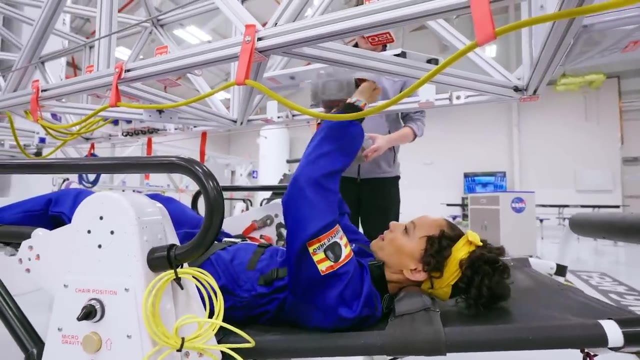 Good thing I'm here. I am very good at replacing these old things. There you go. Old ones out. I'll take the old one. Here's the new one. OK, OK, Whoop, And turn it around. You got it. 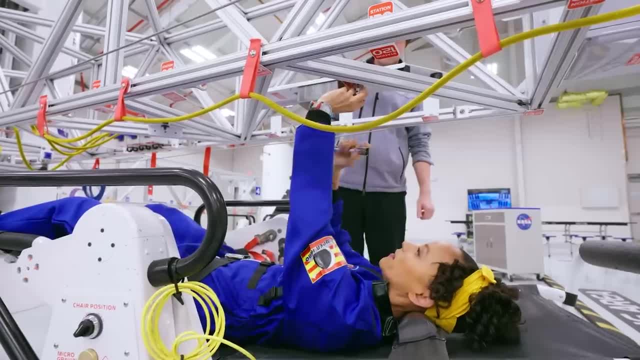 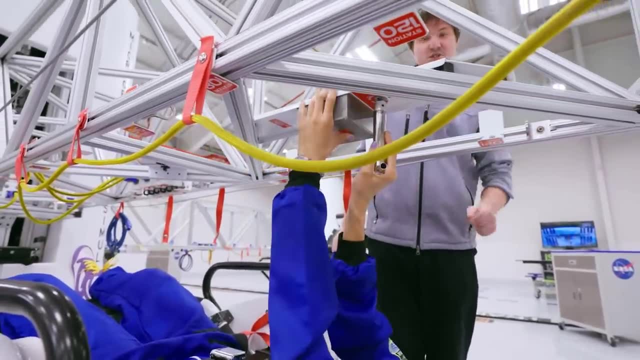 OK, That goes there. Yep, OK, Goes there, Push it in, Push it straight up, Turn your handle, wrench a little tiny bit more to the right. OK, A little bit more. OK, There you go. Now he's talking. 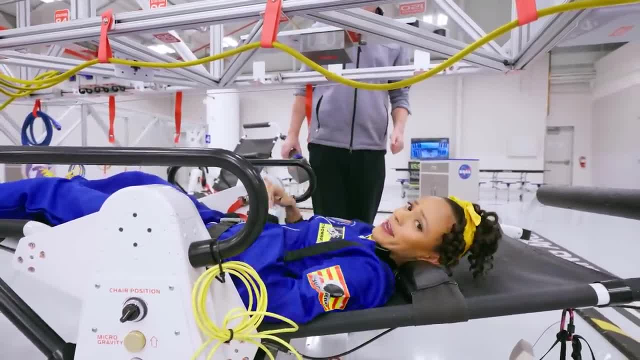 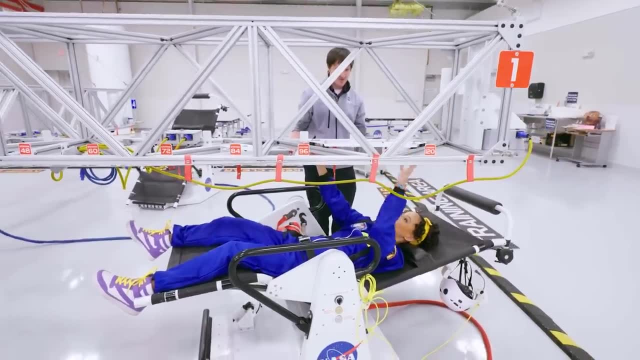 And then let go And you're all good. All right there, buddy, That one's good to go. Perfect, I'll take the wrench back. All right, OK, But hey, we finished our job. Awesome, Good job. 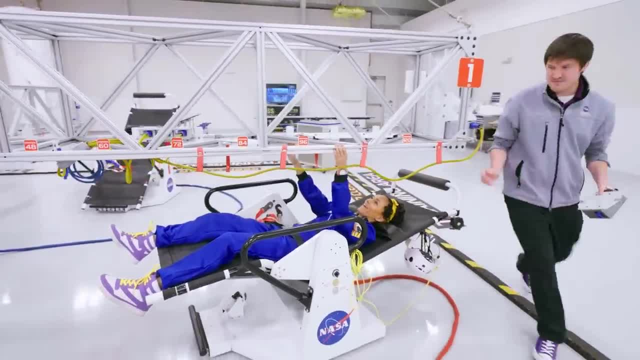 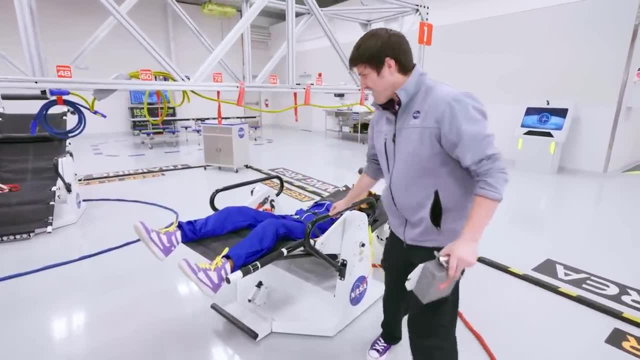 I'm going to get you out of the chair, OK, OK, So stay right there, You can let go. OK, You're floating away from the station, Oh no, Bye. Wow, I could take a nap in this chair. 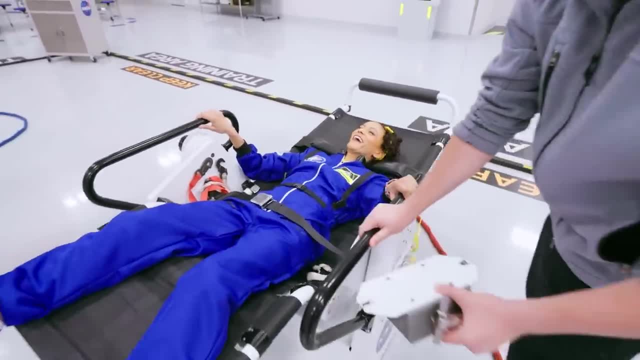 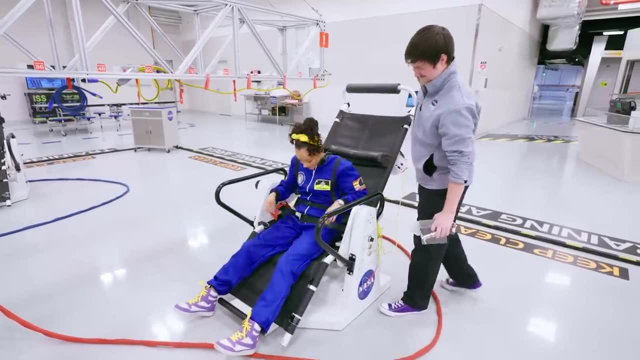 Well, you can, now that you've done your job, OK, But bringing you back down to Earth, Three, two, one, Welcome back. That was a quick ride. Oh yeah, Hello Earth. OK, And there you go. 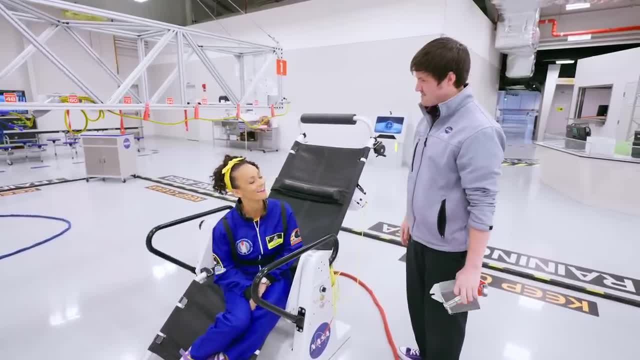 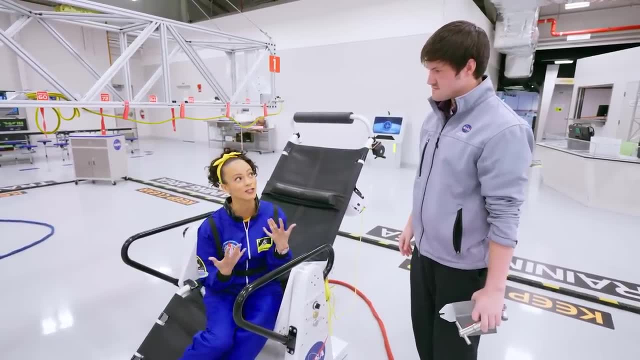 Thank you so much for letting me experience that. Yeah, No problem, That was really cool. So I got to feel what it would be like to do a spacewalk. Now I want to know what it feels like to travel to Mars, To Mars. 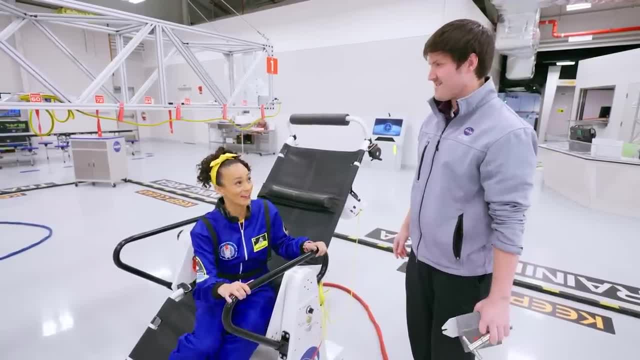 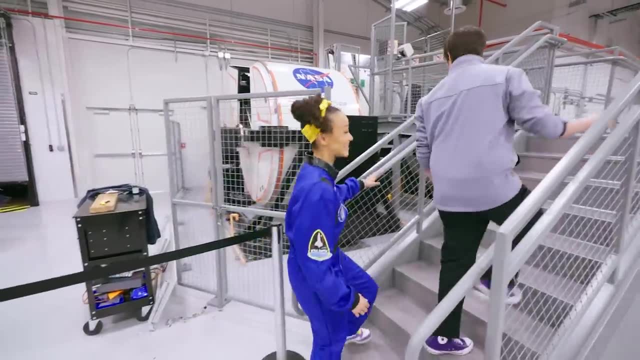 Do you have that here? We do Really, Yeah, Oh, can we do it Totally? Oh, let's go. Yeah, Come on, So come on over this way. Oh, I can't wait to see this, Oh yeah. 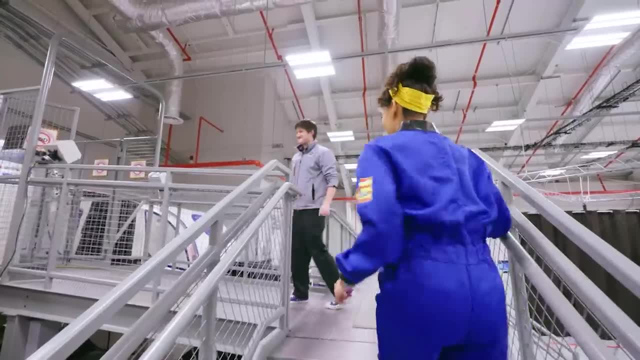 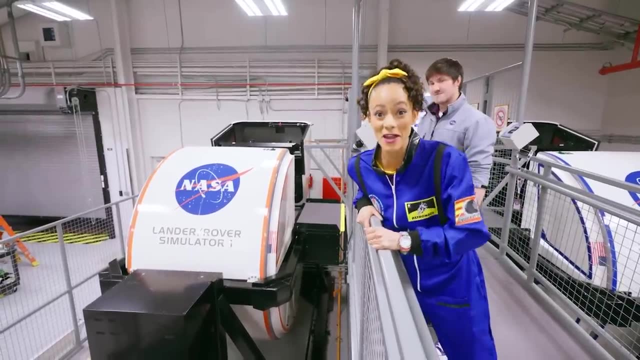 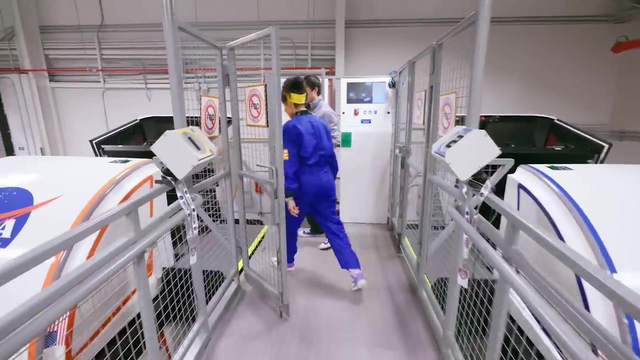 Come on, Whoa, Whoa. Look over there It says Lander Rover Simulator 1.. That's so cool, Yeah. So over here we have a really amazing simulator, Wow, OK. Yeah, This is going to show you how you're going to fly to Mars. 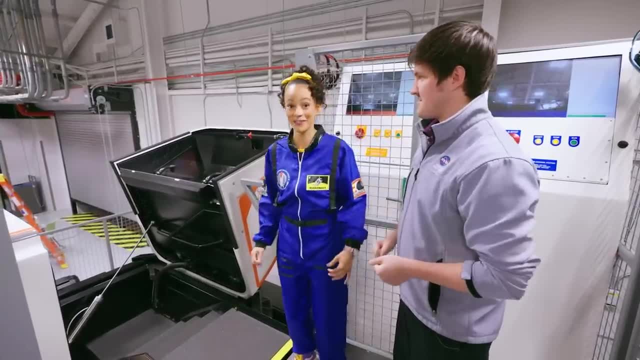 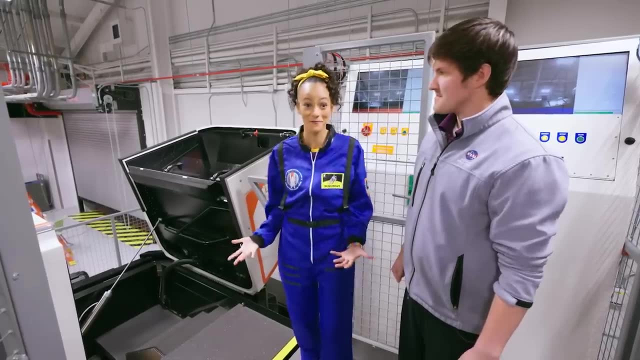 how you're going to land on Mars and then how you're going to drive on Mars. That's amazing And, remember, it's a simulation, so it's not real, But it's going to make me feel like I'm really traveling to Mars. 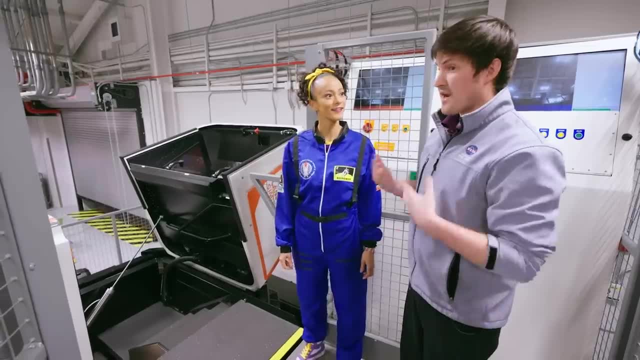 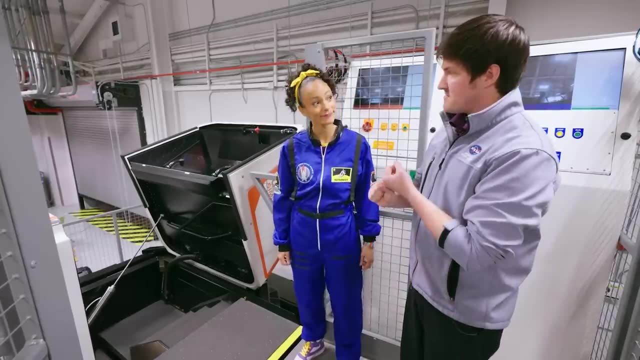 Yeah, Now we have two different positions. OK, Because whenever we do anything with NASA, we try to have a buddy system, Always have a backup. So two people, Yes, two people. So we have a commander who's going to fly the thing. 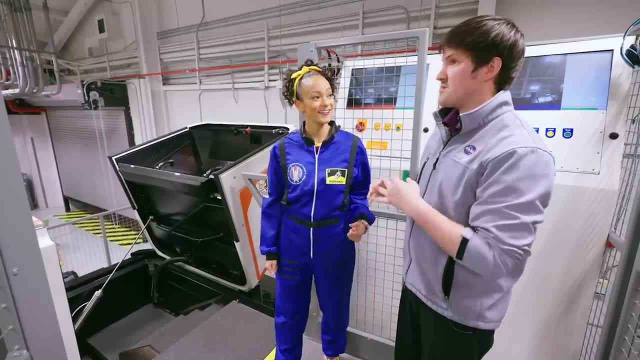 That's you, Yes, OK. And then we have a pilot who's going to drive it- In this case it's a robot. So you're OK, Wow, So you fly there, land and then you can drive. Yeah. 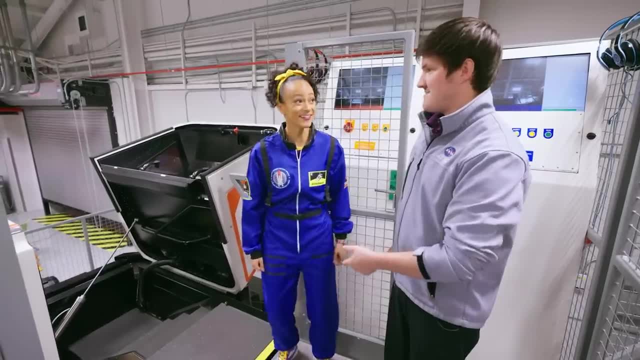 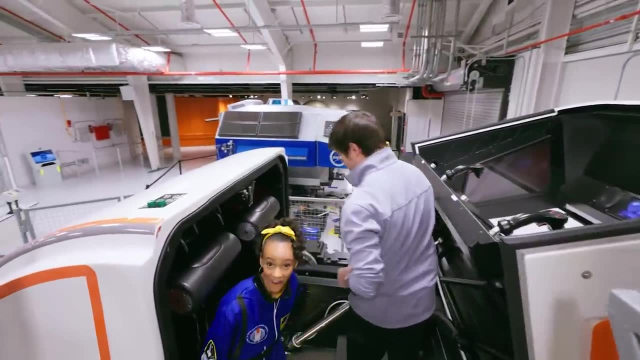 That's so cool, Right? Do you want to go inside? Yes, I do. OK, So head on down the stairs, OK, And then you're going to sit in this seat right here, OK? Whoa, There you go. 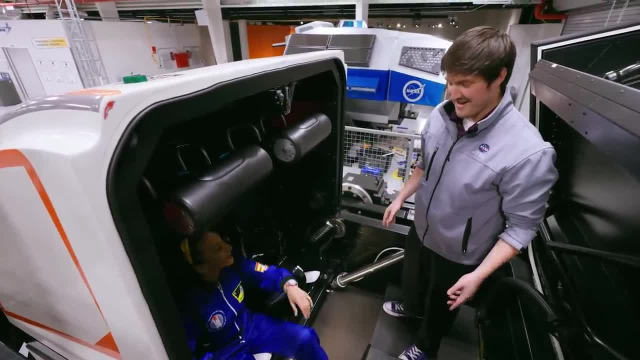 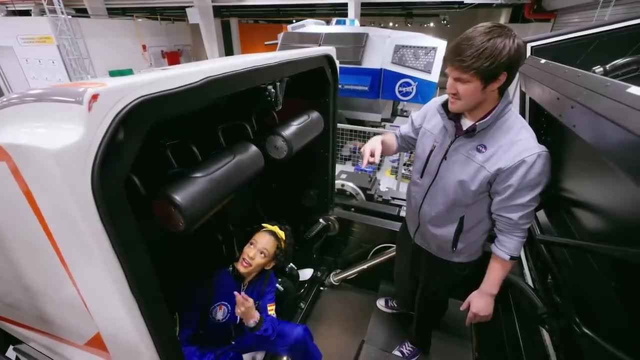 Whoa, It's cool, right, Yeah, Yeah, Now we're going to make sure you're as safe as possible. OK, So if you look up above, you'll probably notice something very similar. Oh yeah, It looks like a seat that you would sit in on a roller. 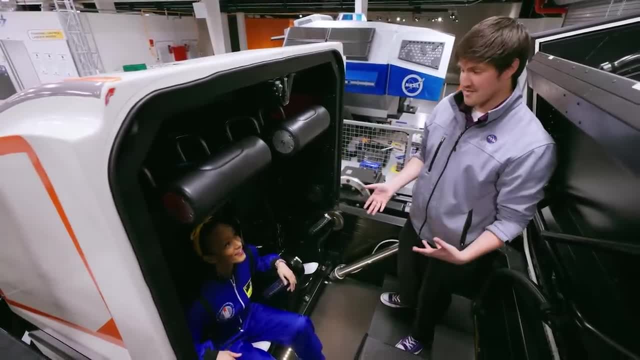 coaster. Yeah, exactly. OK, We want to make sure you're as safe as possible. OK, That's good. So I'm going to lock you in. OK, What I want you to do: put your arms up and you're about to go on a roller coaster. 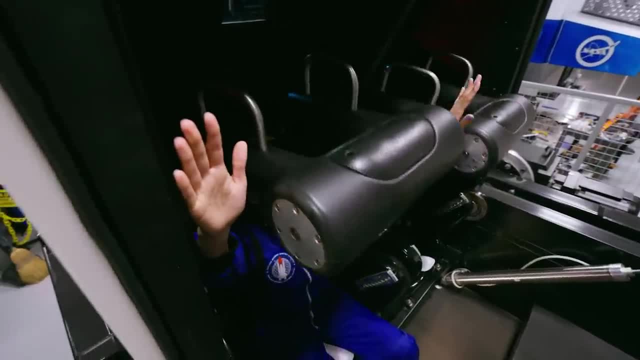 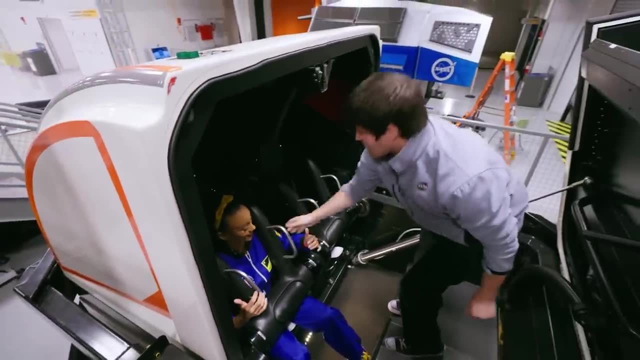 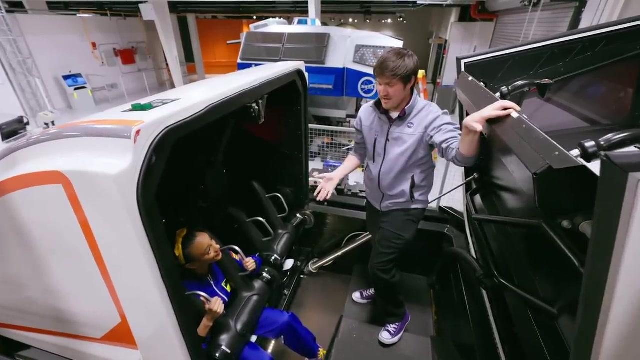 OK, Woo, And then the restraints are going to come down. There you go, Nice and secure, All good, Feel safe, Yeah, OK. Now what's going to happen is when I close this door, we're going to start the simulator. 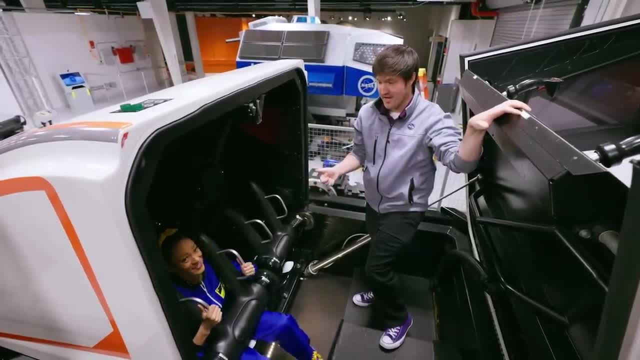 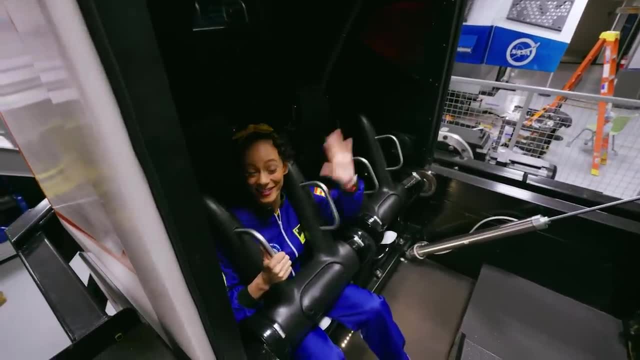 and you're going to fly and do all the cool stuff on Mars. OK, Awesome, Ready. Yes, I'm so ready, Awesome, OK, So I'm going to close the door now. Bye, All right, See you soon. 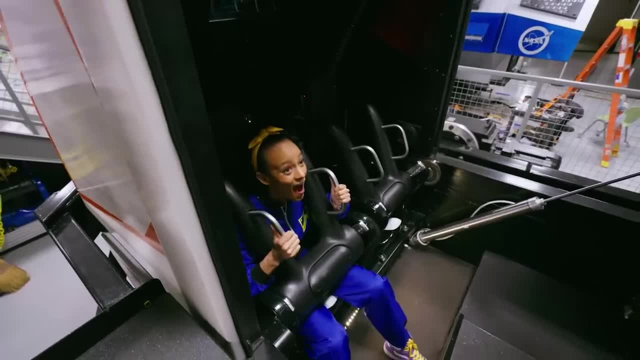 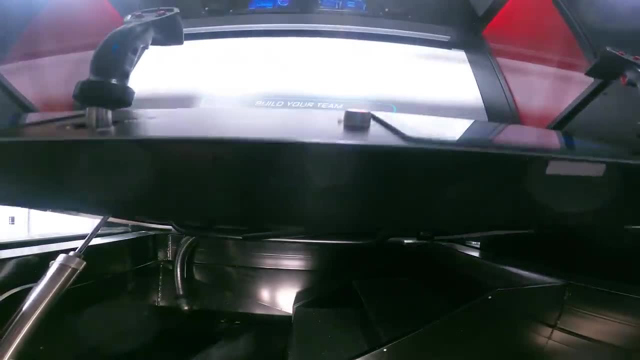 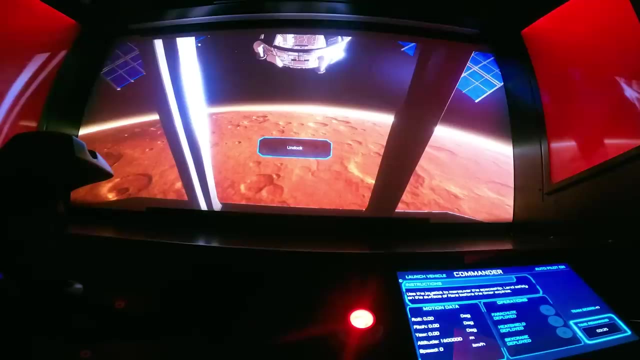 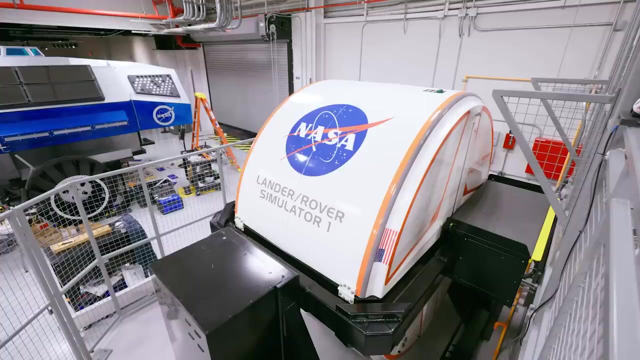 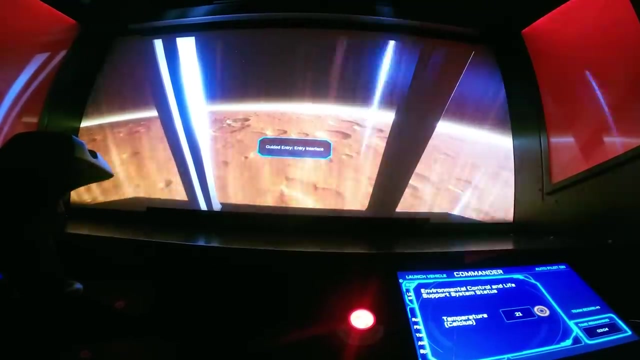 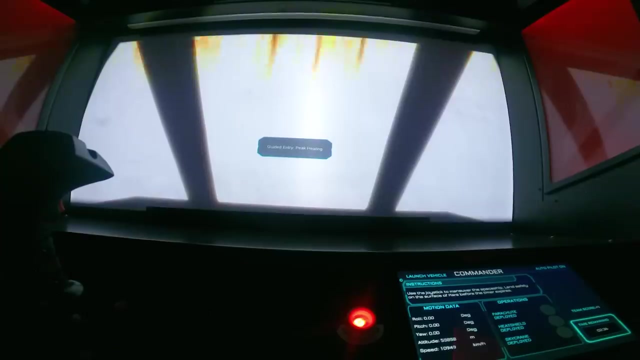 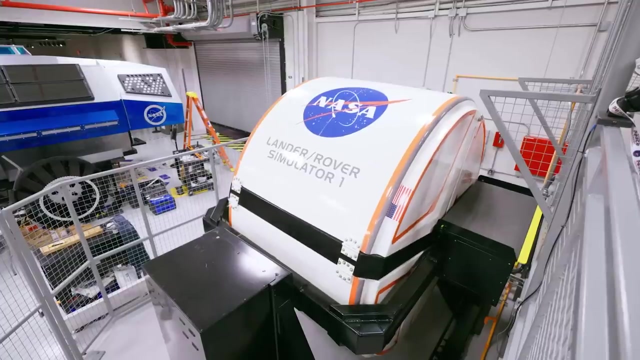 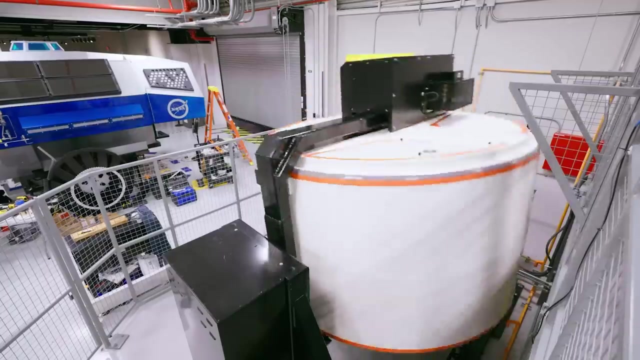 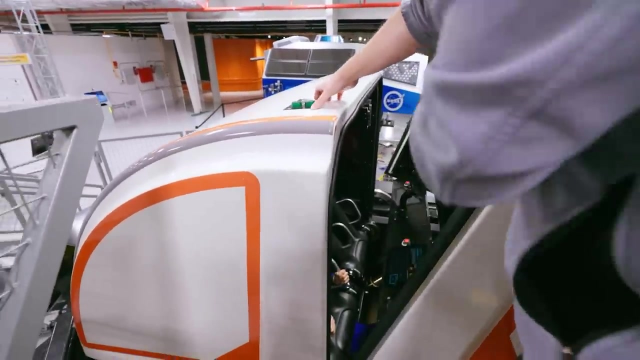 I'm going to Mars. Whoa, Wow, It really feels like I'm getting ready to go to Mars. This is amazing. Here I go, Hey, there, Hey, Welcome back. That was amazing, Mm-hmm Yeah. 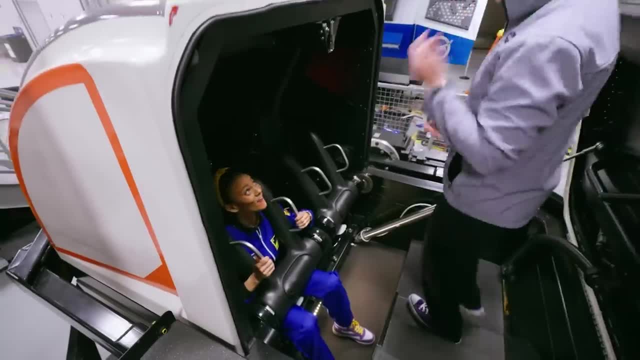 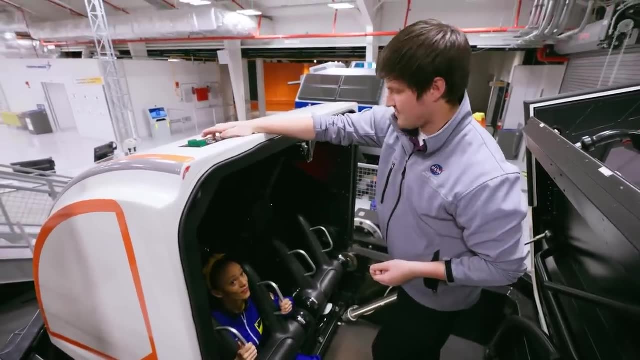 OK, Whoa, Did you see that? You did a great job. Thank you. Now I'm going to get you out of there. OK, So first things, first restraints. We're going to raise those up. OK, There you go. 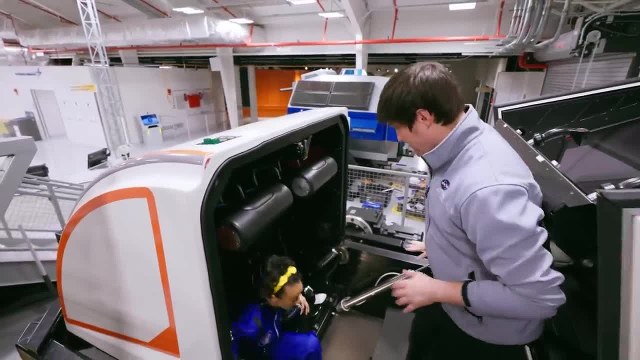 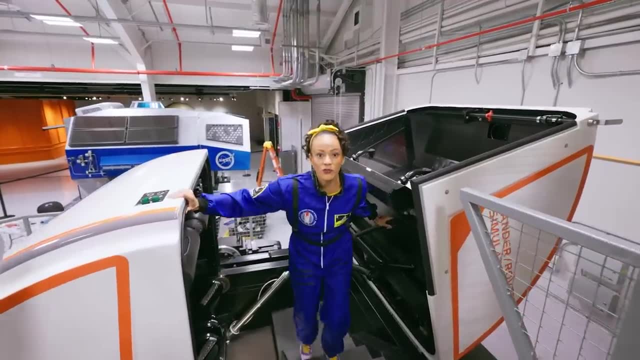 Whoa, Good job. OK, You can come on out this way. Be very careful though, Whoa, You can use the handrail. Yeah, That was wild. Did you see me flip upside down? Whoa, You OK. 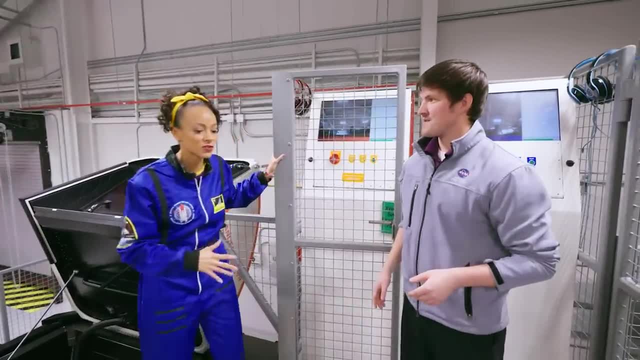 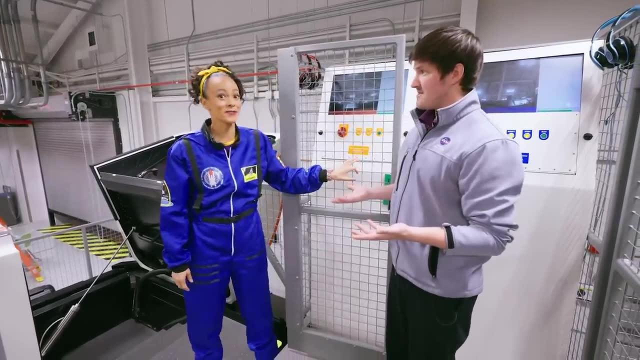 Yeah, I'm good, I'm good, OK. So is that what it feels like to land on Mars and then drive on Mars A little bit? Yeah, Yeah, It's a good simulation, right? Yeah, That was really fun. 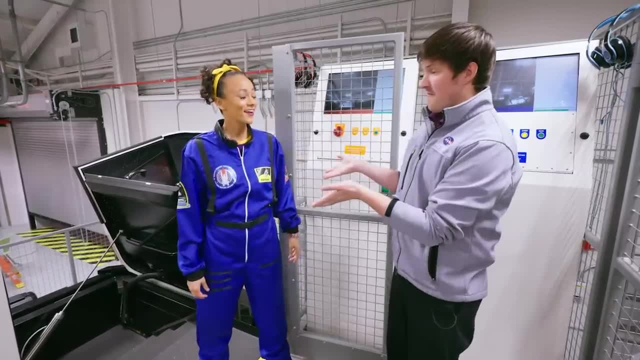 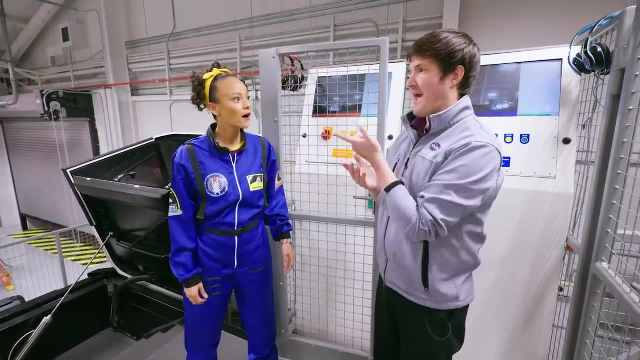 Thanks for letting me experiment with that. Oh, no problem. Yeah, So for that you got to drive to our Mars base, one in the simulation. Yep, Do you want to see our simulated Mars base that we actually have here? Oh, yeah, 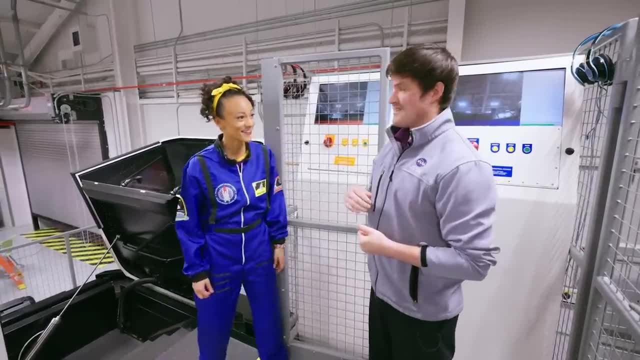 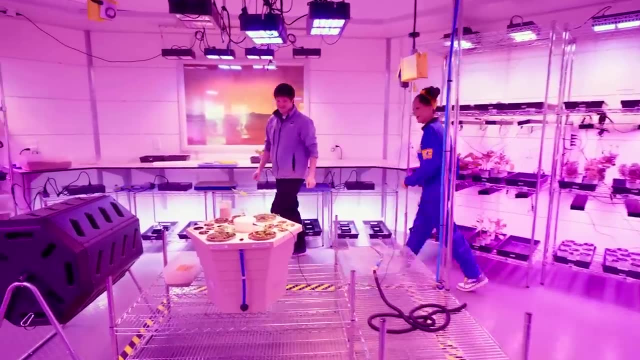 That's last on my list. Awesome, All right, Want to go? Yeah, Let's do it, Let's go Cool, Come on, Come on over this way. Whoa, Whoa, Wow. So welcome to our Mars base one botany lab. 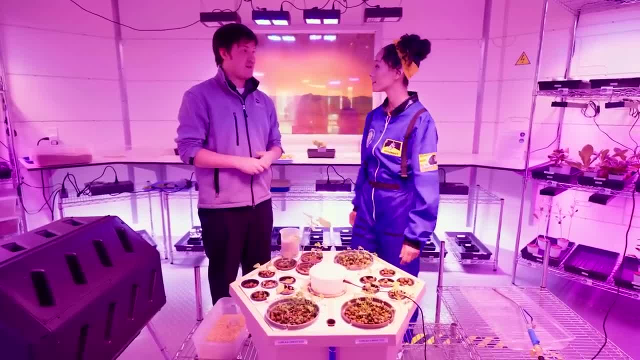 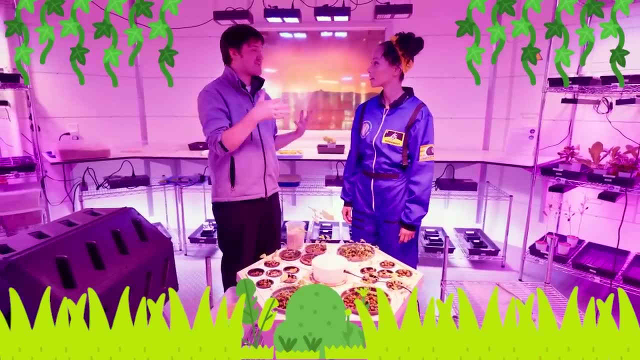 Oh, thank you. I've never been in a space like this before. Yeah, Do you like it? Yeah, It's very cool. Lots of plants in here. Yeah, We have tons of different varieties of plants because we want to see what types of things. 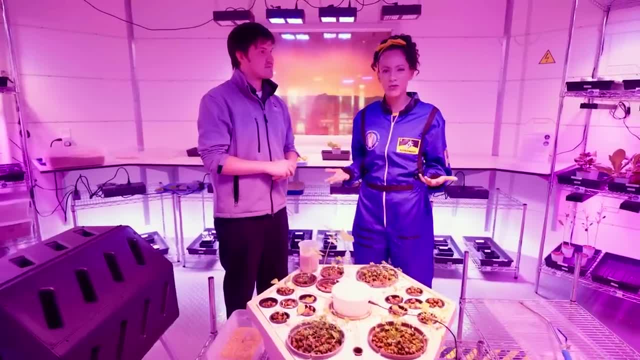 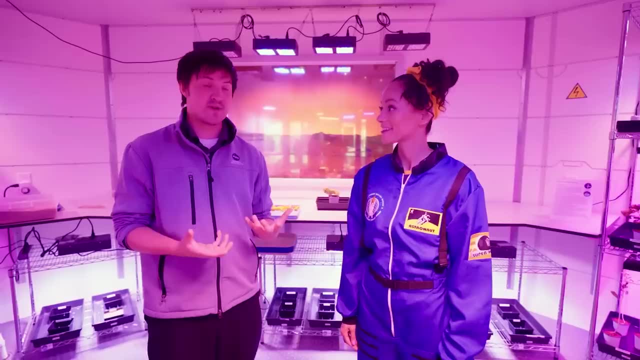 we could grow on Mars. Oh, why would you want to see what can grow on Mars? That's a really good question. So if we're going to go to Mars, like we plan to do, so we can work and do scientific experiments. 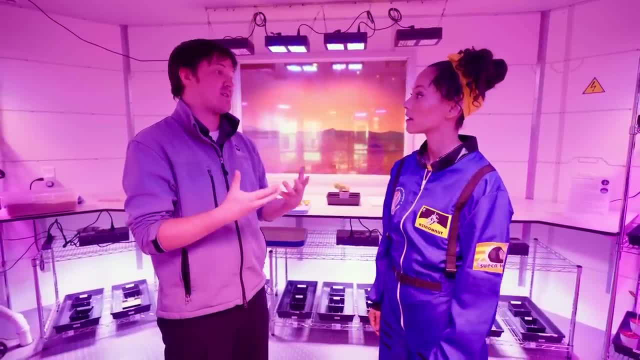 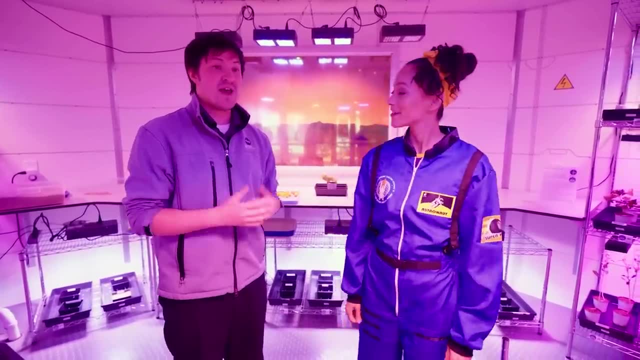 we got to test what we could have to eat on Mars, because we can't bring all the food we're going to take there. Yeah, That makes a lot of sense. Oh, that's cool. Yeah, Now growing on Mars is really difficult. 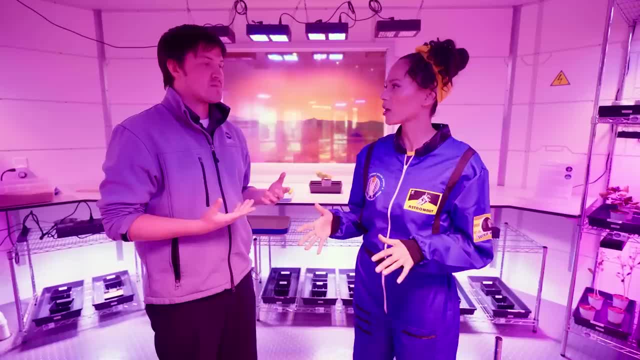 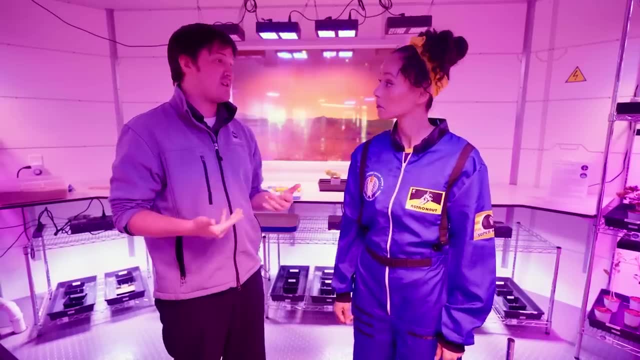 It's not like Earth. Oh Yeah, Is there not dirt on Mars? Well, there's dirt on Mars, but when it comes to Mars, it doesn't have the right things that plants need to grow. Oh, So, do you happen to know what things plants need to grow? 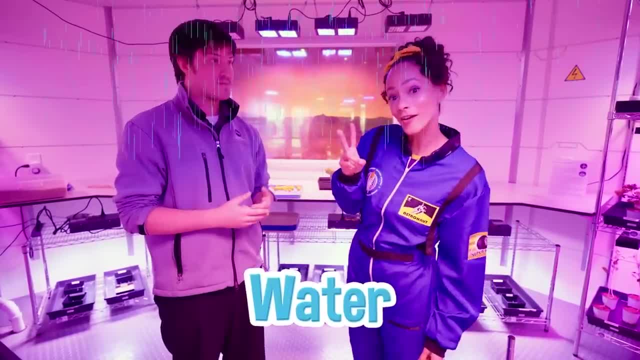 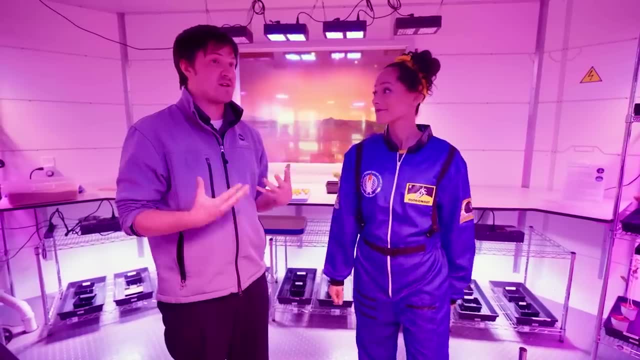 Yeah, They need light and water and dirt or soil packed with nutrients, and you need the right temperature. Yeah, So they need tons and tons of stuff, and it's all very specific to the type of plant. Yeah, Mm-hmm. 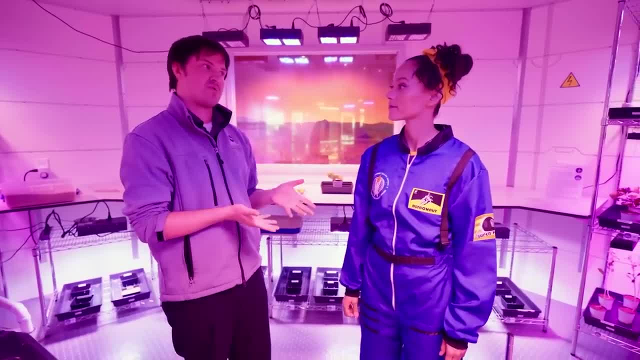 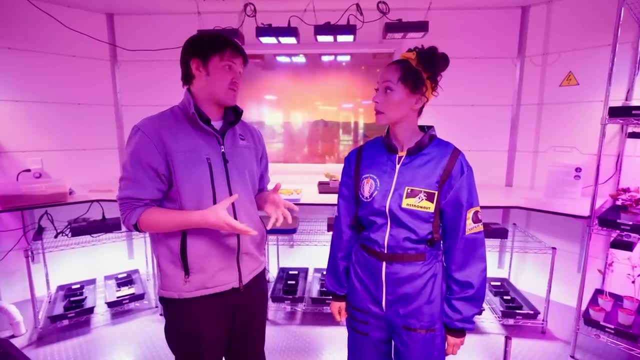 Now, when it comes to Mars, it has dirt but there's no nutrients in it. Oh, So if I just went outside and grabbed any old dirt, it's not really going to simulate how well it works on Mars. Oh Well, what does it feel like? 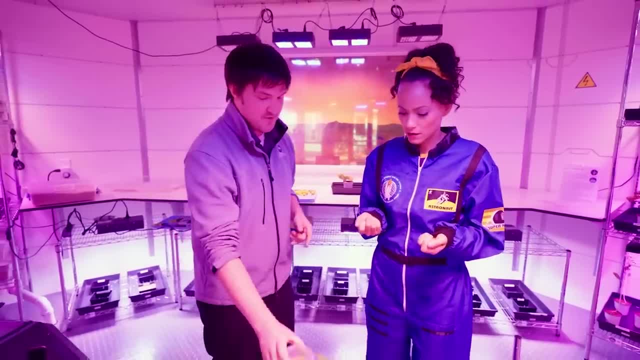 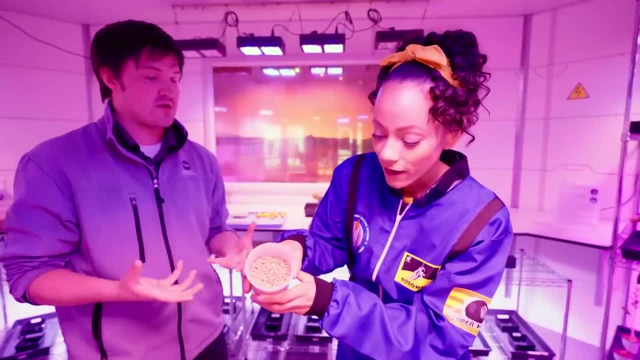 What's the dirt feel like on Mars? Well, I have a really good example. Oh, So this is some of the stuff that we use. Oh cool, It's a simulation of what Martian dirt or soil is like, So this isn't really from Mars. 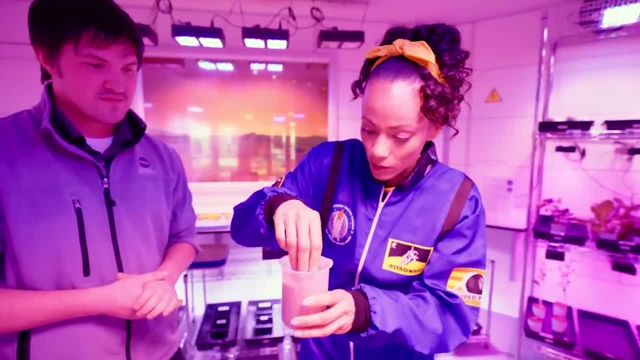 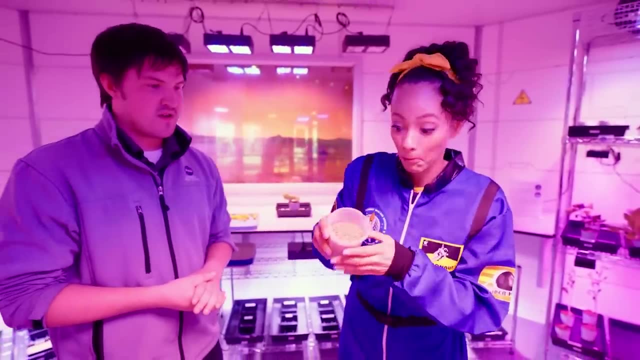 No, it's not really from Mars. Huh, Look at this. Whoa Kind of feels like a bunch of little rocks or little pebbles, Yeah, Huh, So it's like a lot of clay and iron. It's not good for plants, sadly. 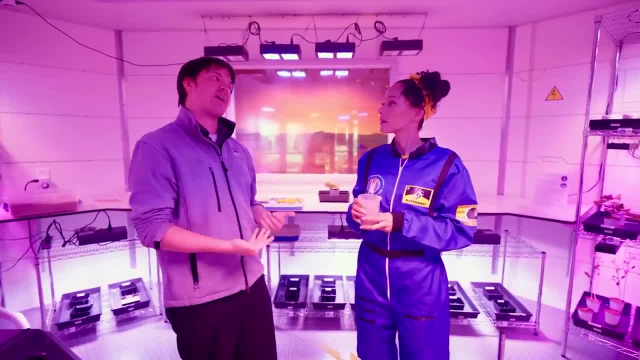 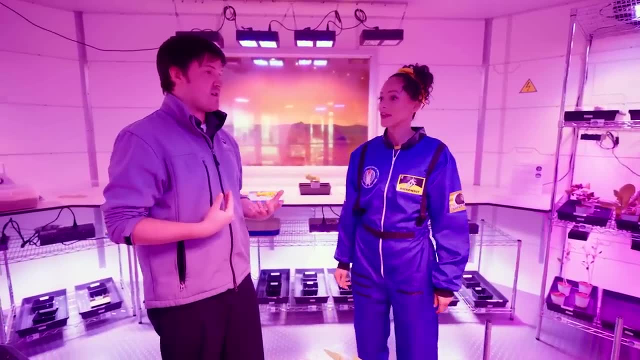 So we have to add in nutrients plant food so that way they can grow a lot easier. Oh, gotcha, All right, cool, Yeah. Now, like I was saying, we've grown tons of stuff in here. Yeah, I can tell. 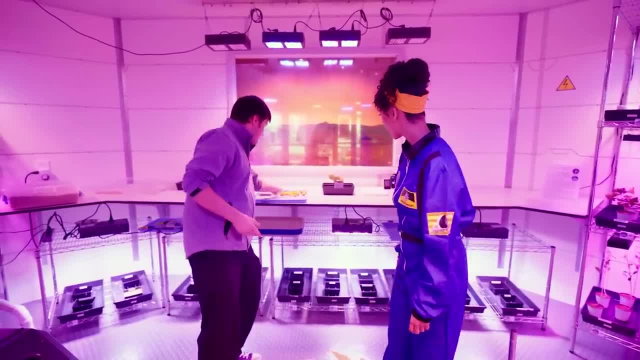 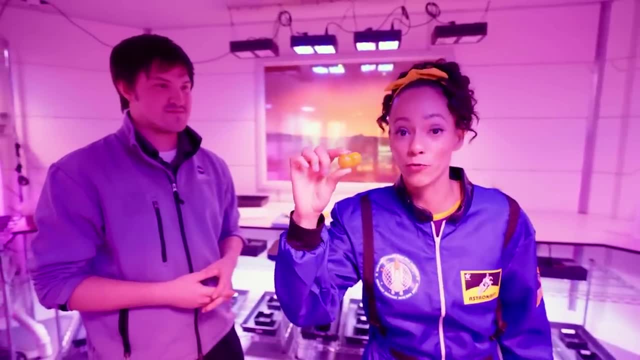 We've grown things like lettuces and even tomatoes. Oh, I love tomatoes. Wow, Can you imagine eating a tomato that grew on Mars? Wow, It's super cool, right? Yeah? Now other things we've grown I want to show you. 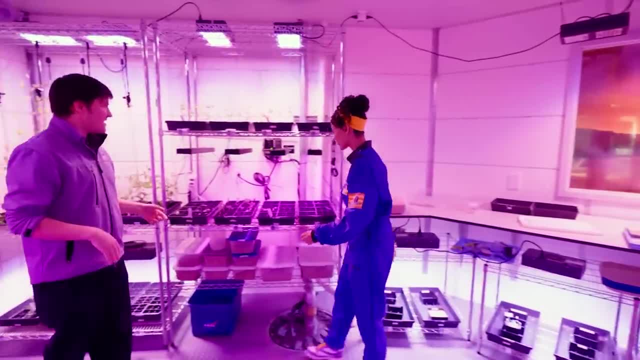 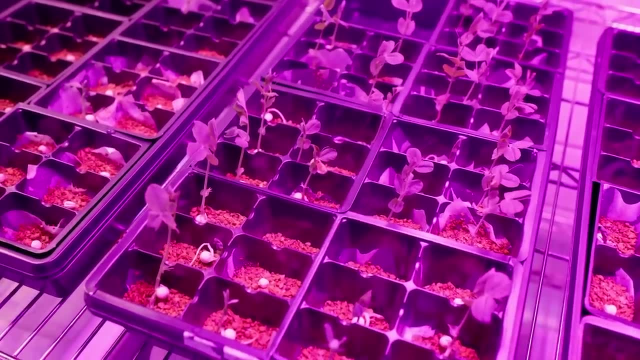 are some of our peas. Come on over this way. So these are some of the peas that we've actually grown. We've tested different types of plants, but we also want to test how those plants grow in different conditions. OK, So some of the things you mentioned before. 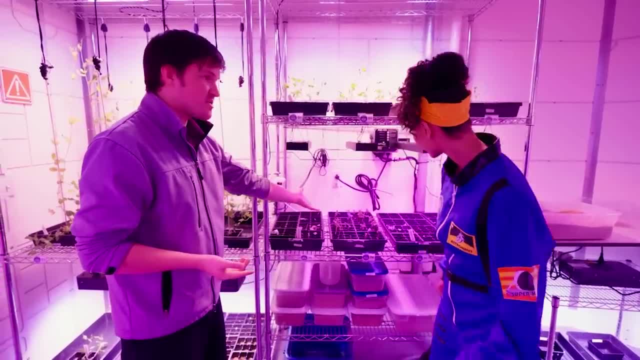 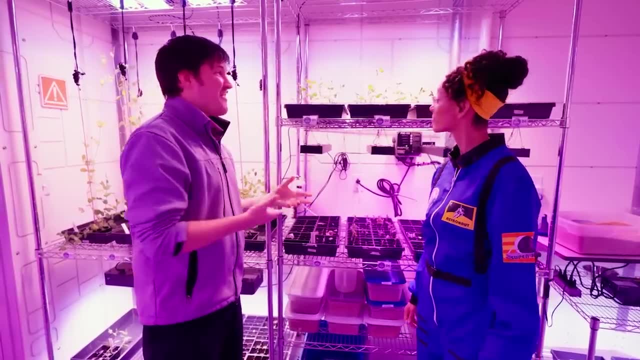 of growing include water. We have water in the trays That helps them grow, All right. And then we have some nutrients in some of the arsolite, the dirt in there, Mm-hmm, And then we have different types of light, even. 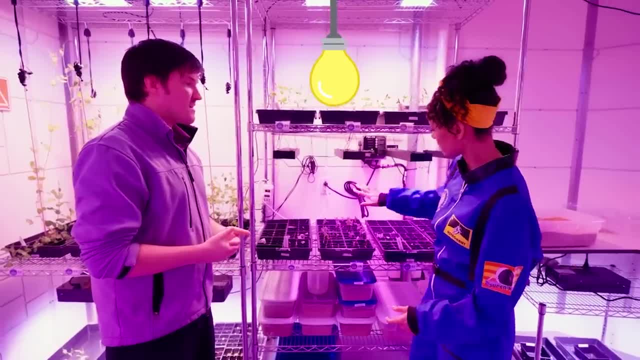 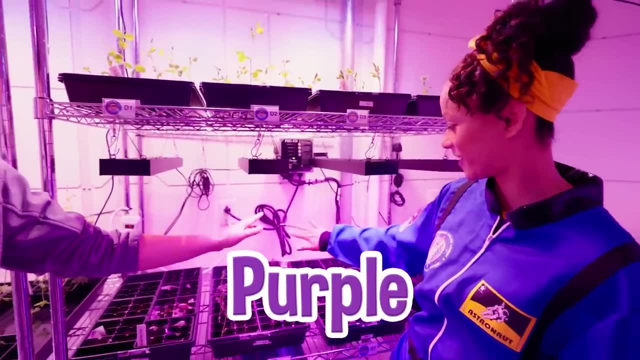 Oh, different types of light. Oh, yeah, it does look different. Yeah, so you can put your hand underneath. So down here we have like this weird purple magenta. Oh, I love that. I love purple Yeah. 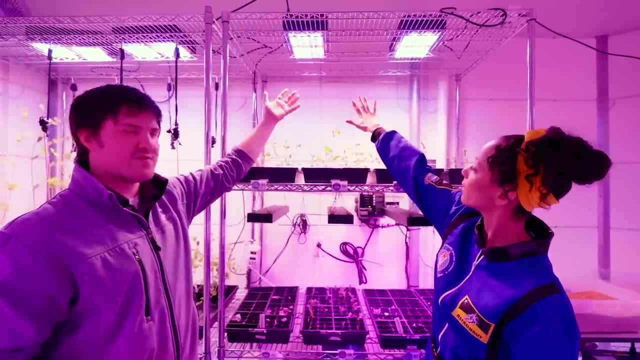 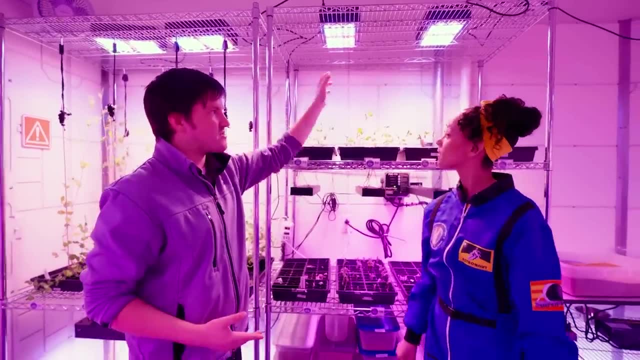 It's got red and blue little lights And then up here on top we have some white light with it. It's a little bit different. Yeah, it looks very different, Yeah, So we want to test how the plants grow in different light conditions. 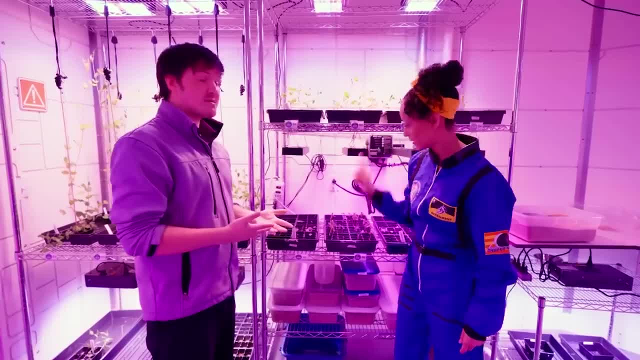 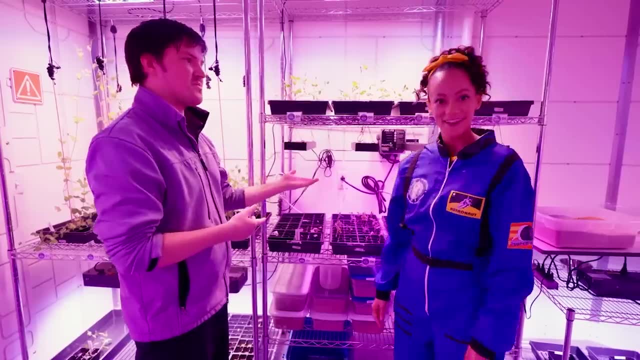 Oh, like these plants up top are growing a lot higher than these plants here on the bottom. Yes, So hey, we know. now for the peas to use more of these lights rather than these ones. Oh, just always experimenting, Yeah. 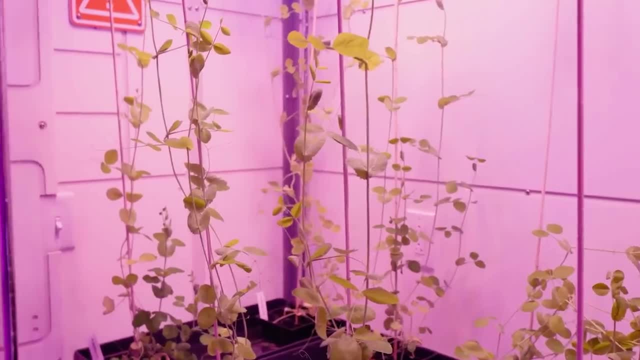 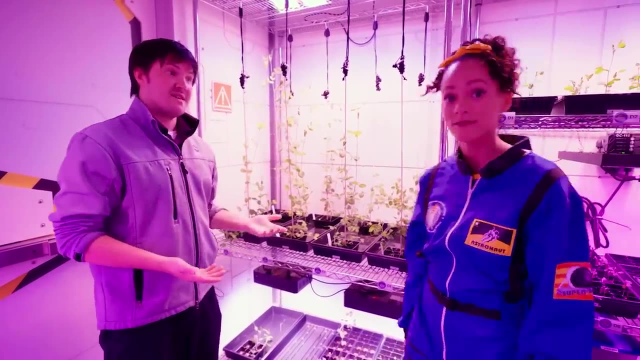 And you can even see some of the ones that we've kept growing even longer. They're even super, super high because they have that nice light. See, they're growing towards the light. Yeah, Wow, they really like this light. Yeah, yeah. 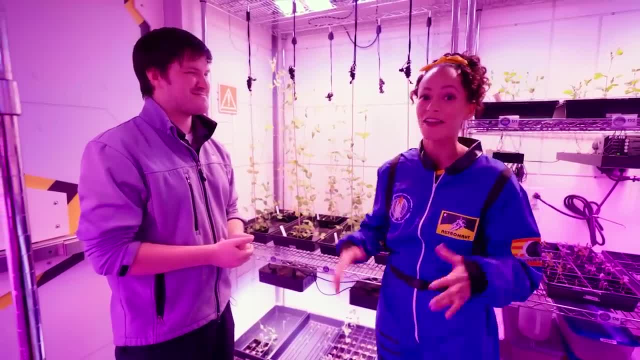 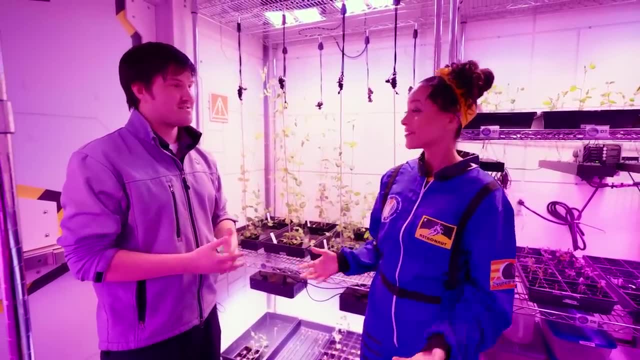 Wow, Well, thank you so much for teaching me all about space and what it would feel like to land and drive on Mars and spacewalk, and now Mars base. Yeah, You've been awesome, Thank you, Thank you, Well, have a good day. 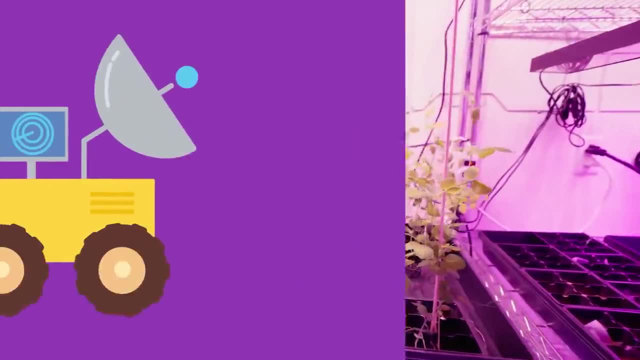 I'll see you around. Bye, Thanks, Daniel, Let's go. Wow, We did everything on my list. What a great day. We got to experience a spacewalk experience, landing and driving on Mars, and we got to go to Mars base. 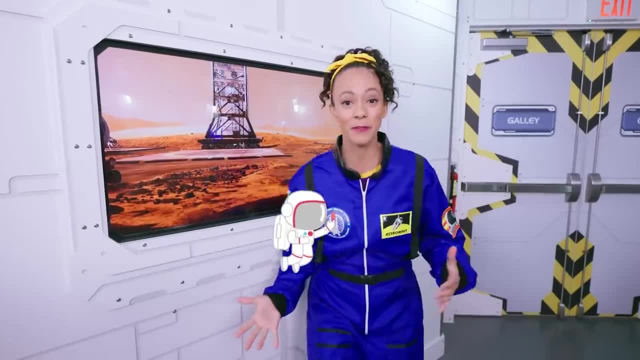 Wow, Space is so amazing. Thanks for learning with me today. Well, that's the end of this mission and the end of this video, But if you want to see more of my videos, all you have to do is search for my name. 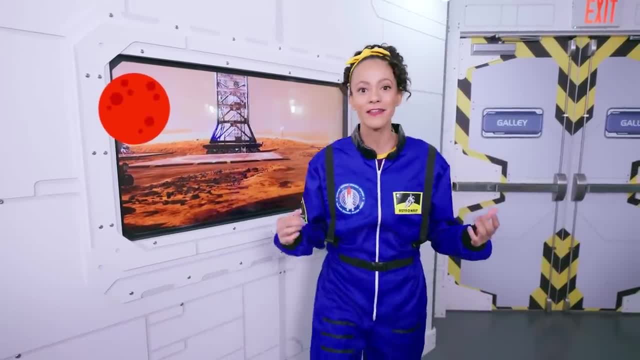 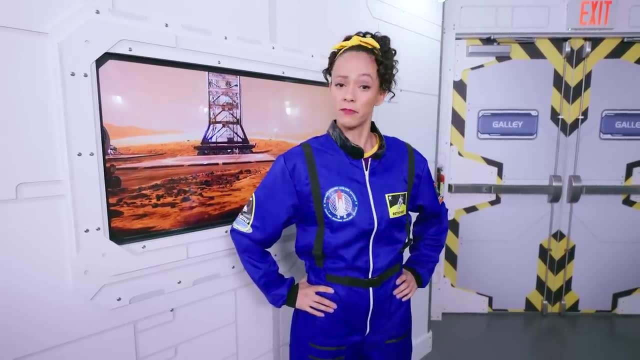 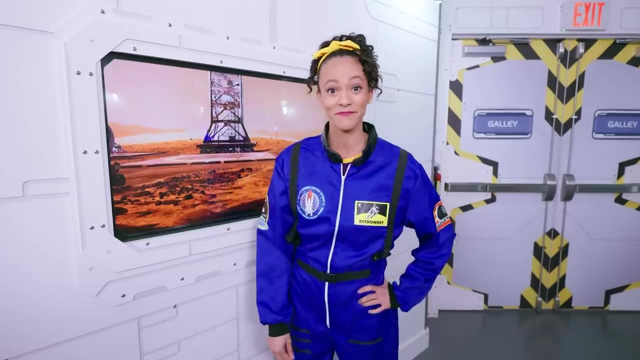 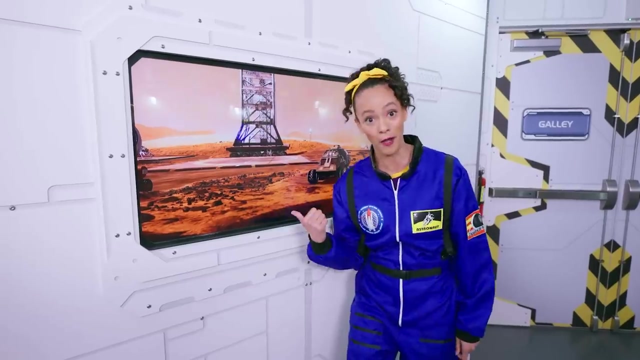 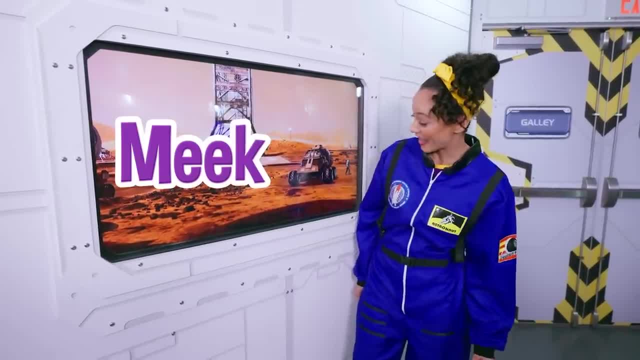 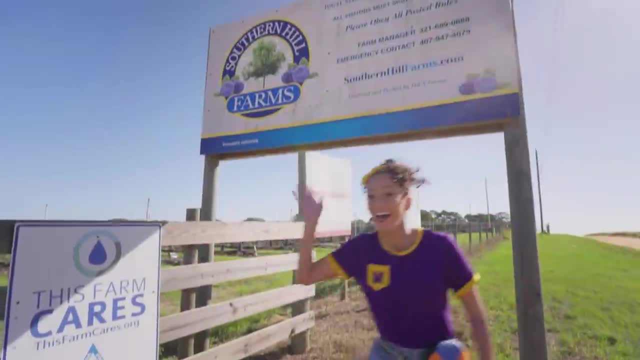 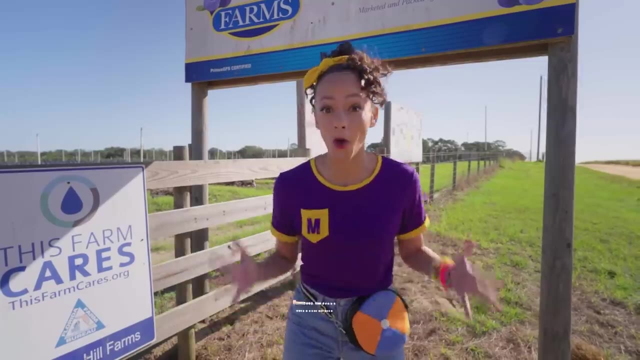 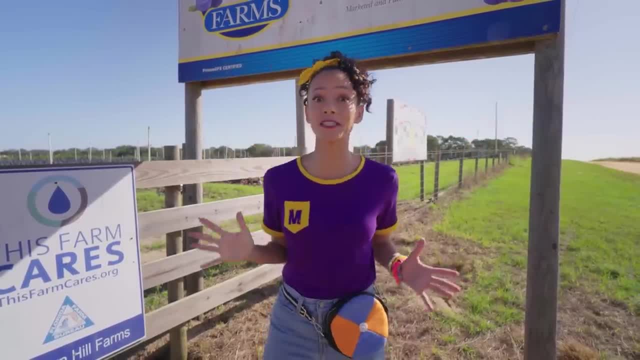 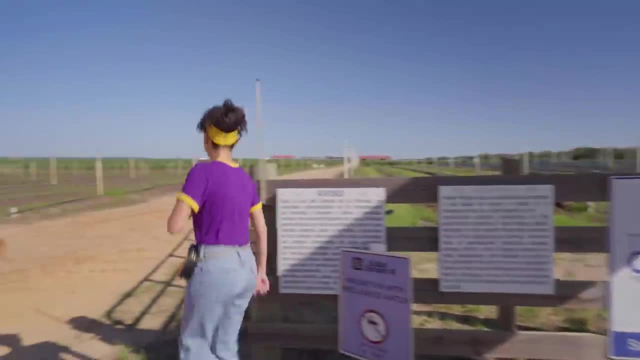 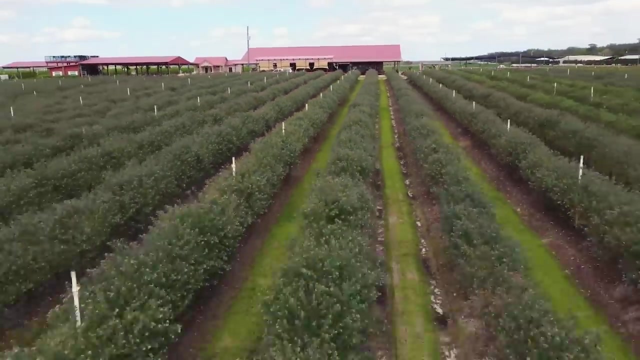 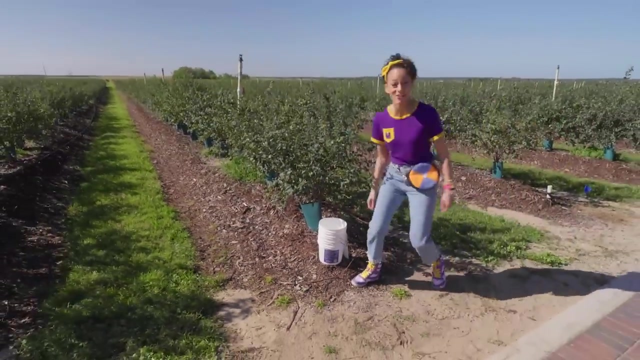 make blueberry lemonade and find some beautiful sunflowers. I love sunflowers because they're yellow, one of my favorite colors. Come with me, Whoa cool. These are buckets that you can use to collect the blueberries in once they're picked. 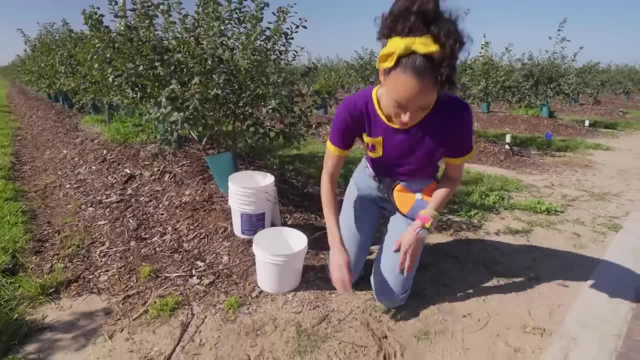 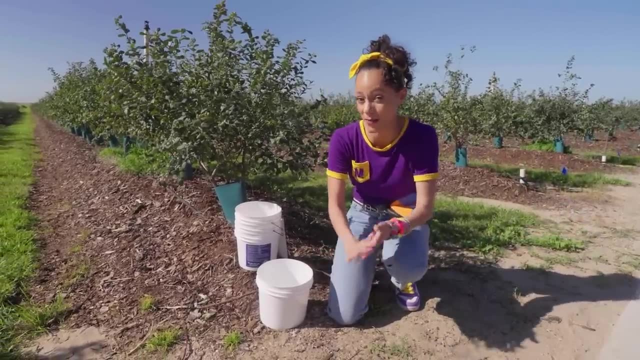 That's so fun. Oh, come down here, look at this. Have you ever seen sand on a farm before? Yeah, you might not expect sand at a farm, but this sand that's really soft and fine. it's called sugar sand. 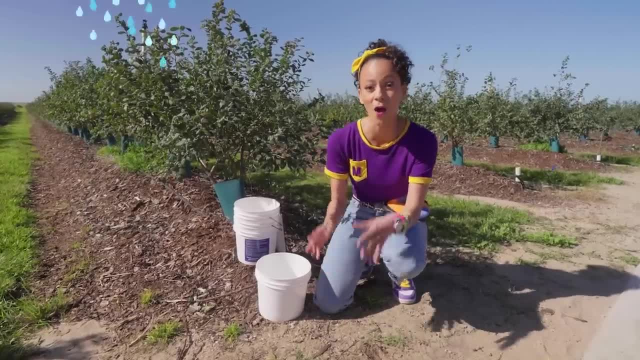 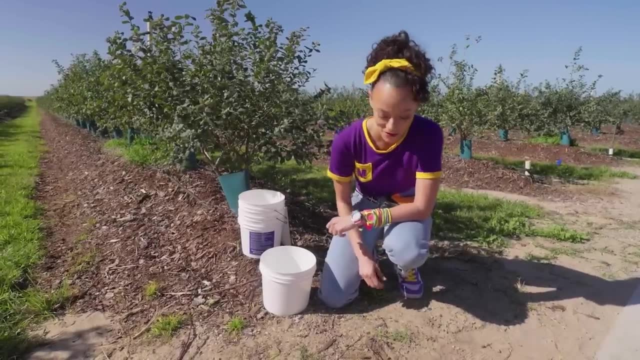 and it's really helpful for the blueberries. With this sand, the water can drain quickly, which is super important because blueberries do not grow in a lot of water, So this sand's really fun to play with and touch, but it's really important for the blueberries. 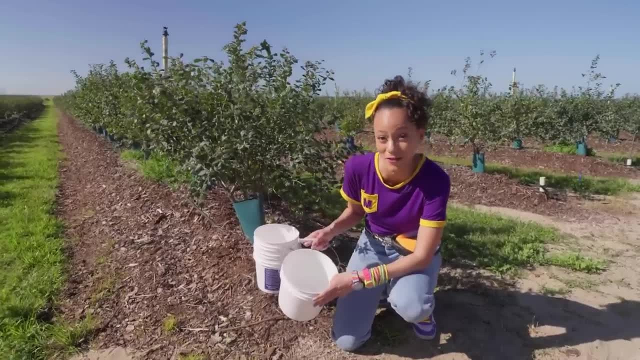 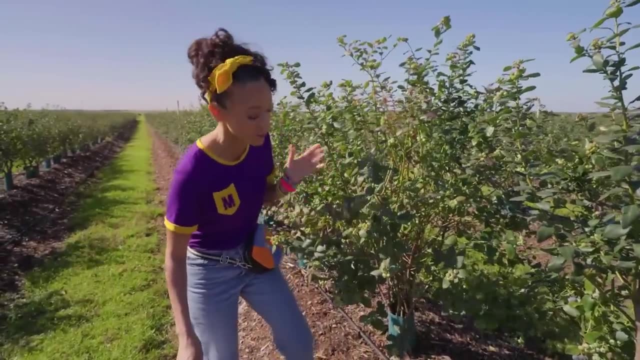 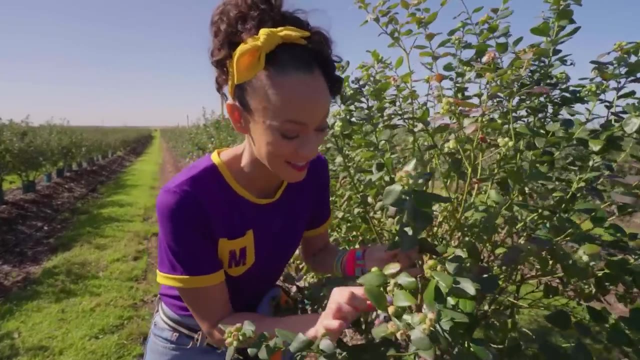 so I'll just leave that there. Do you want to pick blueberries with me? Let's go. Take a look at this. It's a blueberry bush, or a shrub. Come a little closer, See, There's whoops. 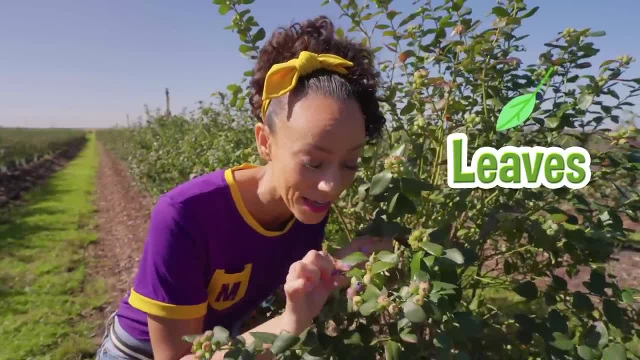 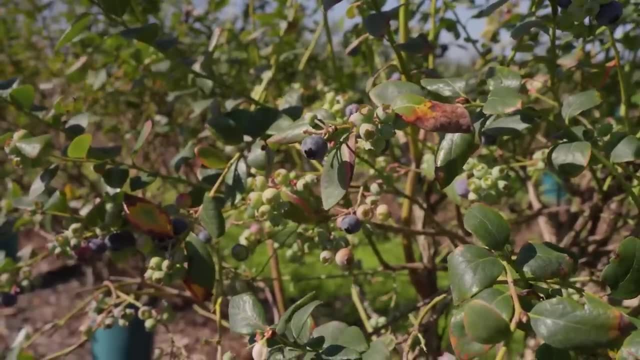 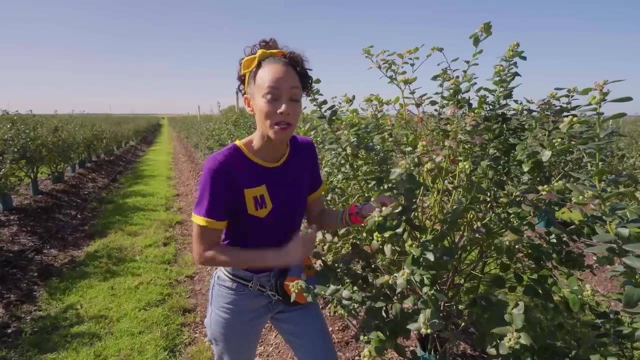 The stem and the leaves and look the fruit- The best part. So see how some of these berries they're different colors. There's kind of a purple, a blue and a green. Do you know which berry is ripe? 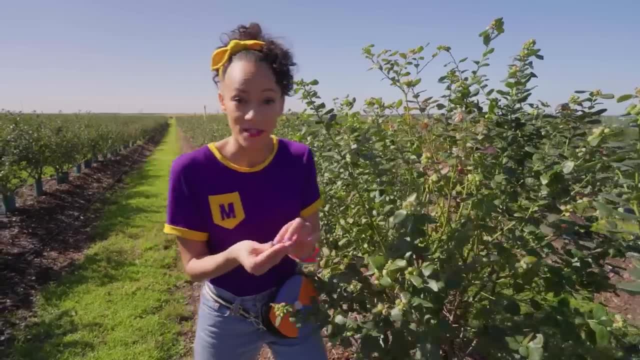 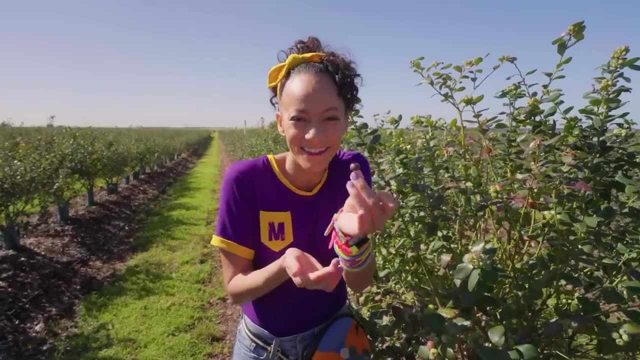 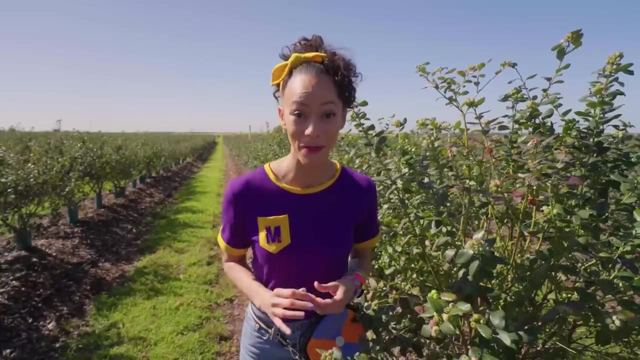 That's right. this one, the blue one, Those are the ones that you want to pick, And ripe means that it's fully grown and ready to eat. They're so cute. I know We could pick 20 ripe blueberries. 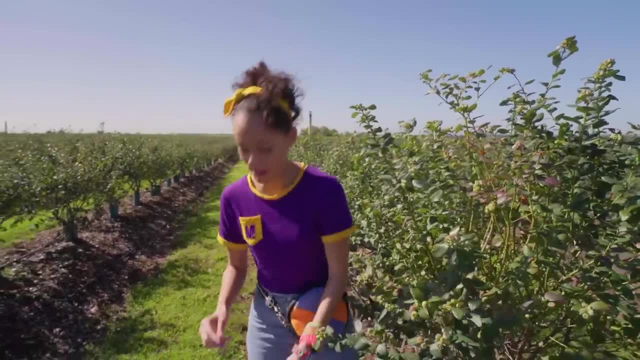 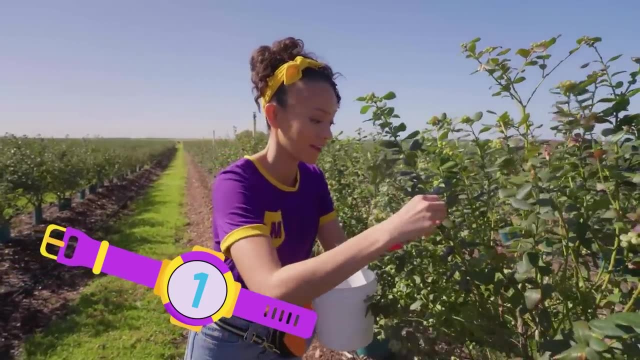 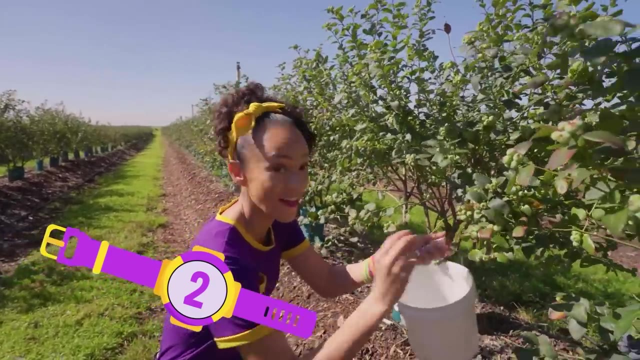 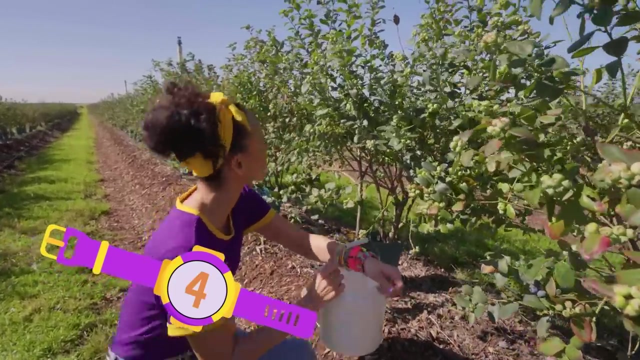 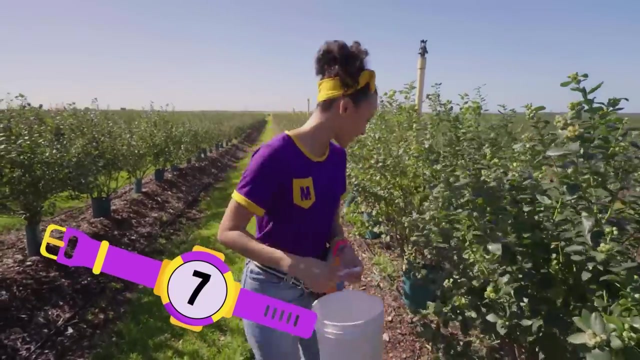 Will you count with me? Cool, So we have one. Hmm, Oh, here's another one. Two, Whoop, there's one down here. Three, Two. One. Two, Three, Four, Seven, Eight, Nine. 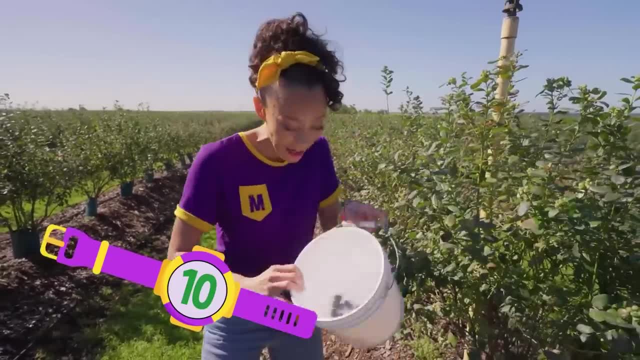 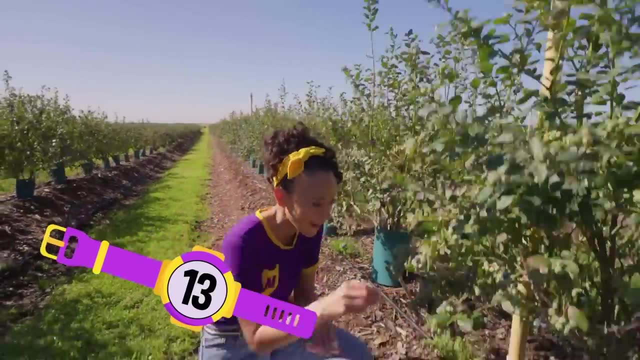 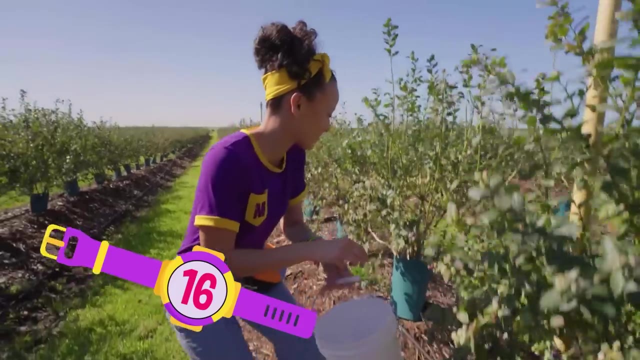 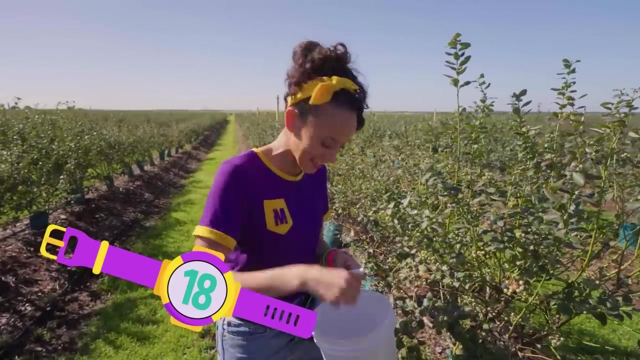 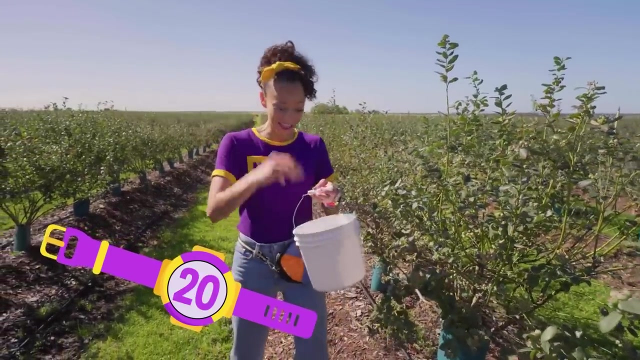 10. Two, Three, One. Two, One, Two, Three, 14. All done in seven parts. Four, Four, 10. Four there, 17, 18, 19, 20, 20 ripe blueberries. thanks for counting with me. see, you can. 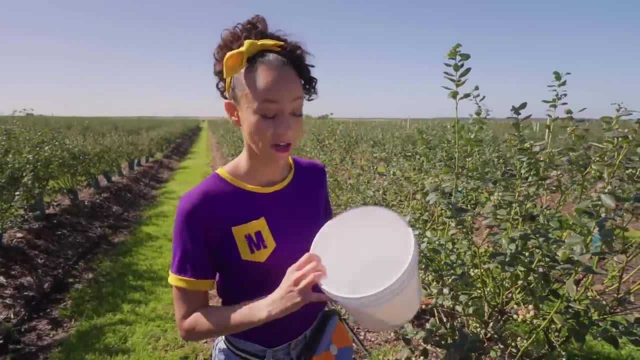 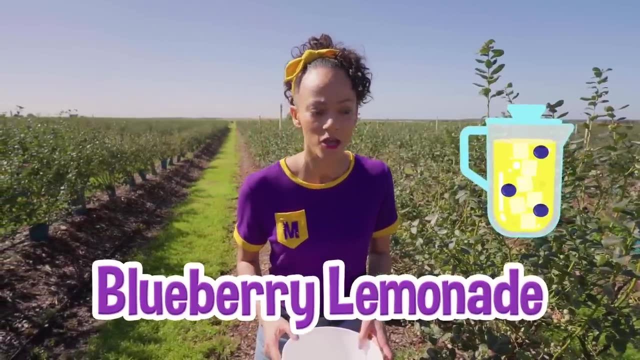 pick them off of the bush, or you can pick them up off the ground, as long as they're nice, blue and right. oh, this is gonna be really good in my blueberry lemonade. you can do all sorts of things with blueberries. what do you like to do? 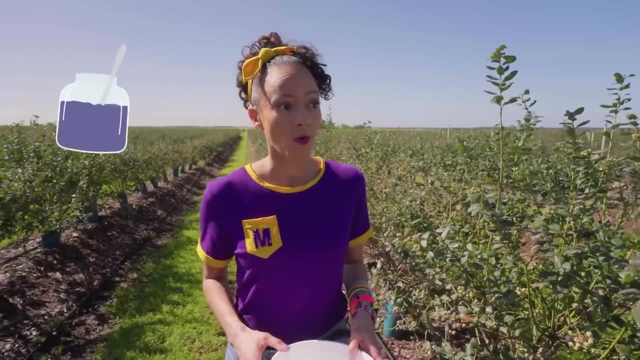 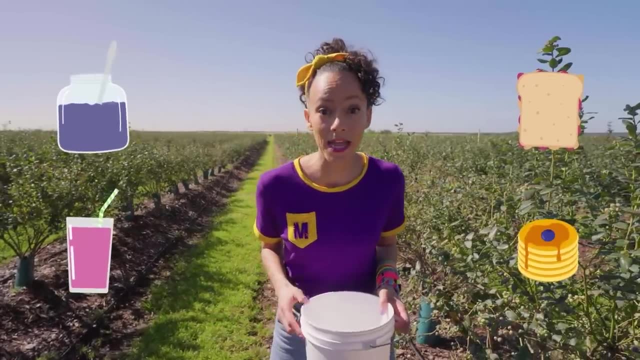 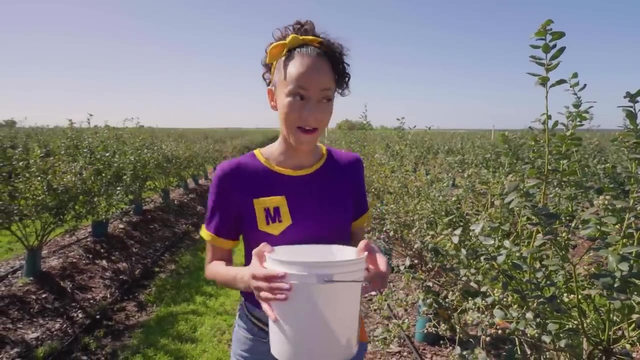 with blueberries. you could make jam or jelly for a blueberry and peanut butter sandwich, or you can make a smoothie. blueberry pancakes, cupcakes, parfaits, juice- there's so much you can do with blueberries. oh, do we keep looking at blueberries? all right, cool, let's go over there. there's more. 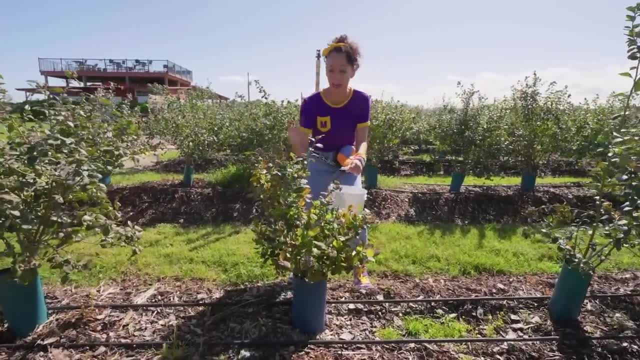 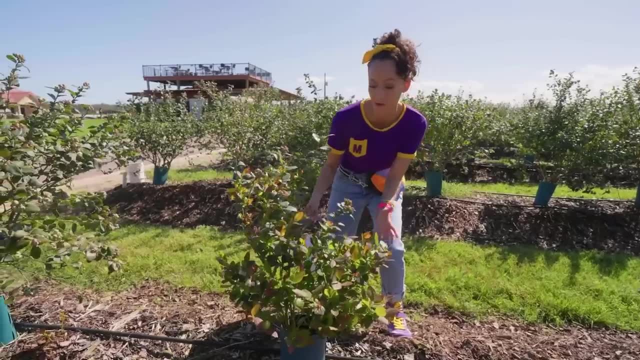 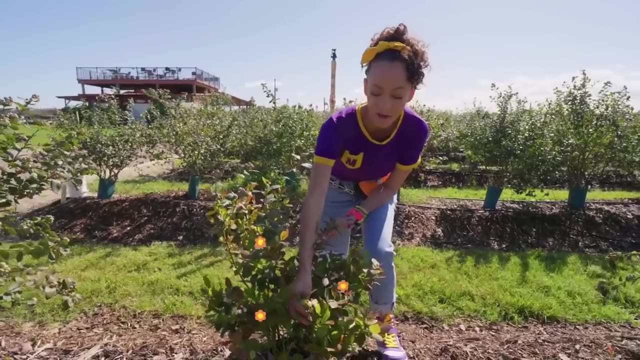 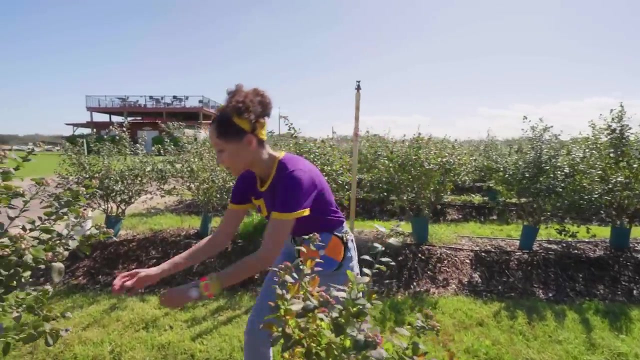 Wow, look, it's a baby blueberry shrub. see, it's much smaller than the other plants we saw, but one day it's gonna grow nice and big and full and have a ton of blueberries on it. you'll notice on the young plants they have little flowers. see, that's so cute. oh, I see another ripe blueberry here. 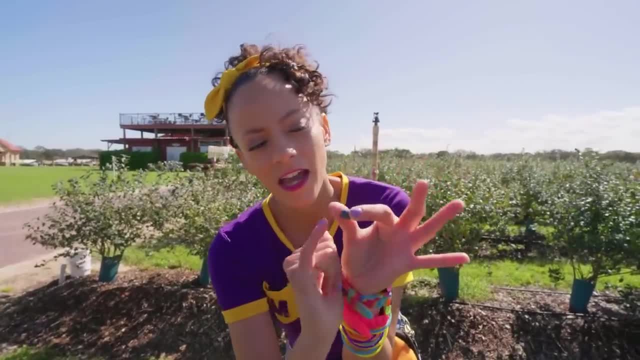 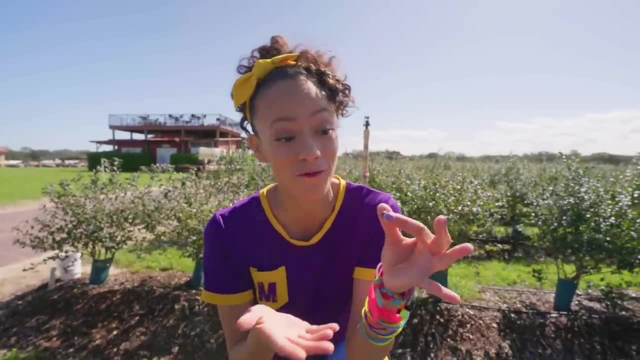 take a look. see how kind of looks white on the outside. that's called bloom, and bloom is like a sunblock for blueberries: it protects it against the Sun, so the blueberries don't get too much sun. check it out: a really big, young, strange flower. come take a look. see, and it looks so white right on the outside. it's called Blue. replace it, love it ohLuh. just be careful. look at those little little differences in that. look, there are plenty of inherited Hilsea and Roth. just wanna put a little sticker on those. 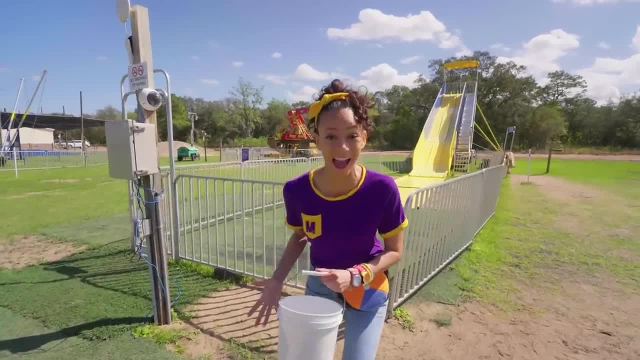 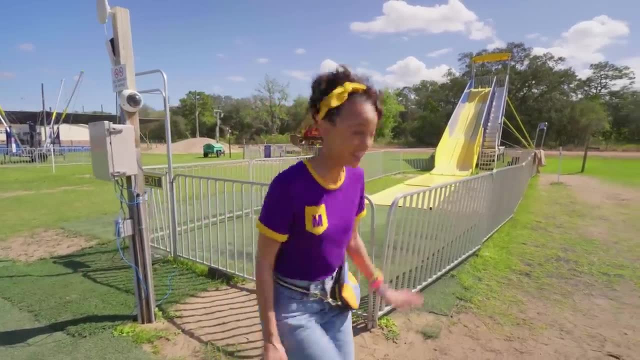 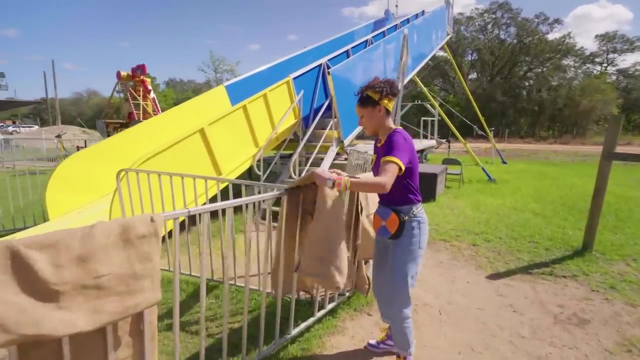 Check it out: a really big yellow slide I have to go down. Let me put my blueberries down so I don't spill any and I'm nice and safe. Come on, Whoa, I get it. You use the potato sack to go down the slide. 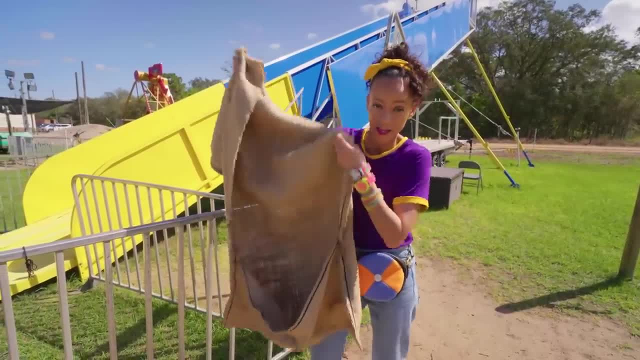 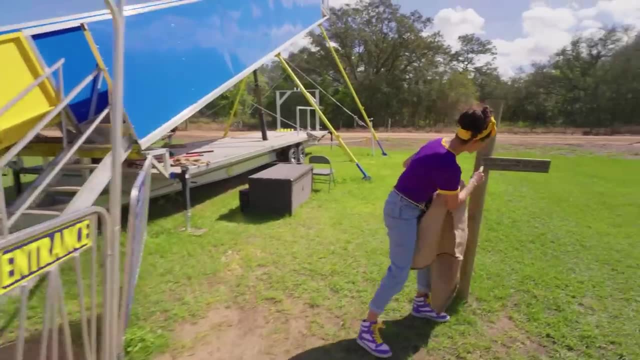 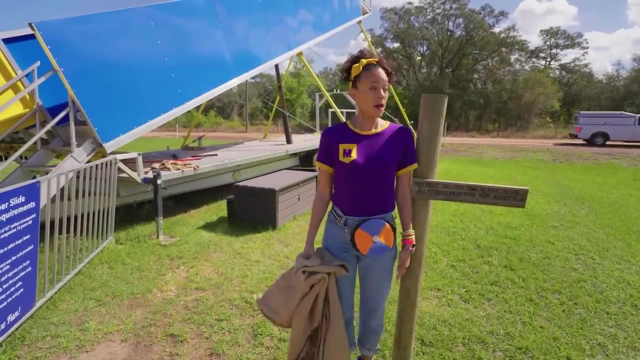 See, you put your feet in here in the bottom, get situated and then you woo, woo, woo. Oh, look at this. You must be this tall to ride alone. All others must ride with an adult. All right, let's see. 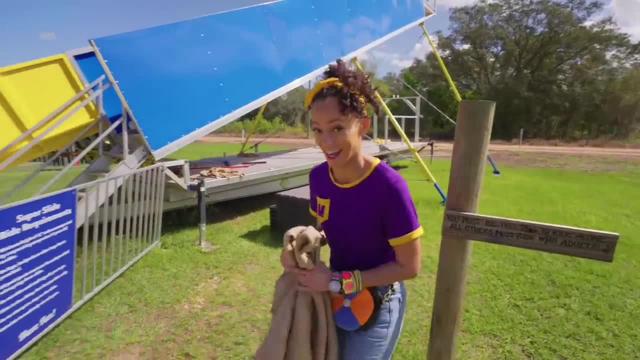 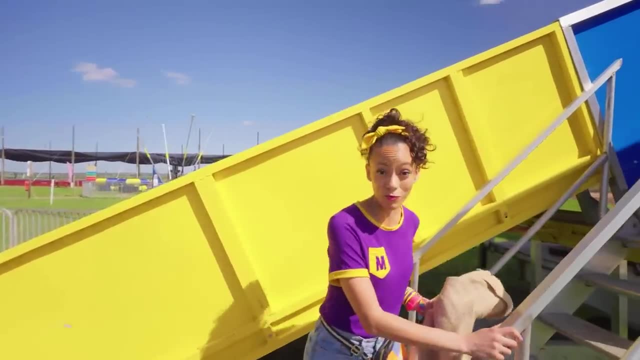 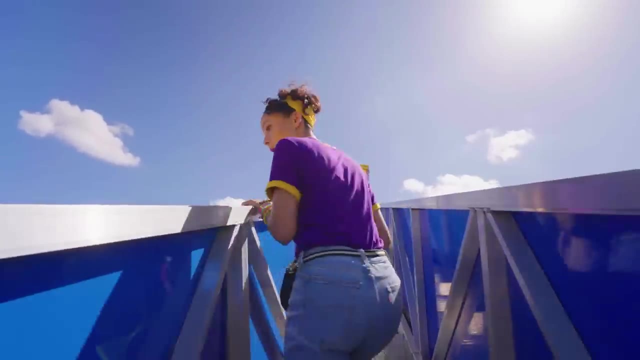 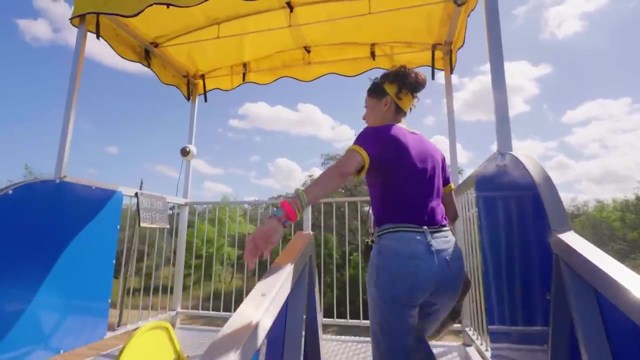 Oh, I think I'm tall enough to ride alone. Let's check it out. Hey, whoa, it's really high up. This is quite the climb. This slide is gonna be awesome. Look how high we are. You can see the entire farm. 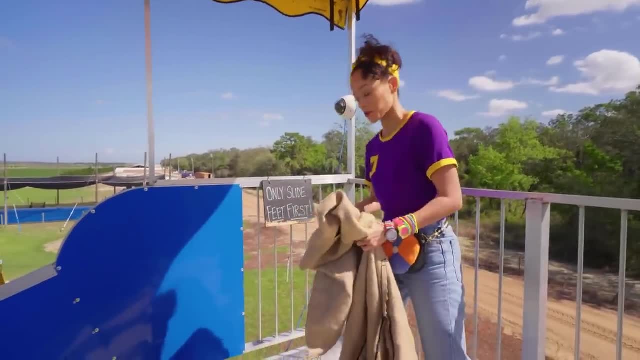 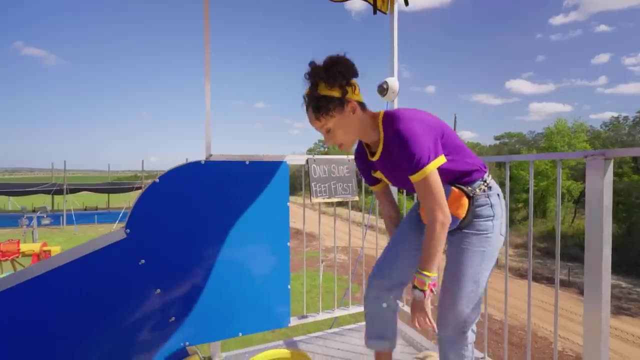 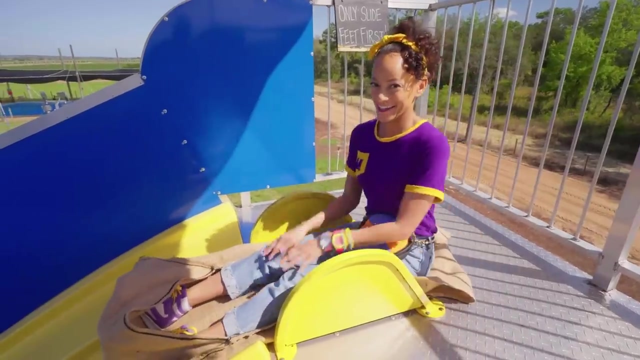 Okay, only slide feet first. Okay, that was my plan anyway. Right, so you lay your potato sack down like this: Sit down and feet first. Feet will go in this little pocket here. Okay, let's go down. Okay, do you want to watch me slide all the way down to the bottom? 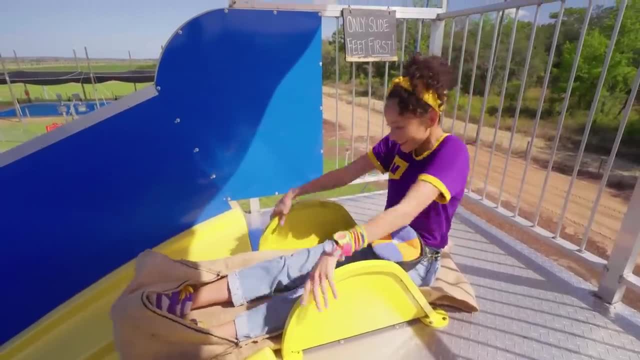 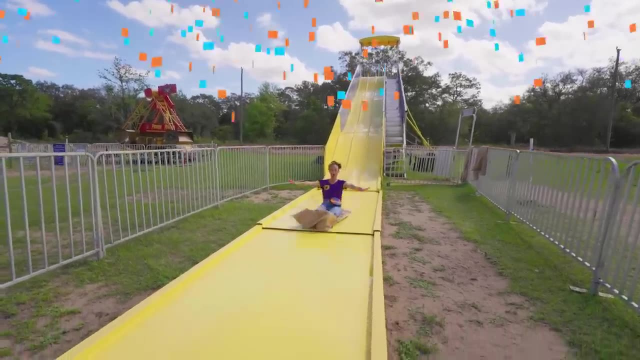 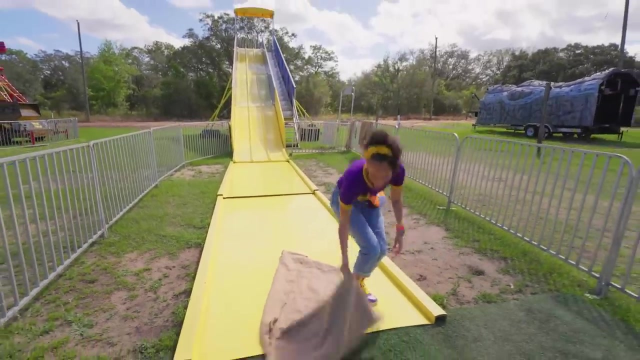 All right, see you there. Three, two, one slide, Woo, Whoa, Whoa, That was so fast. That was awesome. All right, let's put this over here. And my blueberries? Oh, there they are. 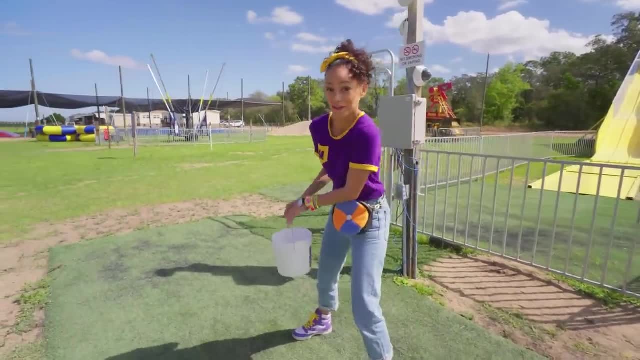 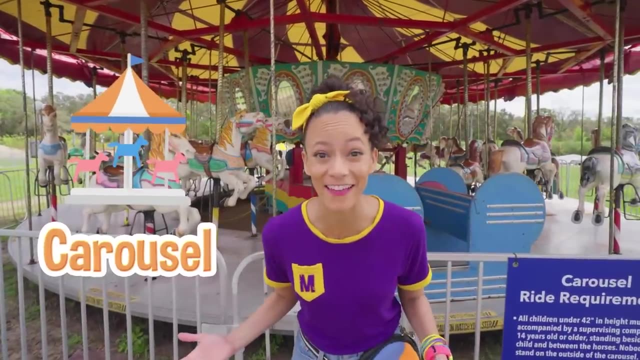 All right, come on blueberries And you come too, if there's more fun things to do. Oh, check it out, It's a carousel. Have you ever been on a carousel before? Well, let's go, Blueberries down. 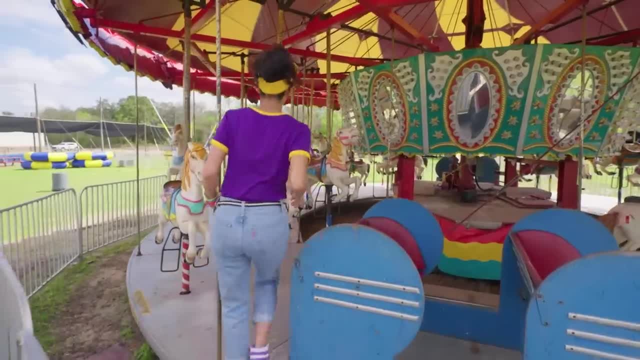 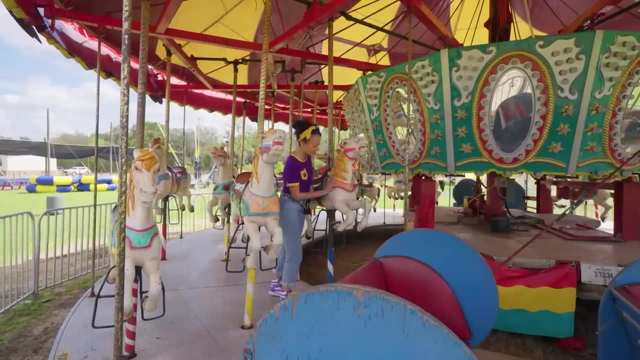 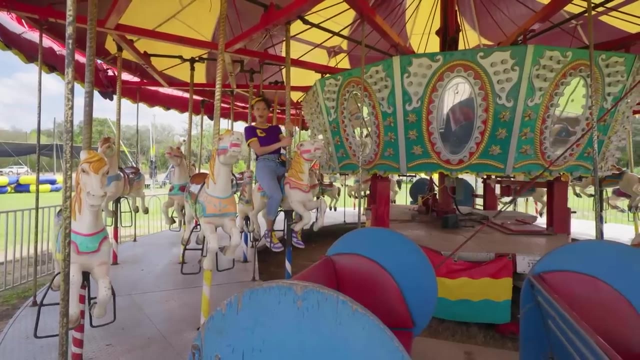 Go for a ride. Hmm, Oh, I love this horse. Oh, it's so pretty. Look at this yellow hair, One of my favorite colors. All right, I'm ready, horse, Let's go. Yeah, on the other side. 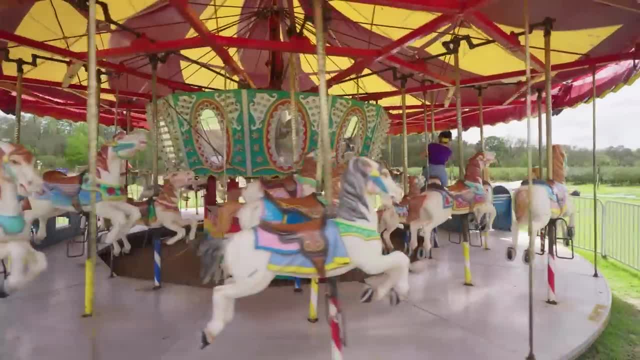 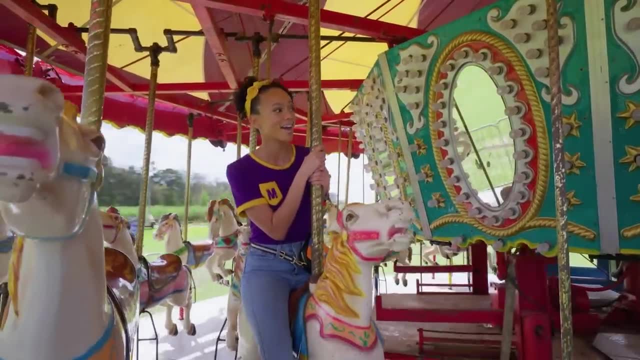 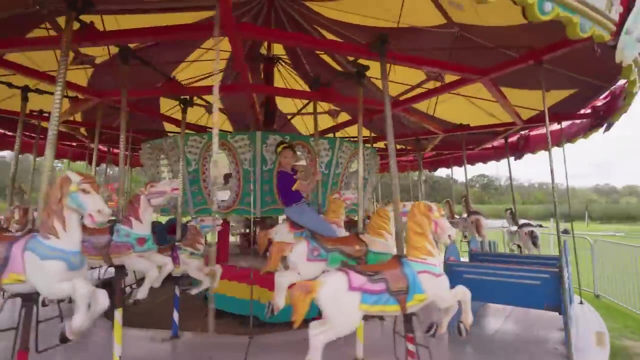 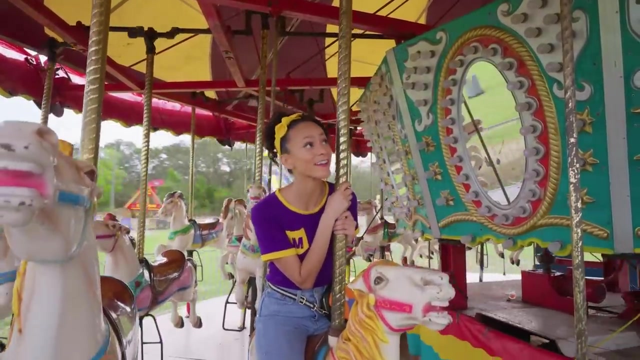 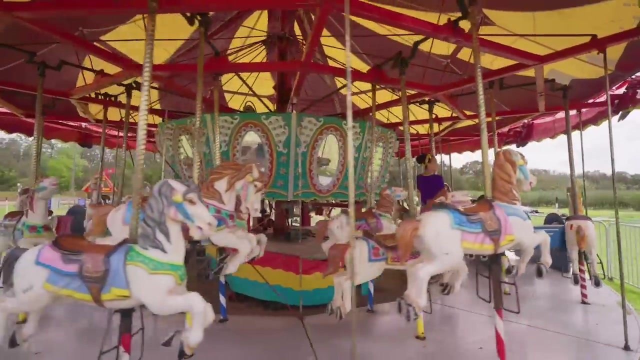 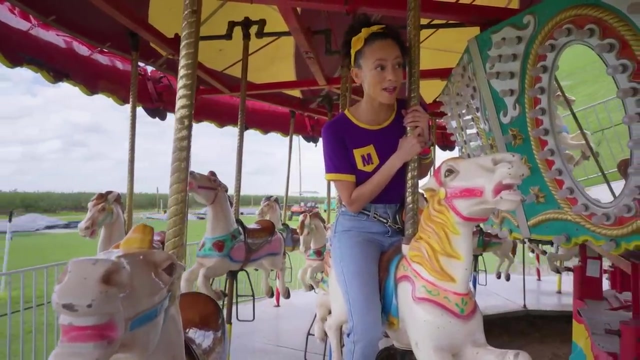 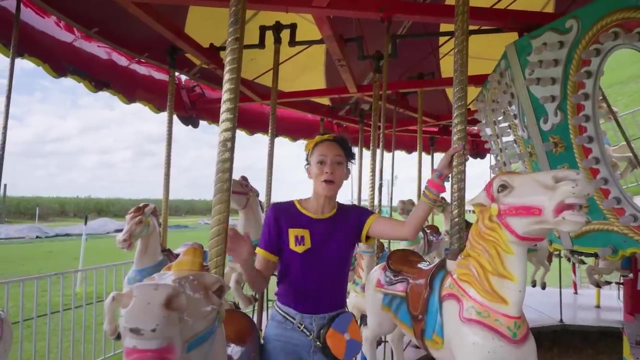 All right, You have to wait until it gets to a complete stop before you get off the horse. That's the second thing to do And we're stopped. That was so fun. Let's see what else we can find here, Wow. 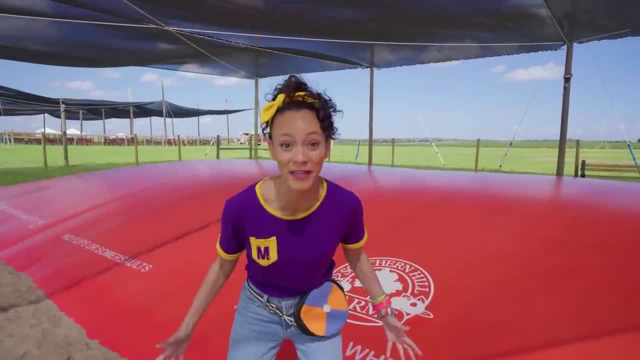 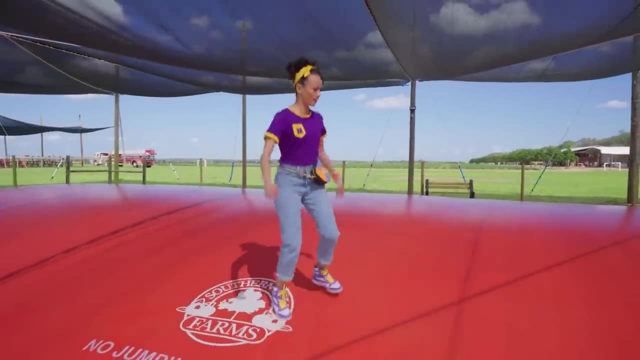 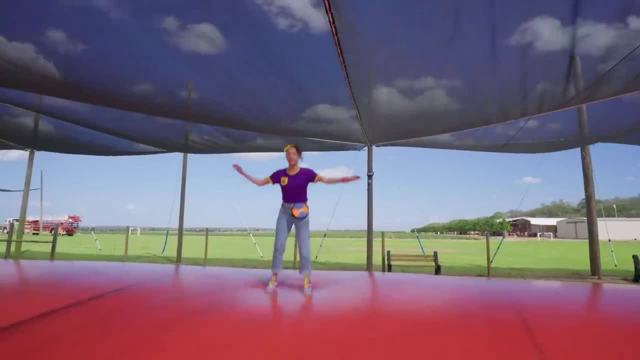 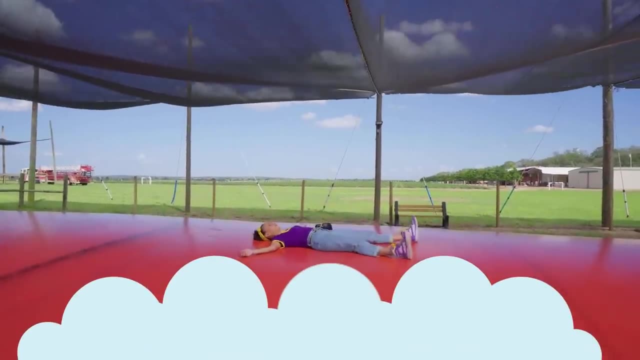 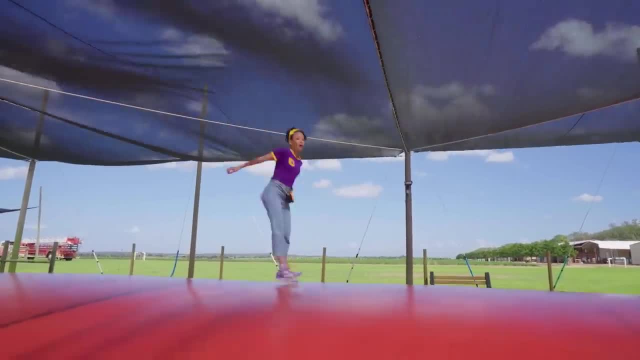 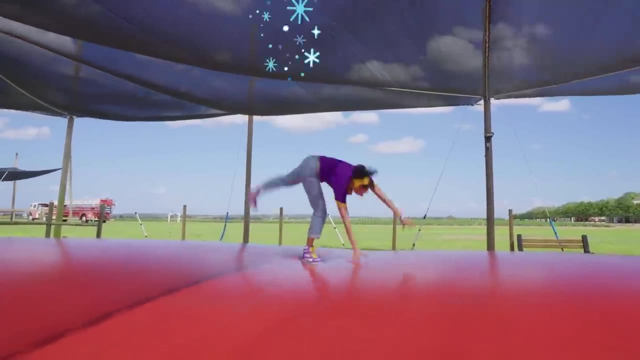 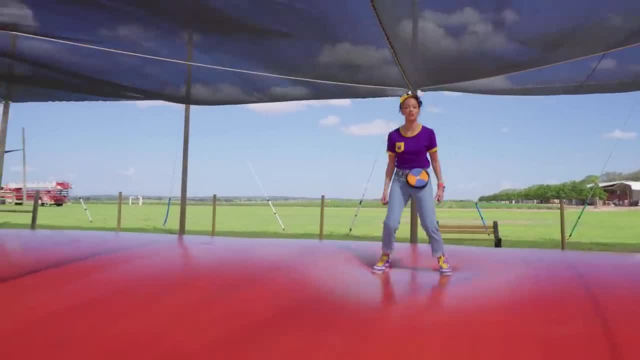 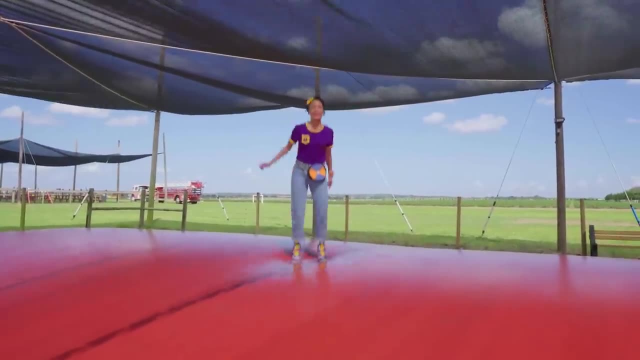 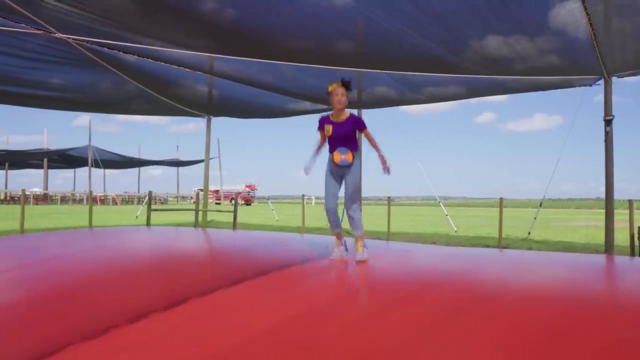 Ready, Woo hoo, Oh, I can also do a round off. Whoa, Hey, You can jump with me. Whoa, Whoa with me. What's one of your favorite jumps? You could do this. Woohoo, You could do it. 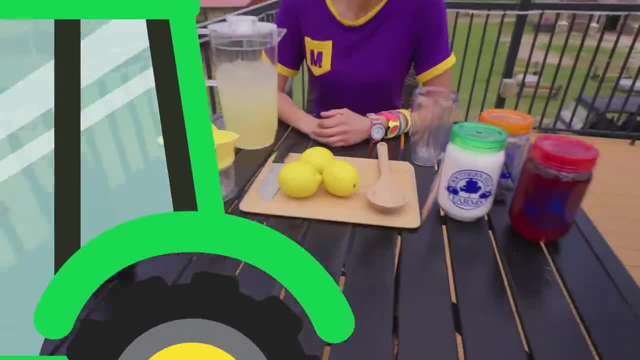 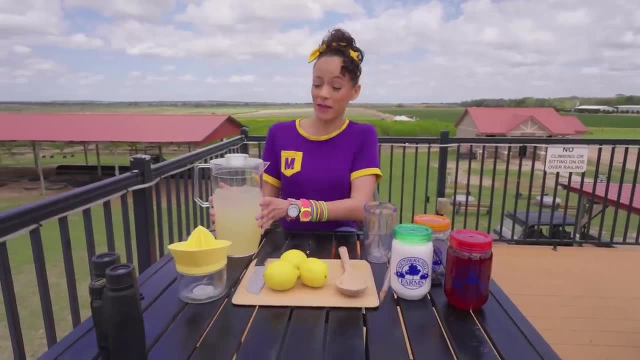 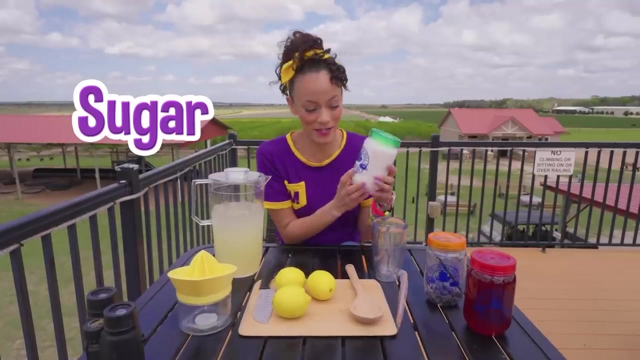 on the other side. Woohoo, I'm so excited to make blueberry lemonade. I already made a lot of lemonade right here. To make lemonade, you need lemons and you need sugar to make it sweet, because lemons are pretty sour And you need some water, But I think we need one. 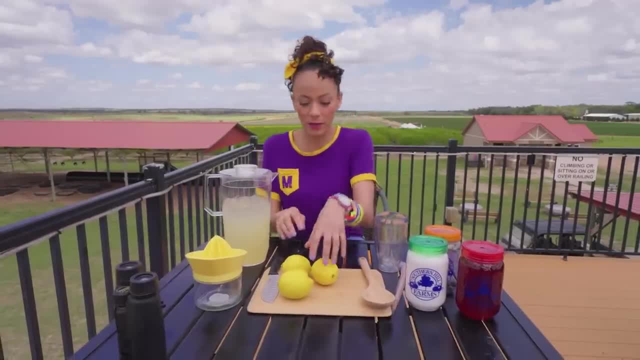 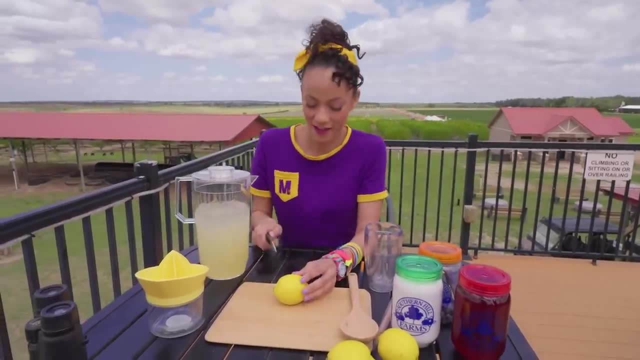 more lemon to go into this lemonade. So let me cut one here. I'll show you how you get the juice out. And remember, only grown-ups should be using knives. Okay, cut this in half like that, And this is a juicer. 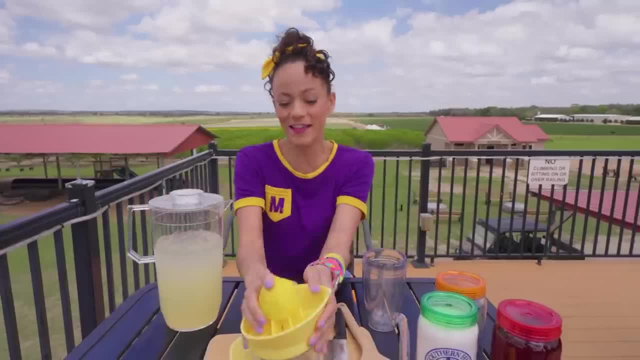 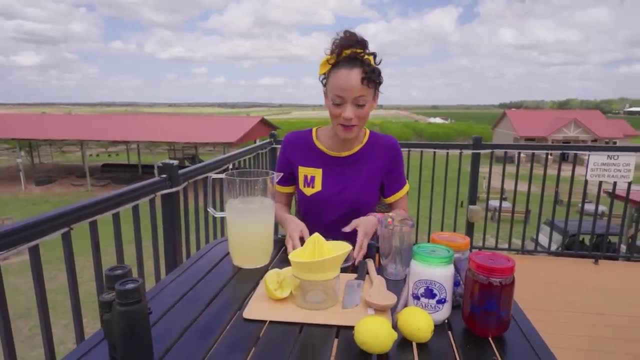 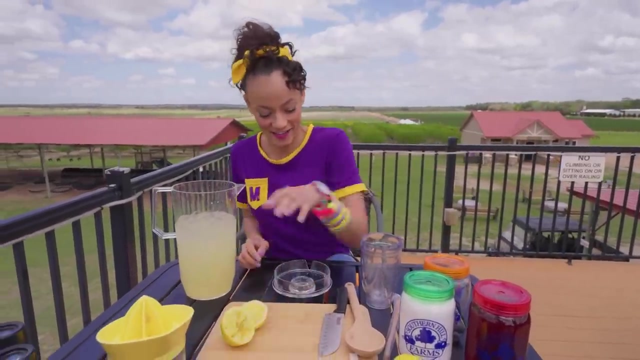 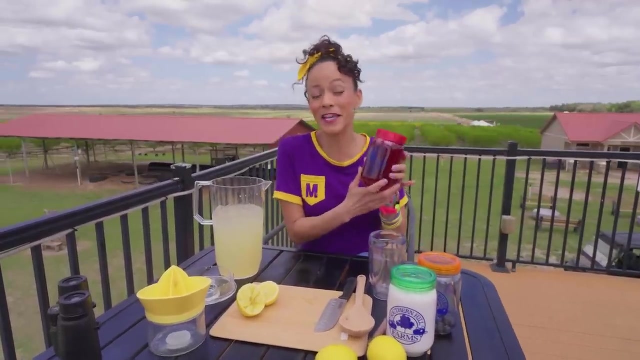 So I'm gonna add that to the pitcher that I already made before Yum. Okay, And my favorite part: we have some juice from the blueberries that you helped me pick earlier. We washed the blueberries and we juiced them. And now I'm gonna put them into the birch- You can do that too. I like these. And then, Okay, And then let's add the fruit. So I'm gonna put a little bit of water in the pitcher. 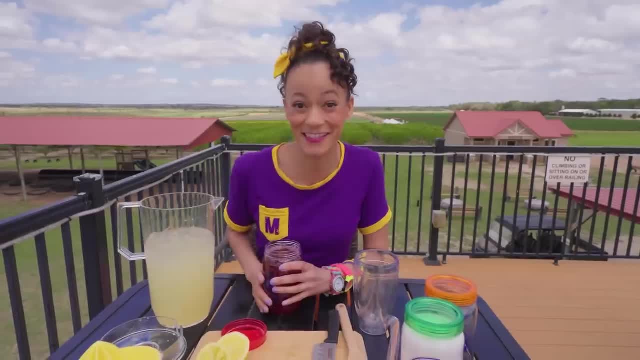 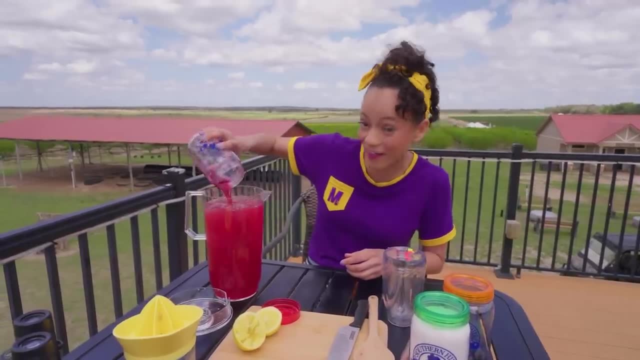 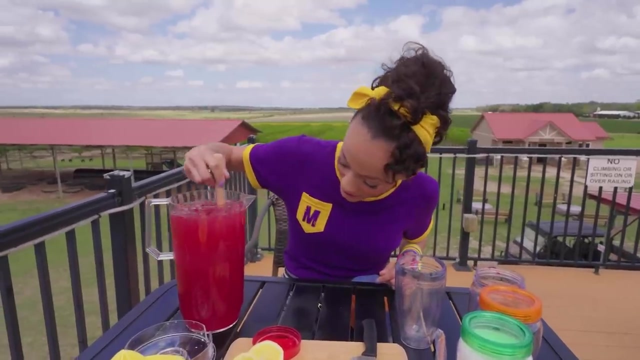 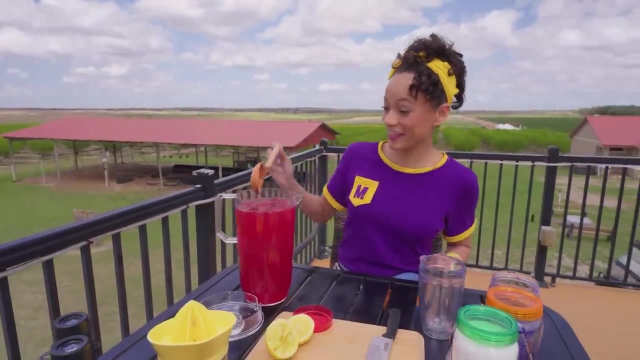 I have some yummy blueberry juice to add to this lemonade. All right, whoa, isn't that such a pretty color? All right, now we'll take a spoon and stir it up. Mm smells sweet and fruity. Hey, I think that's pretty good. 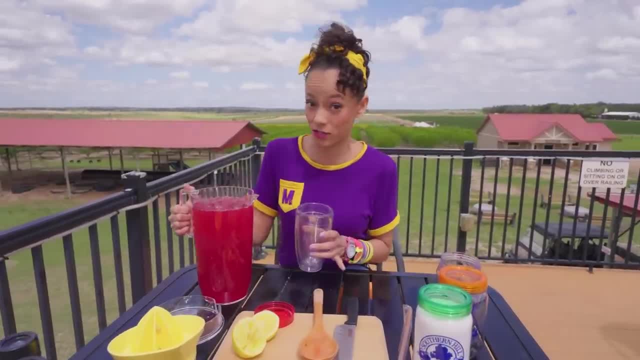 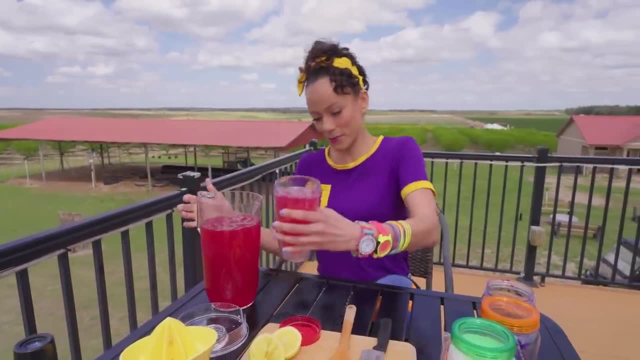 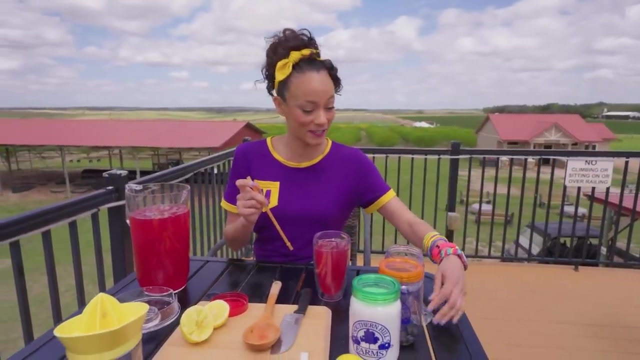 And I have a cup here so I can taste it. I have to make sure it tastes good. All right, whoops, And oh, I should add some extra blueberries to make it really special, Mm. okay, let's see. 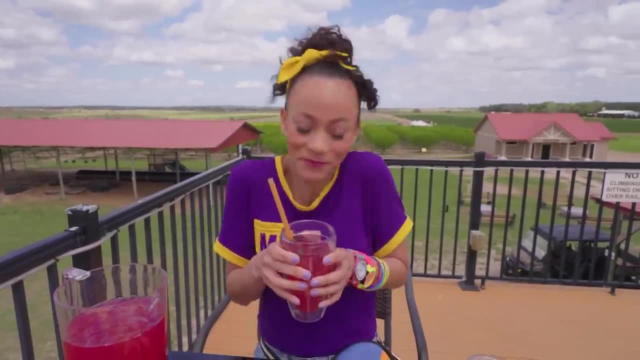 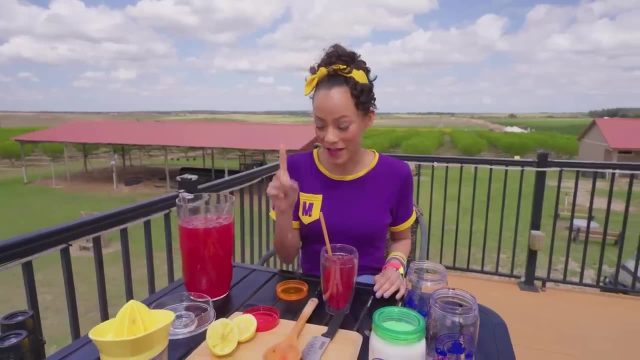 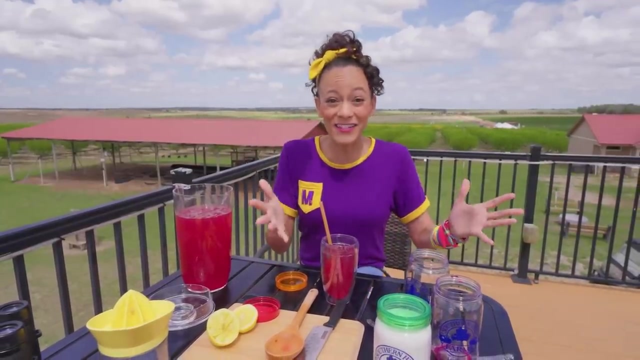 Oh, that's really, really tasty. Oh, I love blueberries so much. Okay, so I picked blueberries, I made blueberry lemonade. What's the other thing that I wanted to do? Find sunflowers, that's right. 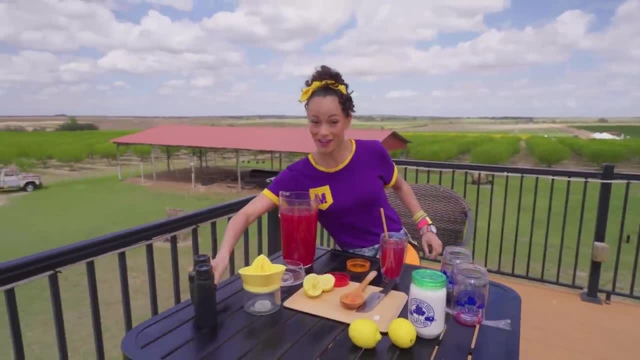 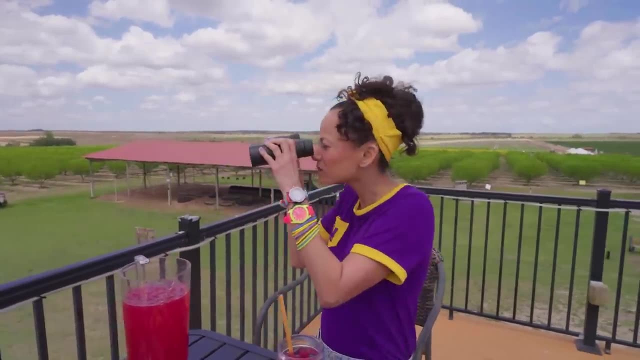 I wonder if there are sunflowers around here. I have these binoculars. They'll help me look a little closer. Let's see Where are the sunflowers. Oh, I see sunflowers down there. Let's get a closer look. 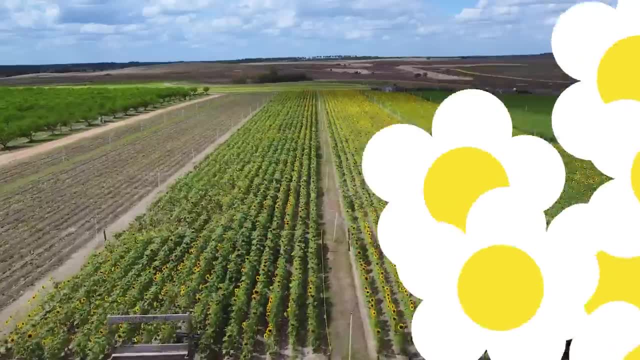 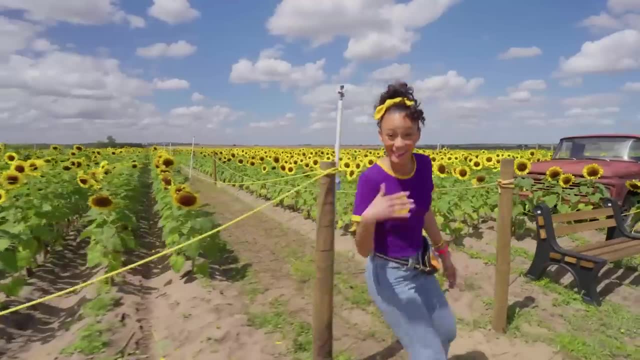 Oh, I see sunflowers down there, Let's get a closer look. Oh, I see sunflowers down there, Let's get a closer look. Come on, I found the sunflowers. Oh, there's a really big one down here. 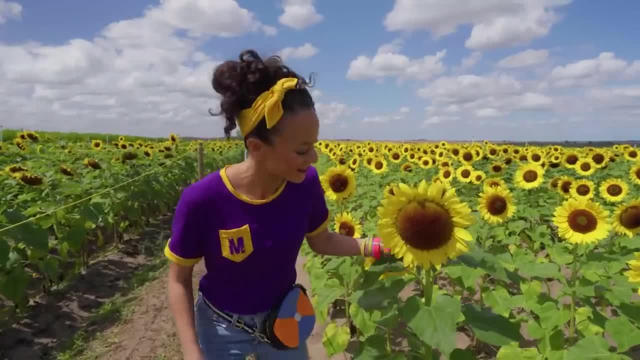 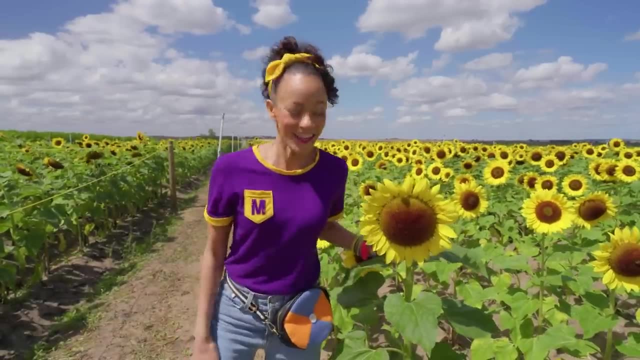 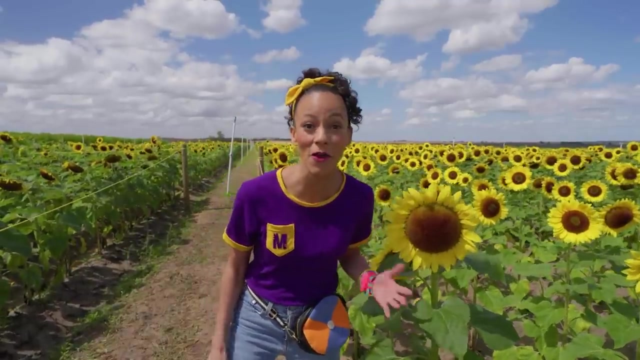 Wow, it's so pretty. See, the inside looks like the sun and the petals all around look like sun rays. Isn't that cool? Like a big, beautiful sunshine. And speaking of sunshine, did you know that sunflowers are attracted to the sun? 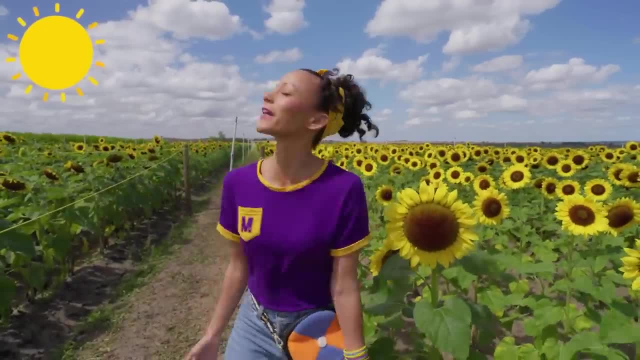 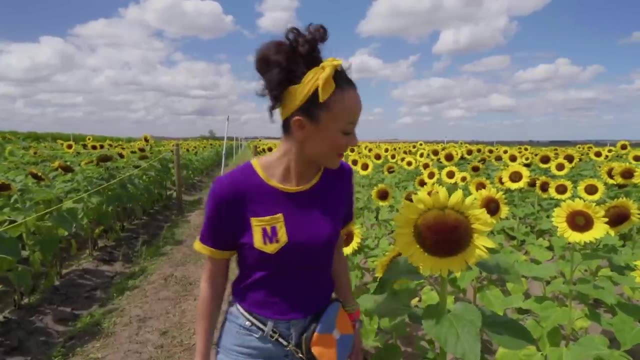 So if the sun is shining over here, a sunflower will look like this, And if the sun is shining over there, the sunflower will look like this. That's so cool. Oh, they're so beautiful. So I think we did everything that we planned. 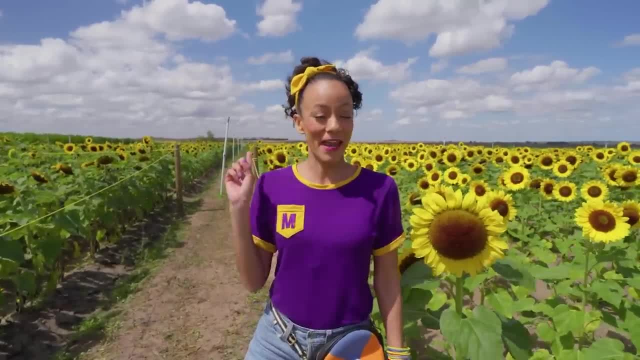 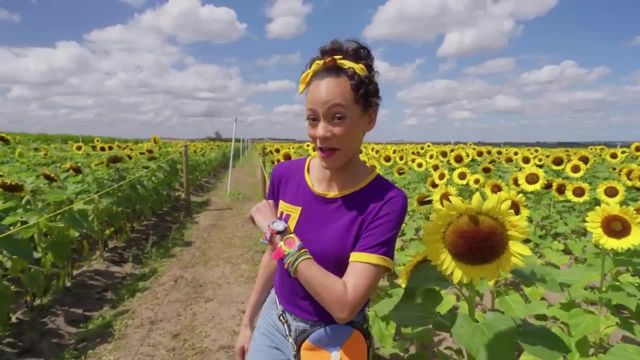 Let's see. We picked blueberries, We made blueberry lemonade, We made blueberry lemonade And we found sunflowers. We did it. Thank you for your help. Well, this is the end of this video, But if you want to see more of my videos, 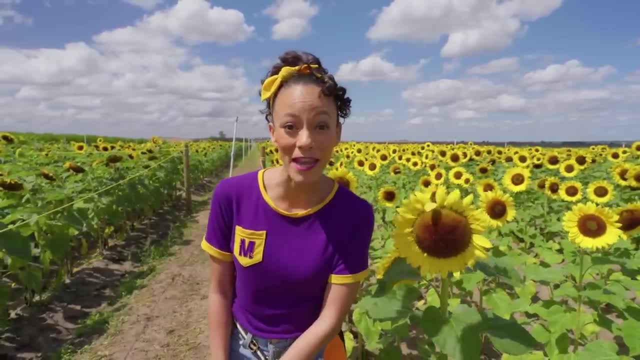 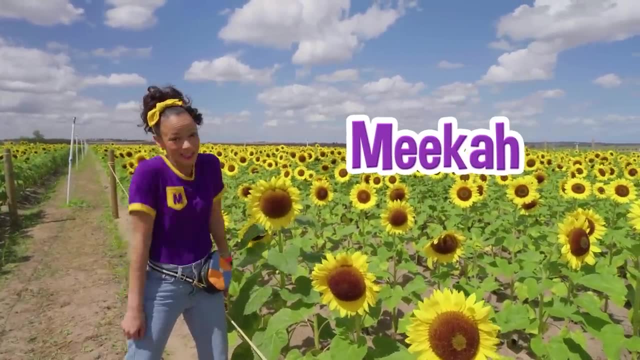 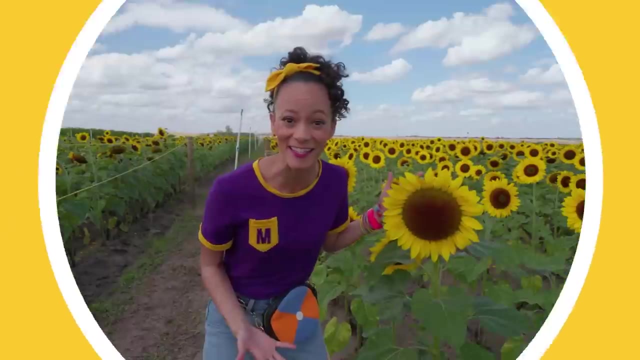 all you have to do is search for my name. Will you spell my name with me? Cool, M-E-E-K-A-H- Mika. Well, we'll see you next time. Bye, Come on, everyone, Let's make learning fun.